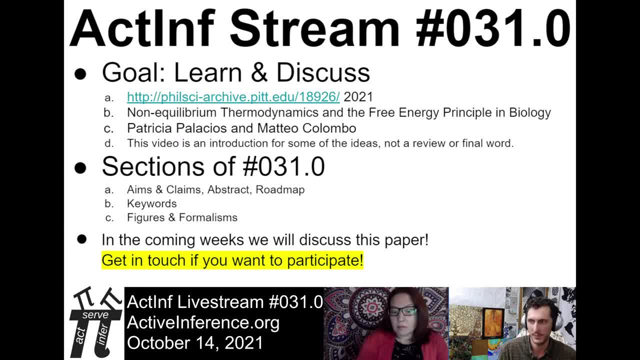 It's not a review or a judgment or a final word. In 31.0, we're going to start by looking over some of the key aims and claims and the abstract and the roadmap of the paper to get the big picture. Then talk about some of the keywords. 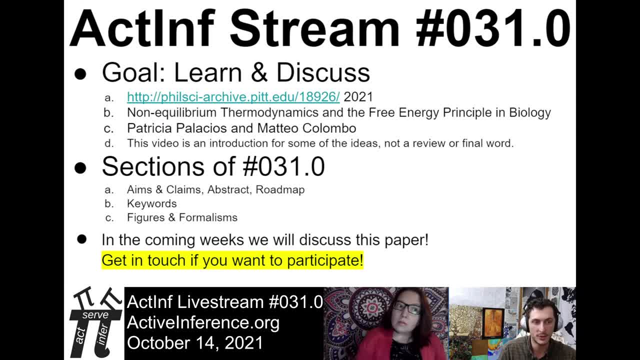 Maybe you're really familiar with some of the keywords, Maybe it's the first time you've thought about some of these topics, And then we'll walk through some of the figures and formalisms and just get set up in the coming weeks to be discussing this paper. 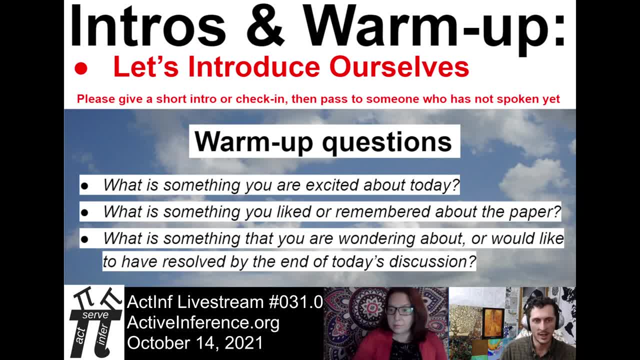 So we'll start with just some introductions and warmups. We'll say hello and then maybe just mention something that we're excited to talk about or learn about or something that we noticed while reading the paper. So I'm Daniel. I'm a researcher in California. 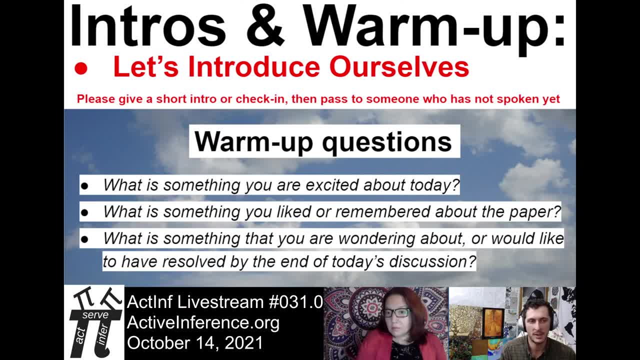 And this is just an exciting paper and topic because it's at the intersection of chemistry and physics, and thermodynamics, but also active inference, And it's a nice starting point for a conversation about what are the precursors and the tenants and the principles of free energy principle and active inference. 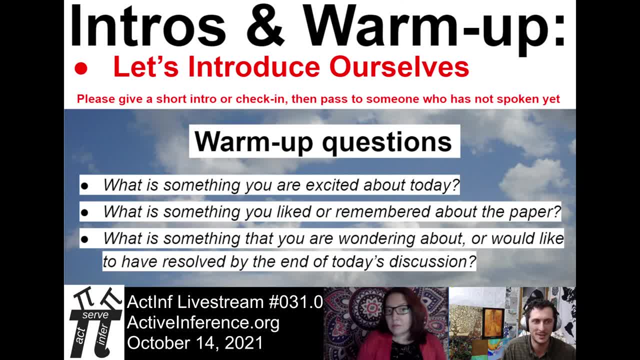 And then what are the consequences and what does that mean for the big picture? Blue, I'm, Blue Knight, I'm an independent research consultant. I'm an independent research consultant in New Mexico And I really was excited to see this paper bring up some of the points that I've brought up, as I've been reading more about active inference, specifically with respect to ergodicity and what that means, the potential implications for that. 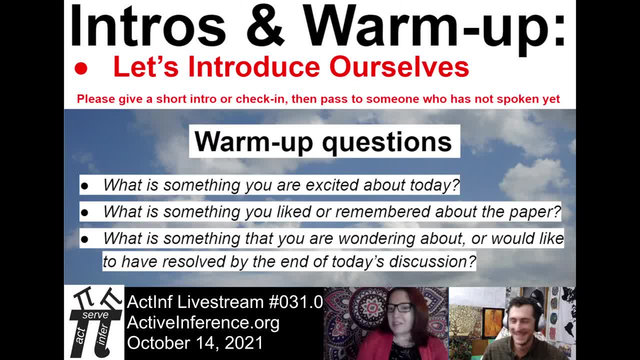 And also just other minor topics, but things I've mentioned in the past. It's cool sometimes to see how the threads of our previous discussions and things that a participant might have brought up Like, hey, this isn't making sense And it's like, don't worry. 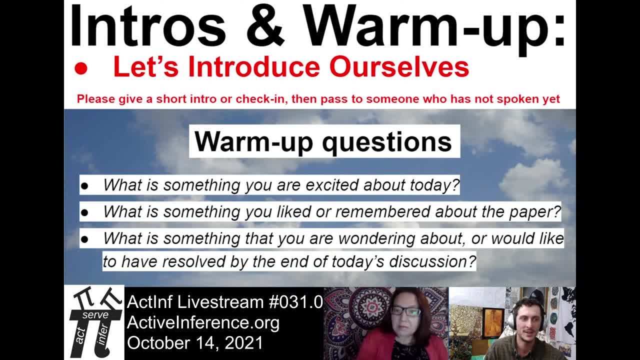 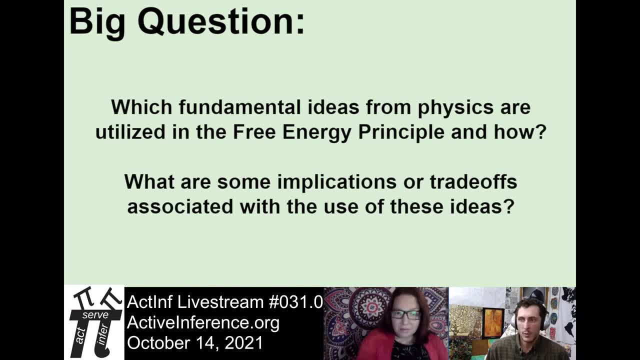 It's not just you. These are open research questions And so we're seeing that and we'll be enacting it in the coming weeks. Some of the big questions in the paper kind of framed in non-technical or in not the author's words. 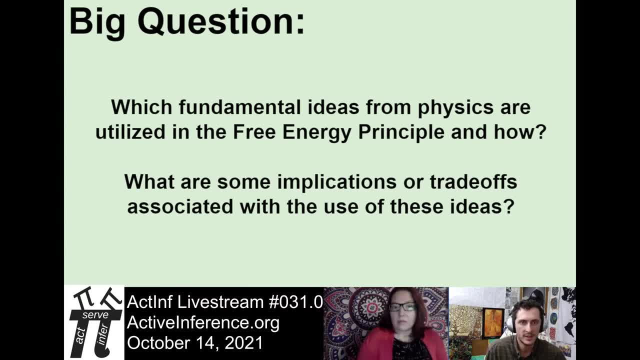 It's really asking what fundamental ideas from physics are utilized in the free energy principle and how are they utilized. Why are they utilized? And then what are some implications or tradeoffs associated with the use of these ideas, Either the ways that they have been used, 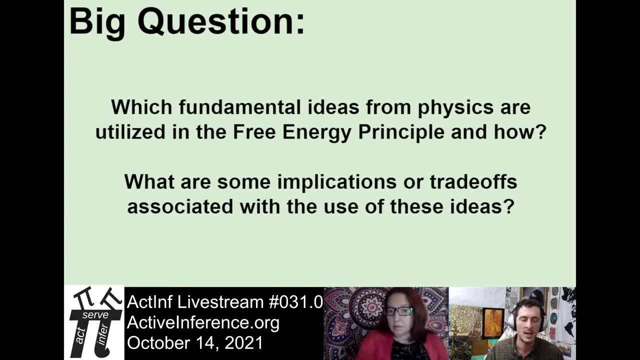 What are the pros and cons, or what are the implications, And what about the ways that they could be used? So, in the spirit of positive contributions to the literature, how are we taking ideas from physics and other fields, bringing it together in free energy principle? 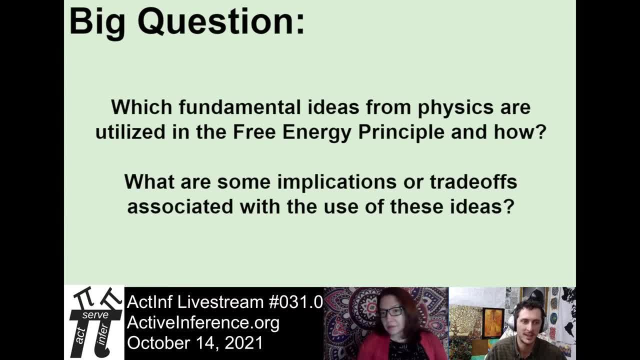 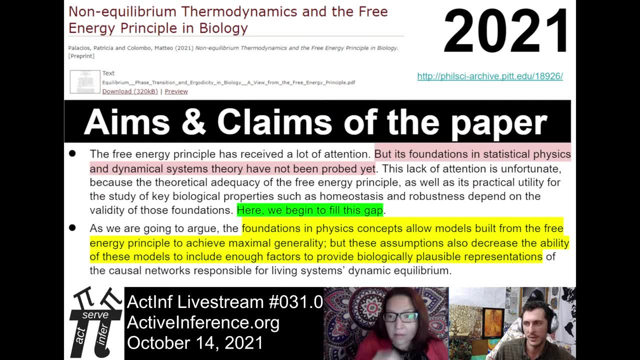 And then, what are the fundamental or just spuriously contemporary tradeoffs? Let's first go to the aims and claims of the authors. So I'll read it, and then, Blue, you can give a thought. Well, the paper is the Non-Equilibrium Thermodynamics and Free Energy Principle in Biology. on the PhilSci Archive at Pitt. 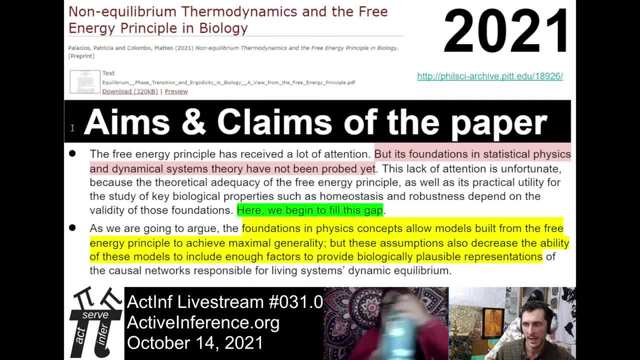 So check out the paper and read it if you want to. And a few of their aims and claims are: The free energy principle has received a lot of attention, but its foundations in statistical physics and dynamical systems theory have not been probed yet. 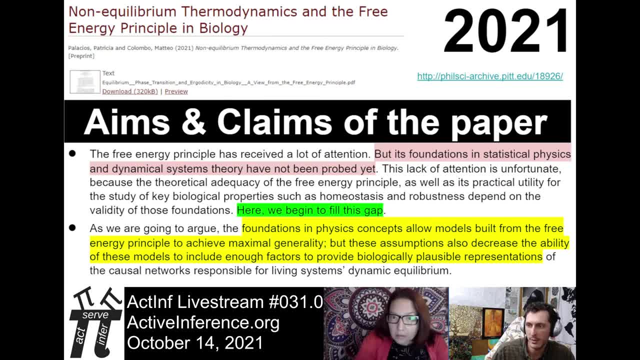 This lack of attention is unfortunate because the theoretical adequacy of the free energy principle, as well as its practical utility for the study of key biological properties such as homeostasis and robustness, depend on the validity of those foundations. Here we begin to fill this gap. 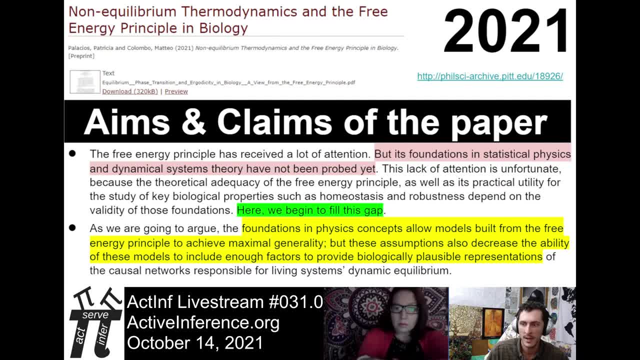 So that's kind of one of their contexts. They're contextualizing claims and their aim And one of their arguments- a claim about their arguments- is that, As we are going to argue, the foundations in physics concepts allow models built from the free energy principle to achieve maximum generality. 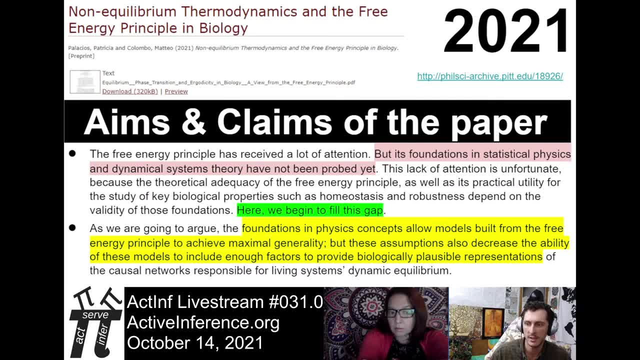 But these assumptions also decrease the ability of these models to include enough factors to provide biologically plausible representations of the causal networks responsible for living systems' dynamic equilibrium. Any thoughts on the aims Or we can continue? Wait, I can't hear you. 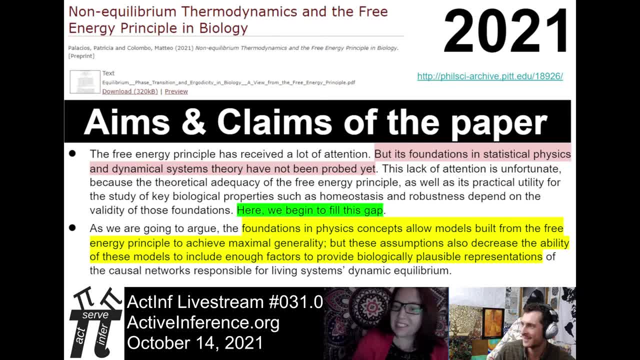 I think that the aims are good. Sorry, I just realized I was muted. I think that the these are good aims. I think that one of the fundamental claims is that, in order to make the FEP more generalized- generalizable- it's not as specific to biology as it could be. 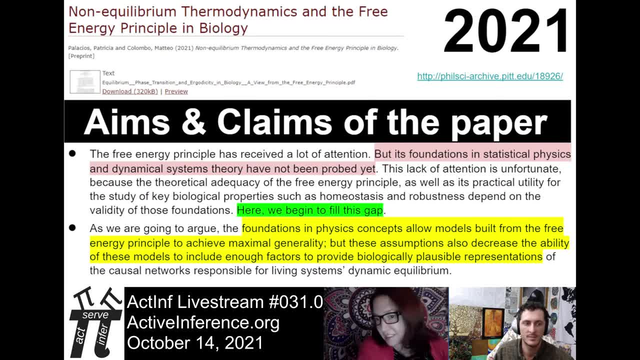 I think that that that was like the key to that. I think that that that was the key to that. So we can continue. So was like the key trade-off, maybe, yes, between specificity and utility and generalizability. so one mindset is that as we generalize, we're going to be explaining more systems, different. 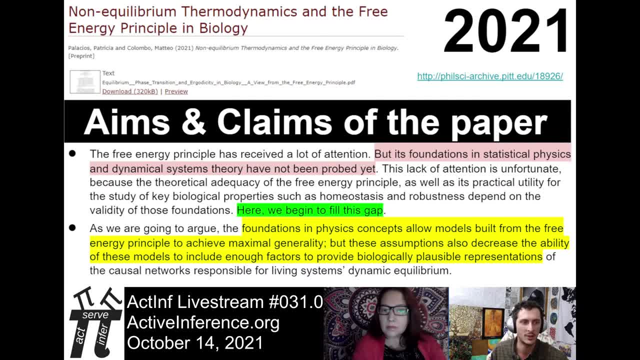 systems, explaining them better, doing more, and it's just all up up, up with generalization. another contrasting opinion is that as we generalize, we, out of necessity, abstract or average out over particulars, and so we might actually lose utility or potentially and even disastrously lose the specifics of the system that we're talking about. so, all of a sudden, we 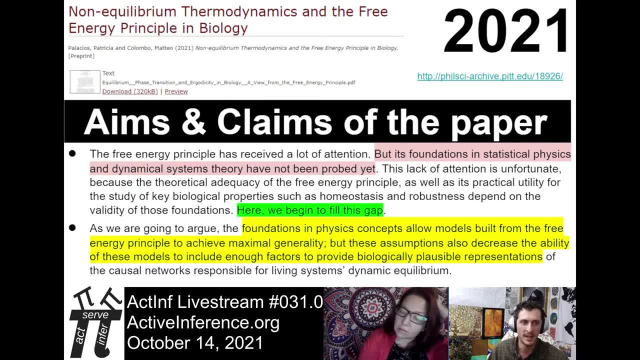 have this free-floating generalization or abstraction that maybe initially was inspired by wanting to explain some sort of key biological property like homeostasis and robustness, in the author's view, but then we end up sort of throwing out the kernel or the the essence of what we wanted to explain because we generalized too much. so we'll be exploring that. 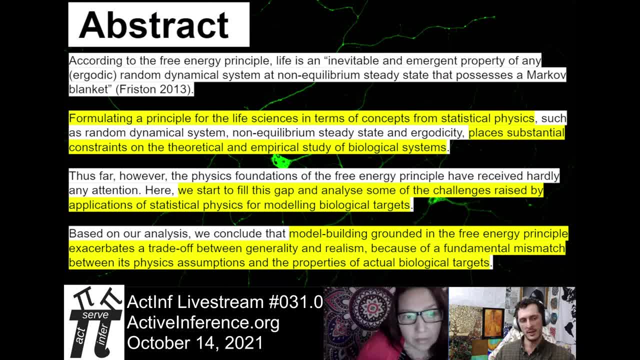 okay, do you want to read the abstract? sure? according to the free energy principle, life is an inevitable and emergent property of any ergodic, random dynamical system at non-equilibrium steady state that possesses a markov blanket. first in 2013, formulating a 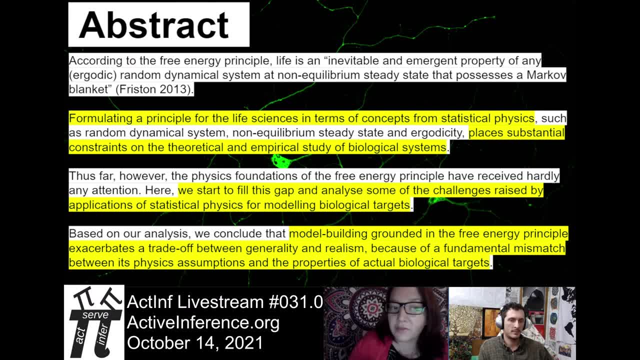 principle for the life sciences in terms of concepts and principles of life sciences from statistical physics, such as random dynamical system, non-equilibrium, steady state and ergodicity, places substantial constraints on the theoretical and empirical study of biological systems. thus far, however, the physics foundations of the free energy principle have received hardly any. 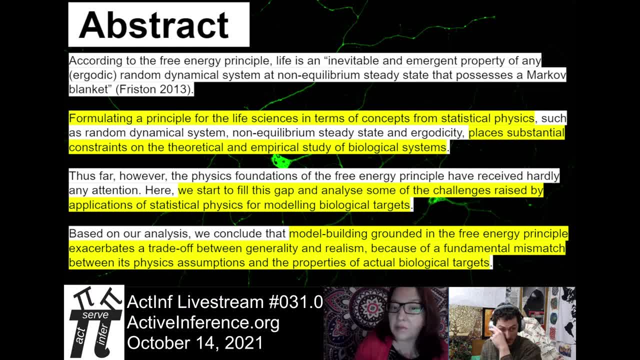 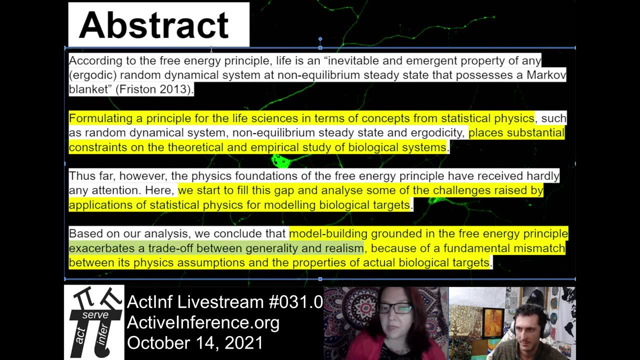 attention. here we start to fill this gap and analyze some of the challenges raised by applications of statistical physics for modeling biological targets. based on our analysis, we conclude that model building grounded in the free energy principle is a very important part of the theory, and the free energy principle exacerbates a trade-off between generality and realism. 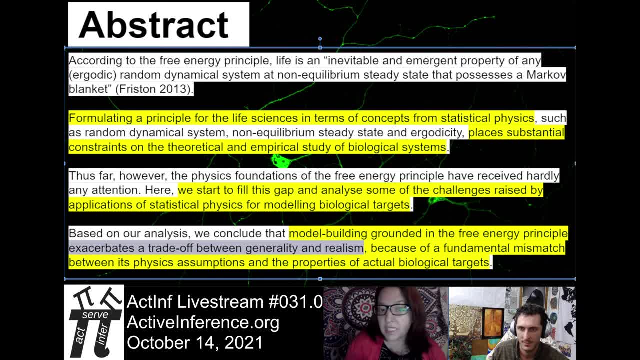 because of a fundamental mismatch between its physics assumptions and the properties of actual biological targets. cool, and there's a lot to say. that's just the opening salvo from the authors. how do they make good on this abstract? we can look at the roadmap. there's not too many sections. 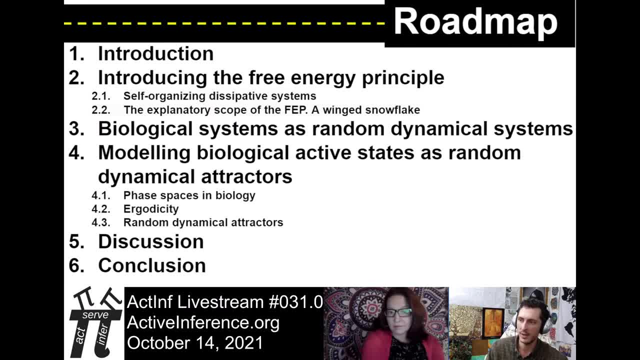 in this paper, but there's a lot of uh meat within. there's a general introduction and then a specific introduction to the free energy principle, which is described in the context of self-organizing dissipative systems, and then there's a little discussion on the explanatory scope of the fep and the introduction of the 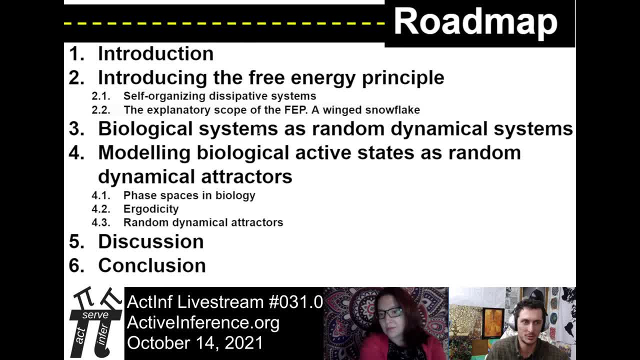 winged snowflake, thought experiment or idea, which we'll return to soon. section three talks about biological systems as random dynamical systems and the introduction of the winged snowflake, which isn't something that fep invented, it's not something that actin invented. this is a broader 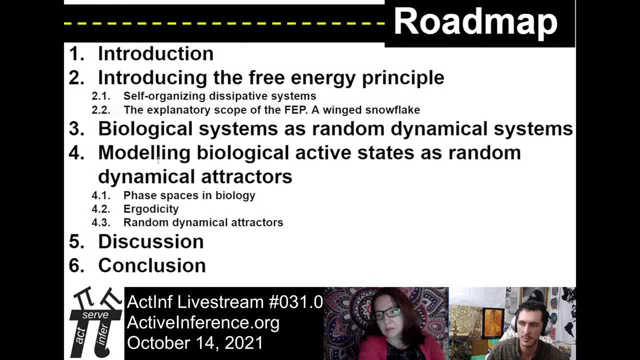 question about how to model biological systems and dynamical systems. section four models biological active states as random dynamical attractors and talks about three big physics ideas that if we take section three, you know, if we want to be modeling biological systems as dynamical systems, then we're using this physics ontology and what other key terms. 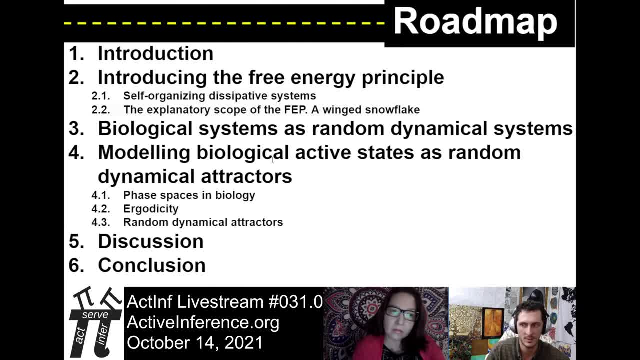 are relevant physics for discussing random dynamical systems, And we will go through them. They are the idea of phase spaces in biology, ergodicity and random dynamical attractors. There's then a discussion and a short conclusion. So that's kind of the overall roadmap. That's where we're going to go. 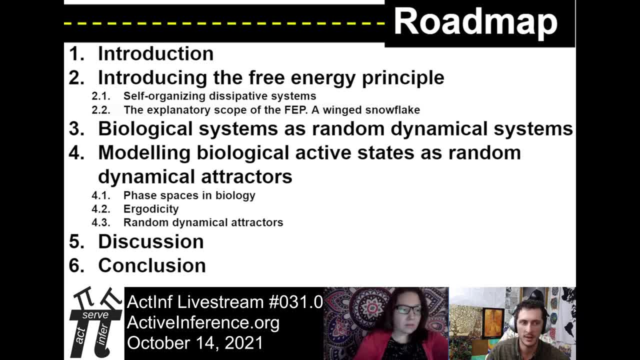 We're going to be exploring that trade-off, or the implications of the introduction of physics fundamentals into the generalization of biological systems and maybe even non-living systems as well, And just how's it all going to come together and how does it influence how we research going? 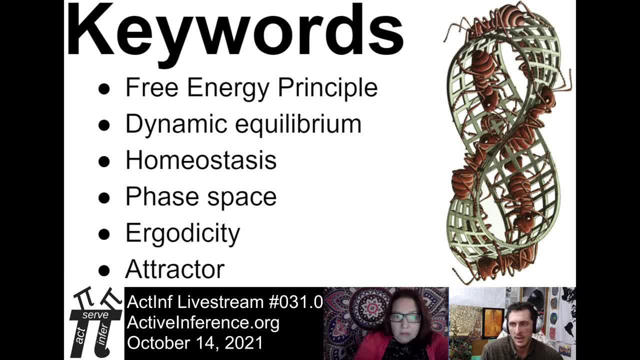 forward. The keywords are FEP, free energy principle, dynamic equilibrium, homeostasis, phase space, ergodicity and attractor. And we can ask where's active inference? Not that it has to be a keyword for everything, But as we discuss, let's keep in mind what are the differences between FEP and ACT-INF? 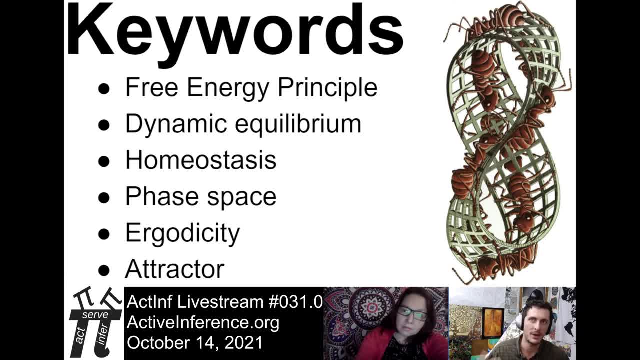 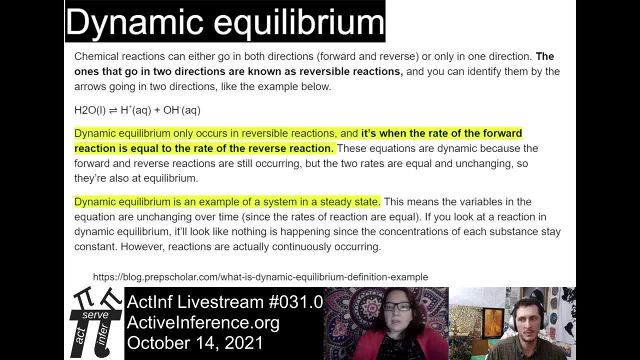 And what are the implications of these claims about FEP for ACT-INF? All right, How about the first keyword, dynamic equilibrium Blue? So interestingly, like you said that you like how this paper brings together physics and chemistry and biology, And I thought that chemistry was kind of blatantly omitted. 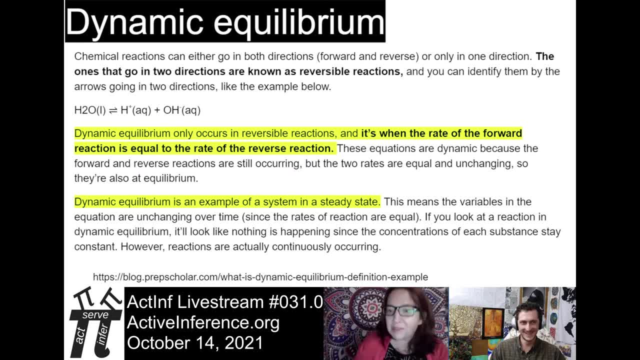 And in my heart I'm a chemist- Like if I hadn't studied neuro I would have really like gone into OCHEM. I just thought that like working in the lab was a little scary, like too much ether and too like whoa. when I came out. 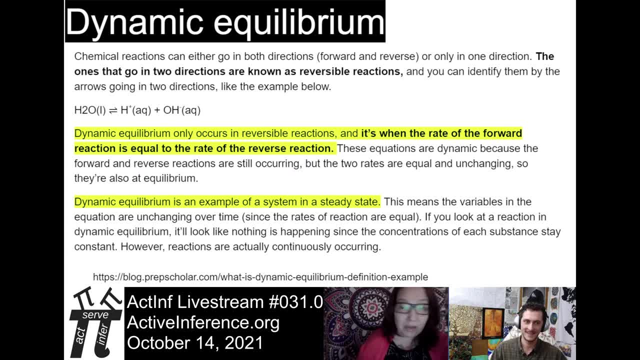 So, really, when I look up dynamic equilibrium or the context that I'm familiar with, dynamic equilibrium is in chemistry And so a dynamic equilibrium occurs when you have a reversible chemical reaction. So it's not that the reaction is over, right? Like here's an example of water ionizing into hydroxide and protons, right? 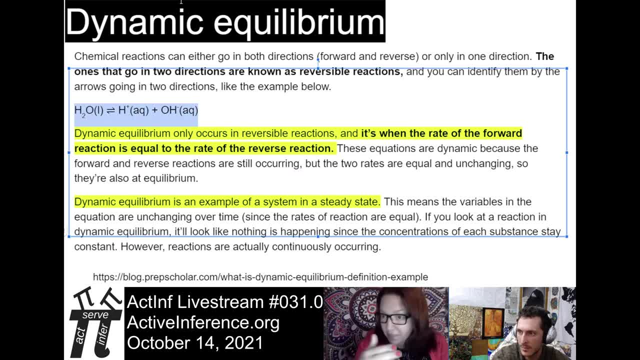 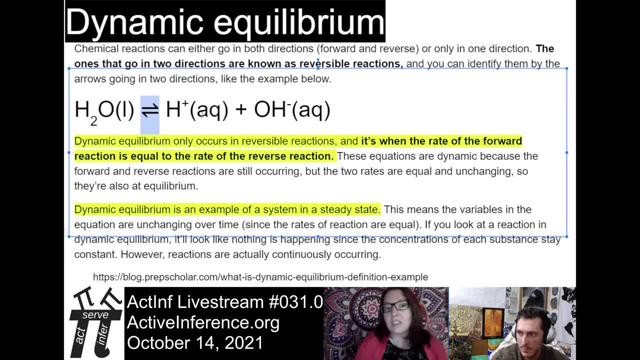 And so it's not that when you have the equilibrium that the reaction is still occurring. It's just occurring at equal rates in the forward and reverse directions. So this is dynamic equilibrium and it only happens in a reversible chemical reaction. So there's no other way. 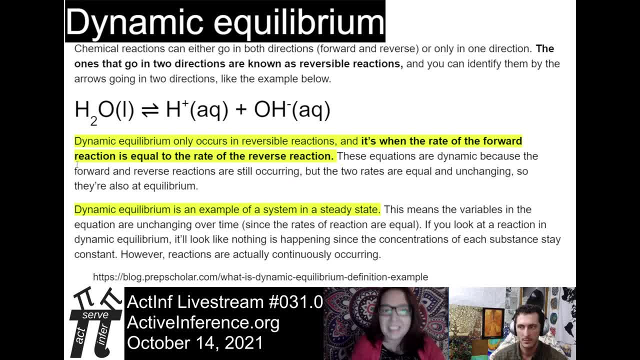 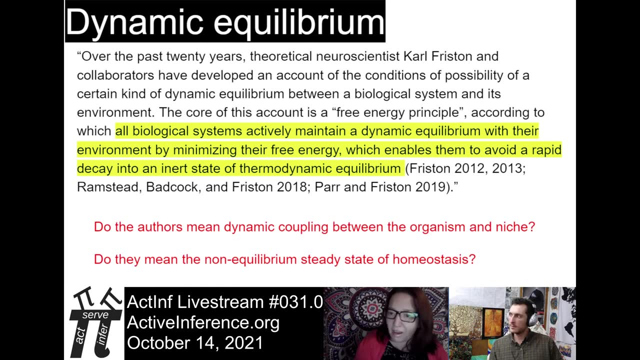 That I know of that, that dynamic equilibrium happens. It is an example of a system, particularly a chemical system, at a steady state, And so I looked through the paper. I don't know if you want to flip to the next slide. I looked to the paper and I looked like: well, how are the authors using dynamic equilibrium? 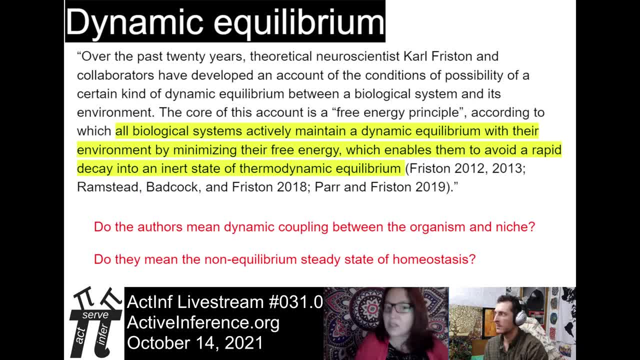 And I found this phrase, which I'll say here: the core of this account is a free energy principle according to which all biological systems actively maintain a dynamic equilibrium with their environment by minimizing their free energy, which enables them to avoid a rapid decay into an inert state of thermodynamic equilibrium. 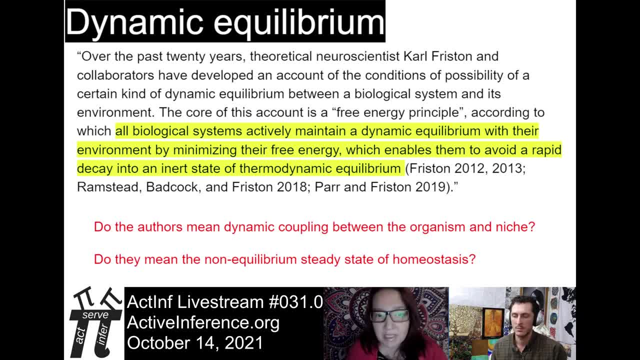 And so then there's some citations: Friston and the Ramstad 2018 paper, and Par and Friston in 2019.. And so even I looked back through these papers and looked for dynamic equilibrium, and it's not there in the references that I was able to find. 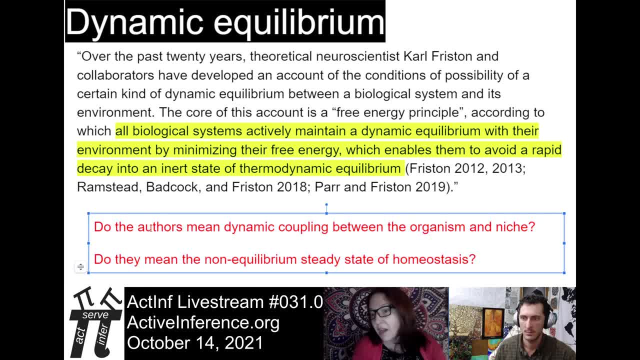 And so I was curious what the authors meant. What was meant by dynamic equilibrium in a living system? I mean, as far as I know, like maybe they meant dynamic coupling between the organism, organism and the niche, or maybe they mean the non equilibrium. 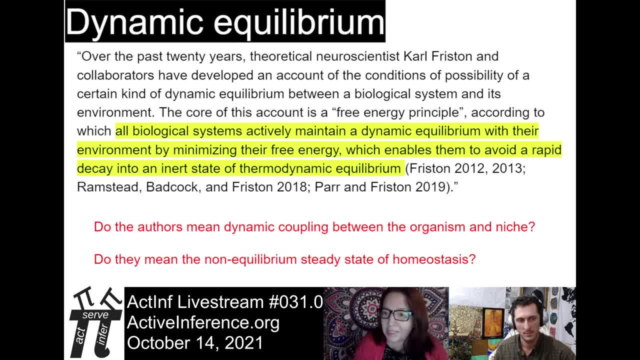 steady state of homeostasis, which is not a dynamic equilibrium, It's a non equilibrium. So I just found this, this phrasing, kind of curious and I'm assuming, just based on context, that they're referring to homeostasis. But homeostasis includes plenty of irreversible reactions. 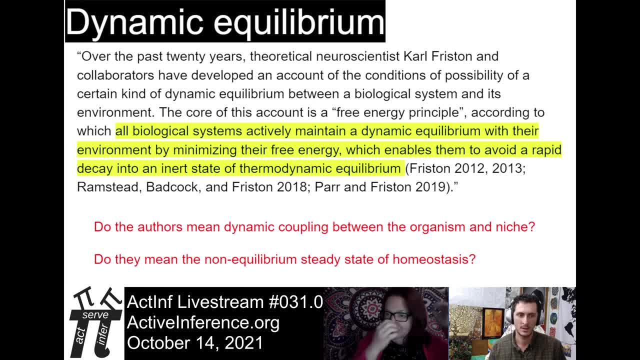 Irreversible chemical reactions, And so that's kind of why this was a little bit sounding. It makes sense Like, if we think about, instead of the water ionizing and the H plus and the minus coming back together and the overall values on both sides are staying the same. 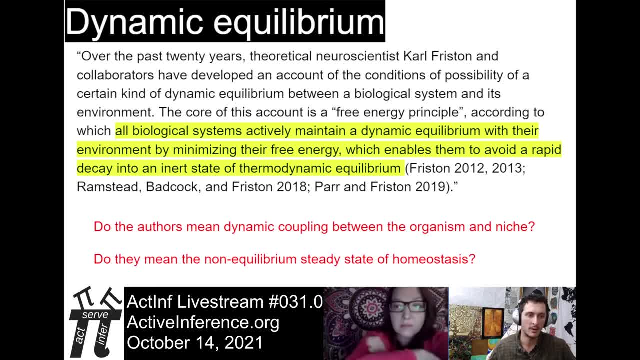 So let's think in the biological case, like, moment to moment, our, our mass is staying the same. Let's just say, or some people maintain the same mass for 30 years. but underlying that stability Is actually many, many, you know, synthesis of fatty acids and the breakdown of fatty acids. 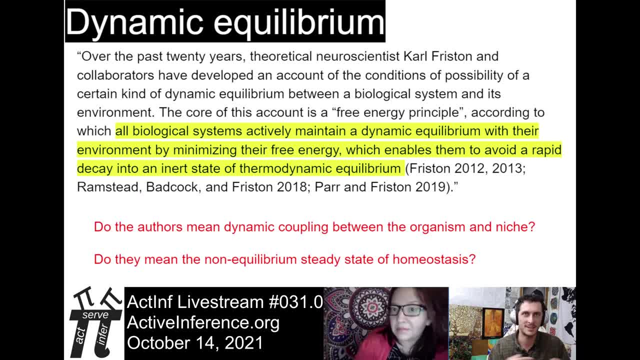 And so it's like, okay, I get it that they're both going both sides at the same rate, So there's a stable point. but then also it's constituting its own irreversible thermodynamic reactions sometimes, And so it's a good question. 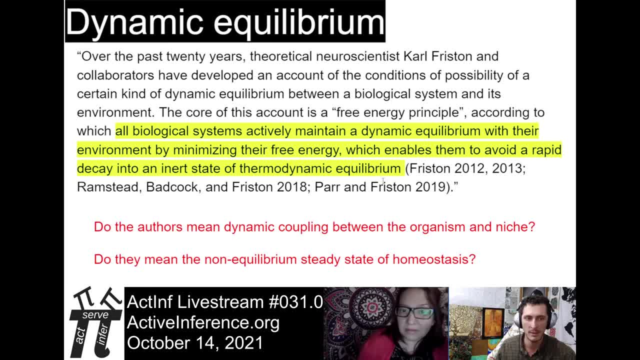 Do Friston at all use the term dynamic equilibrium? And are we talking about dynamic couplings, Yeah, Which might be at steady States, or are we talking about the non-equilibrium steady state of homeostasis? Okay, Brings us to homeostasis. 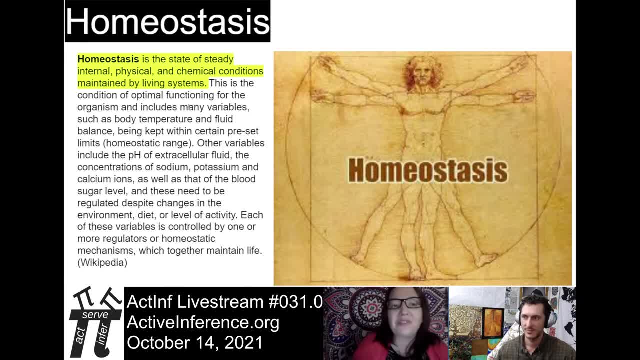 Sure. So homeostasis is the steady state of internal, internal physical and chemical conditions that are maintained by living systems, And there's a lot of variables that are can be included in here. Mass, I think, Actually Changes at night. like the you, the carbon that you exhale, like you actually weigh less in the morning from like sleeping all night and like emitting carbon. 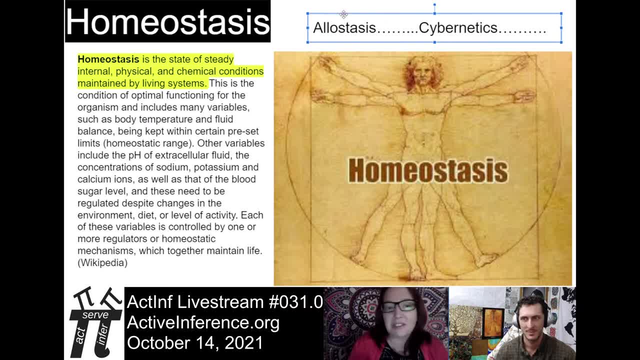 I heard um. I don't know if that's really true, but I guess it depends on what scale you're measuring. Um. but but I think that pH has to be the same or within like a pretty defined range: Um, osmolarity, sodium, potassium and calcium ions, blood sugar, um body temperature is a huge one. 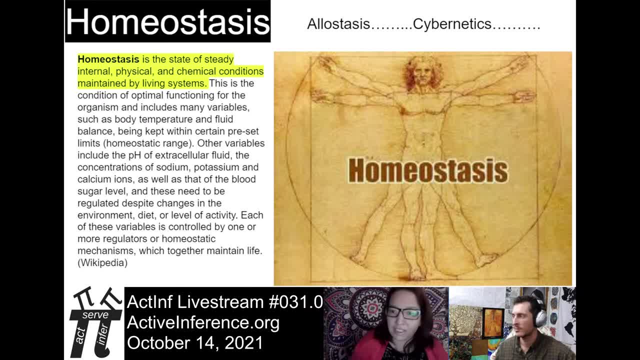 So, and and we act. we do things throughout the day like eat and drink and use The restroom and put on jackets to maintain, to help with our, you know, homeostatic conditions. um, internally, Well, unless we're eating at night, we're losing water and some other molecules. 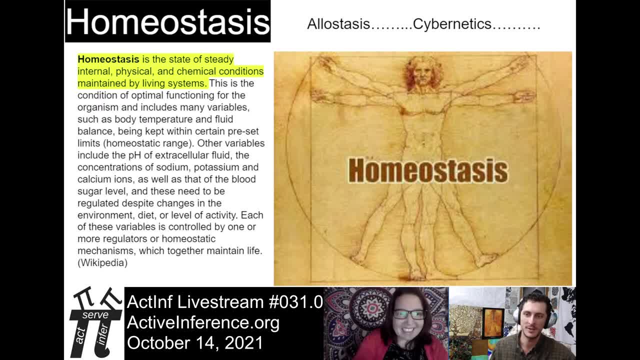 So definitely we're lighter in the morning. And then one discussion that we've had in few different streams is: when do we think of homeostasis as reducing uncertainty from a set point like sort of a desired temperature, And then we want to just reduce? 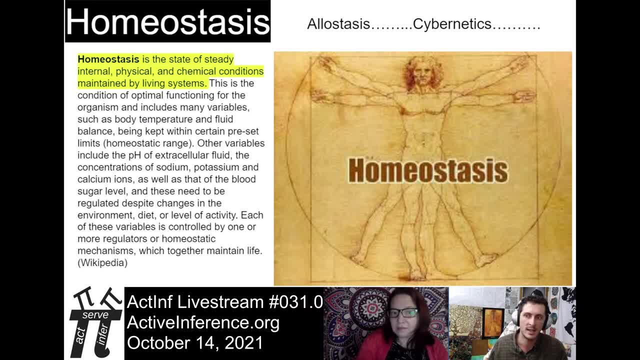 Okay, Reduce our discrepancy versus when do we see allostasis or almost like anticipatory processes by which biological systems actually take excursions, qualified excursions, from set points, And how do we think about that within the broader history of cybernetics? 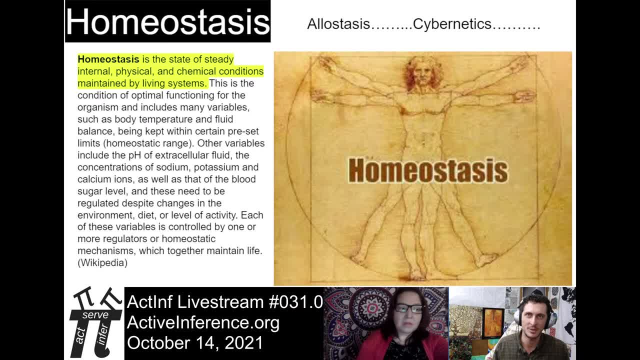 And it's been said that, um, cybernetics had some challenges with dealing with post homeostasis. So it's easy enough to see how a cybernetic system Seeks A set point, But then, once you start thinking well, what is the process by which that set point is itself moved around all of a sudden? that challenged a lot of historical cybernetics frameworks. 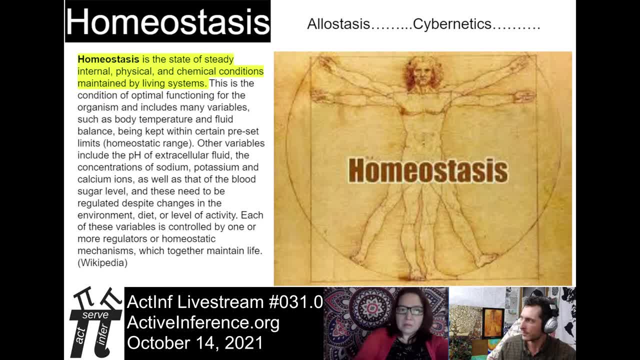 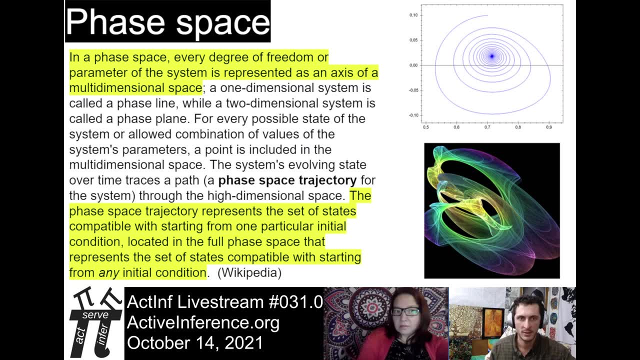 So that's definitely what we're exploring with act Inf. let's take another dip into a physics or a mathematical idea of a face space. So I'll read the yellow parts. or you want to go for it? I'll read the yellow parts. 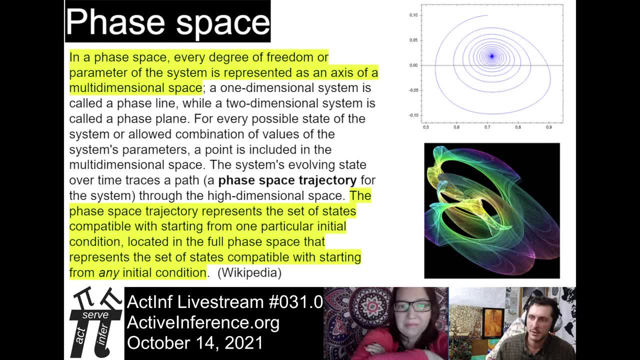 And then you give any description. So In a phase space, every degree of freedom or parameter of the system is represented as an axis of a multidimensional space. So, like every point on this spiral has two variables that describe it. It's like it's value on the X and value on the Y. 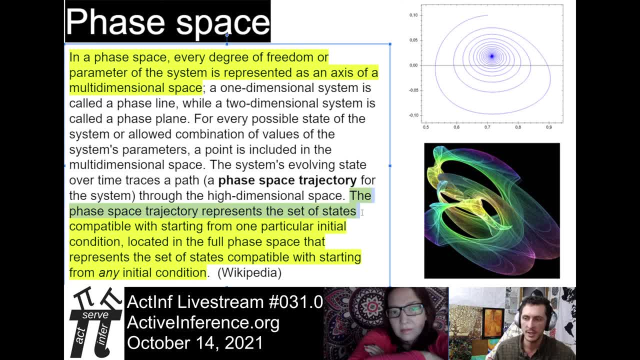 And then the phase space trajectory represents the set of states compatible with starting from one particular initial condition located in the full space space. that represents the set of states compatible with starting from any initial condition. Mm-hmm. So just a quick comment or thought on that. 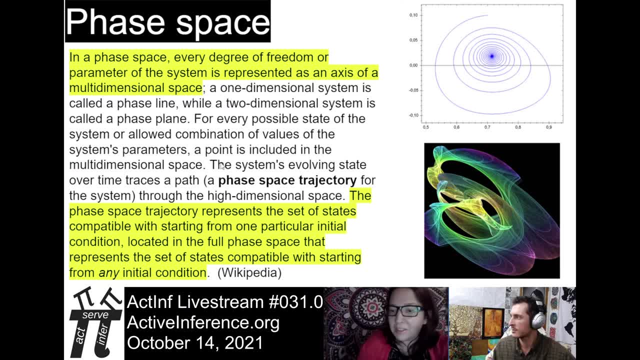 So even just in the maintenance of homeostasis, like where your- you know, osmolarity is the same and your blood glucose is the same, or just intercellular glucose or ATP levels, or you know, if you just want to look at at just maintaining homeostasis, not even including, like, the potential possible actions that I could take in, like moving in a three dimensional environment or anything like that, but but it it becomes very quickly an expansion of homeostasis into a multidimensional environment. 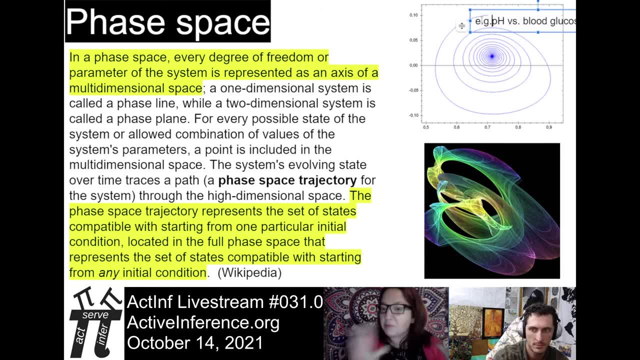 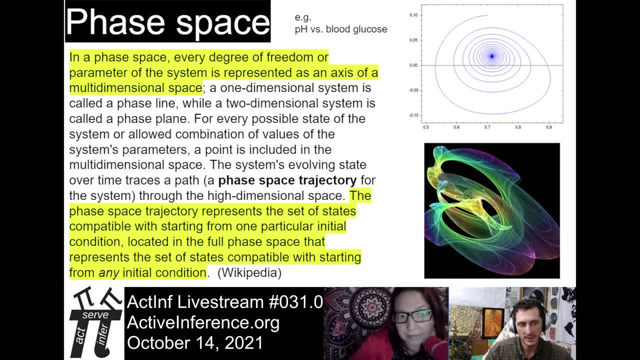 Yes, Base spaces are just kind of the descriptive. It's literally just the space that something can happen in. and then there are trajectories through phase space. well, there's points which just are static values, like three comma four, and then there are trajectories which are like linkages amongst sets of points, and then also out there in phase space are attractors. so in the field of dynamical systems, an attractor is a set of states in the phase space towards which a system tends to evolve. 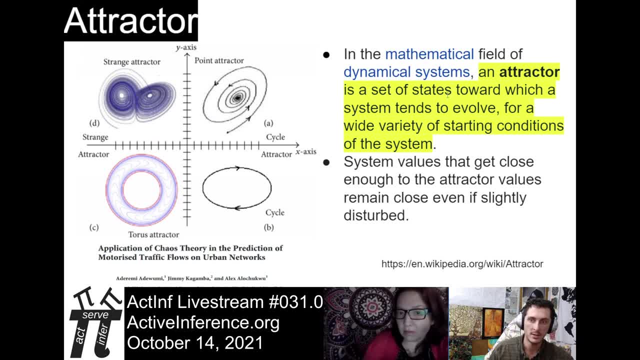 The systemifi is a set of states in the phase space towards which a system tends to evolve for a wide variety of starting conditions of the system. agara and tri Katie's less tense about that, but what Jeff puts forward is that systems and attractor is a set of states in the face space towards which a system tends to evolve for a wide variety of starting conditions of the system. System values that get close enough to the attractor values remain close even if slightly disturbed. 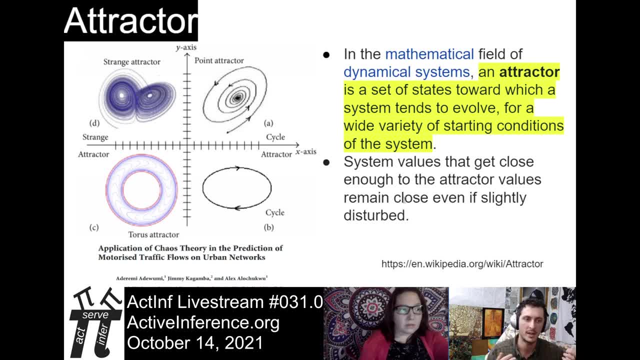 So kind of mental model isn't step forward with a say approach. a different implies. So a kind of mental model there is like a rubber sheet and someone pulls the middle down a little bit, Doesn't stand out quite as you would imagine a system. 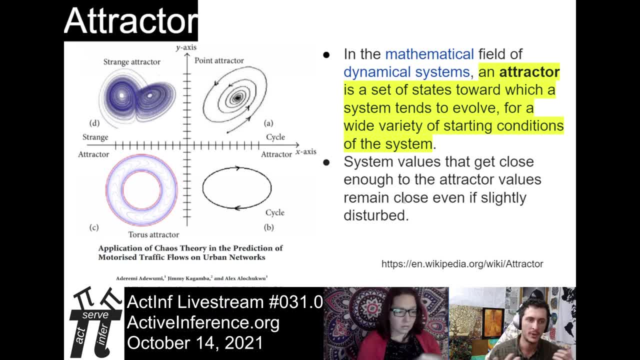 no, that is no an attractor, because things from near or far are attracted towards it and keep Pourke like a see bottom of that. well, they're going to resist being moved away from it and so that's sort of a simple ball rolling into a bowl attractor state, and there's simple equations that govern that type. 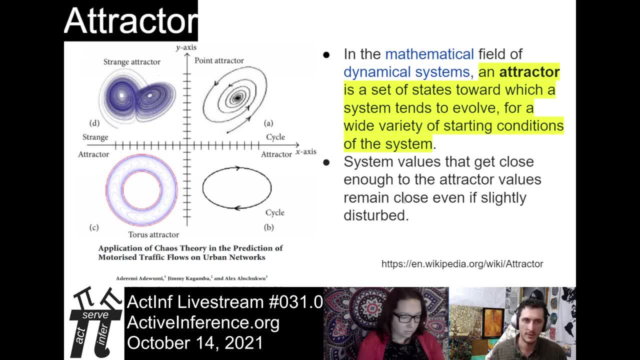 of movement, but in higher dimensional phase spaces there are different geometries of attractors, and then also for biological systems. it is a challenge to model using attractors, but that's what this paper is really about. can we use that model of an attractor to talk about biological? 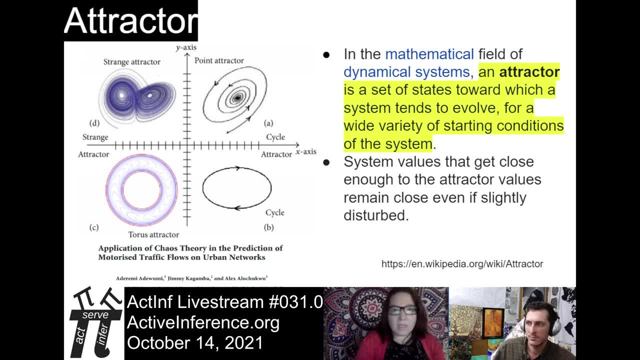 systems and how they regulate okay. so yeah, and i just pulled this image out. actually, i think it was brought up in the, in the paper, and i don't remember if the original author who outlined these four types of attractor, if that was kaufman, i think i feel like it was kaufman, but 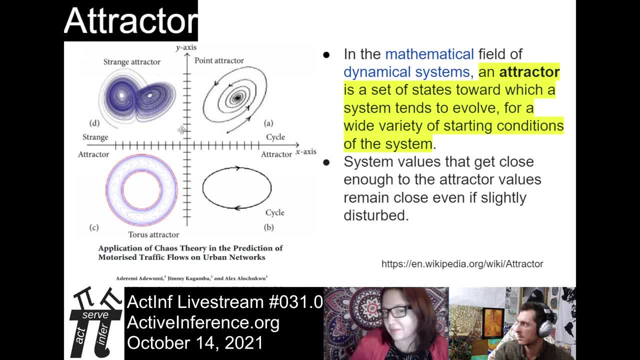 it was cited in this paper as well, about the four different kinds of attractors, and so that's what's shown here- is the strange attractor, the point attractor, the cycle and the torus. um, so just in case you were wondering what those kind of attractors looks like, it's it's a drawn to points in this kind of way. 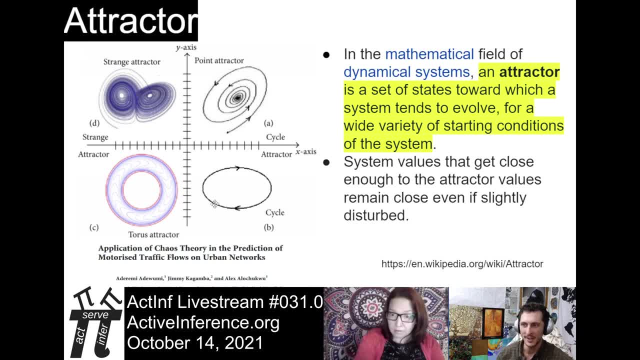 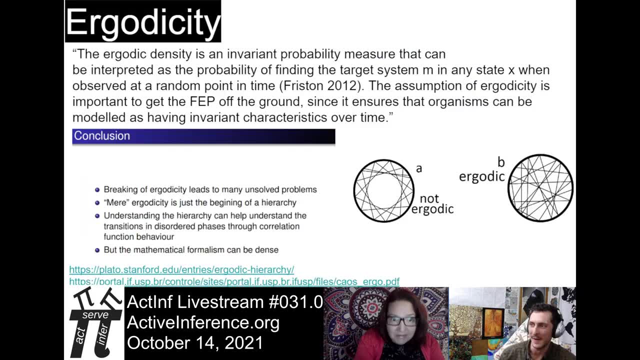 it is also on another phase, space of attractors with its own x and y axis. okay, ergodicity. so this is a quote from the paper, then blue- any thoughts would be cool. so there's a quote from the paper that says that ergodicity is a invariant probability measure, that 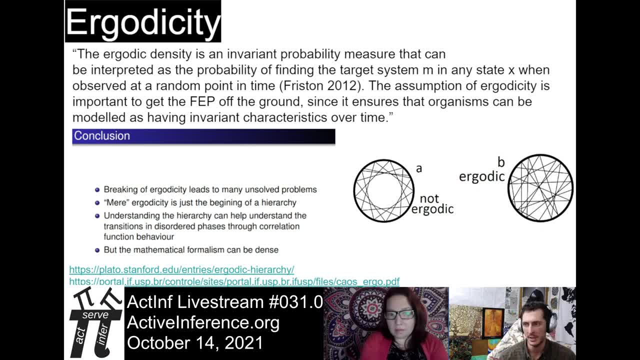 can be interpreted as the probability of finding the target system m in any state x when observed at a random point in time first in 2012.. the assumption of ergodicity is important to get the fep off the ground, since it ensures that organisms can be modeled as having invariant. 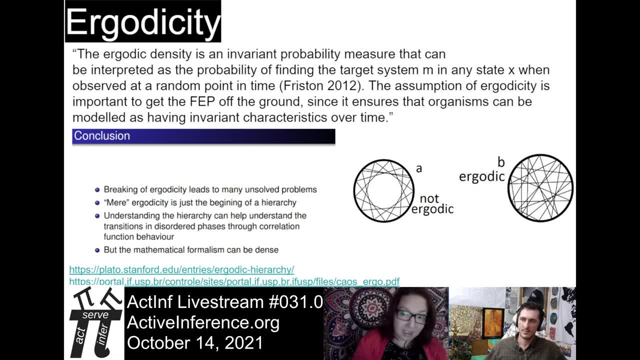 characteristics over time. so just to kind of relate ergodicity to the phase space. so the concept of phase space, that all of the potential points in that space are visited at one point or another, like that is ergodicity. and then the probability that you can find a- uh, the system in that space. 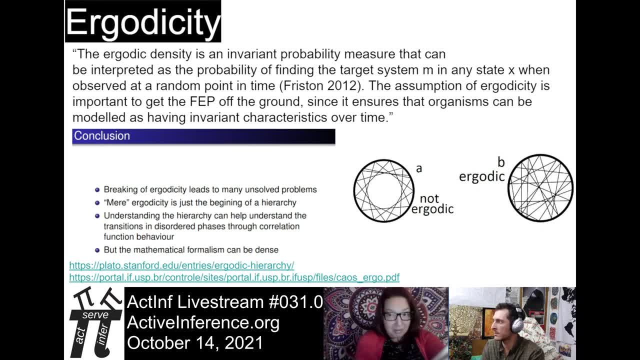 or it at that point in space corresponds to how much time the system spends at that point in that space. if that makes sense, it's kind of a circular loop. but this is just one slide. we're going to return to ergodicity later on, but this is um. 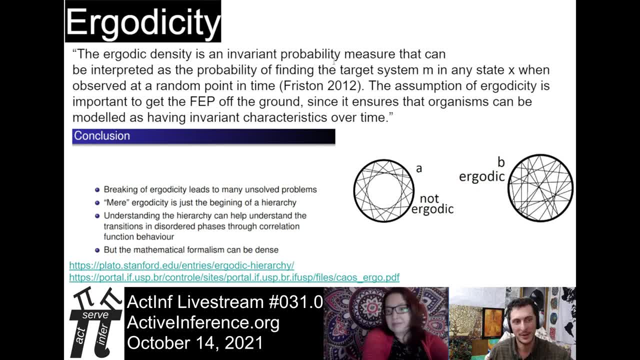 a topic that blue and i like learning about. however, if you know more about this, it would be great to have your perspective, as well as if you're also just learning it and have questions to bring, because there's a lot you could learn about ergodicity and the ergodic hierarchy. so 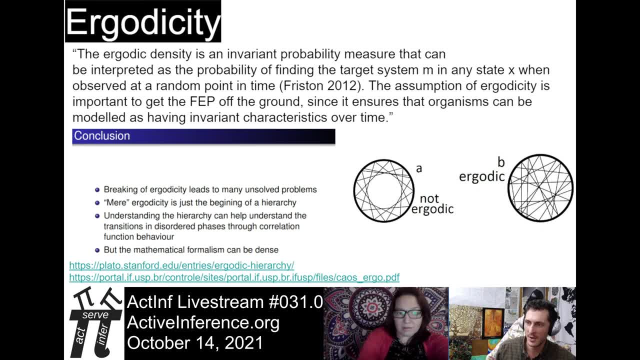 take a dive and then let us know how the water is also getting fep off the ground. i'm thinking: does fep start on the ground? does it start underground? does it start? is it a snowflake with wings? has it always been that way? so no, exactly, it's like the water cycle. okay, so onto. 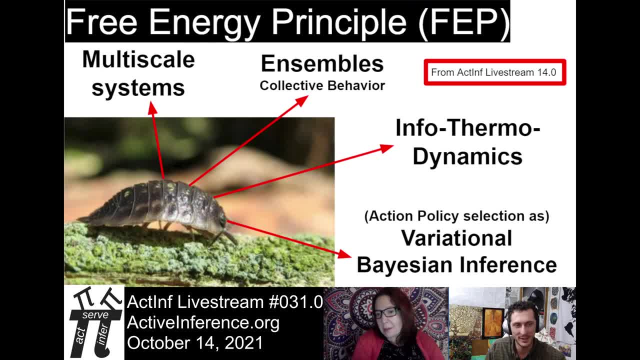 the fep, which is, of course, the target, the system of interest of this paper and in active livestream 14, and before then and after then, we've had a lot of discussions. what is the fep? how does it relate to active inference? and it seems like we'll be working. 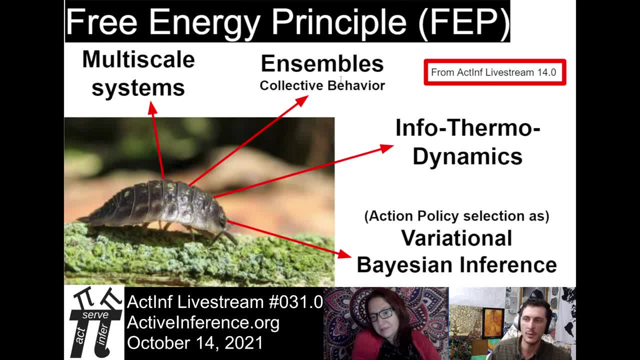 on those questions for a long, long time, but a few pieces that we've pulled out as kind of being good sort of cues to bring up alongside free energy principle and just see them as like cousins or in a network together, multi-scale systems, ensembles like the collective behavior of 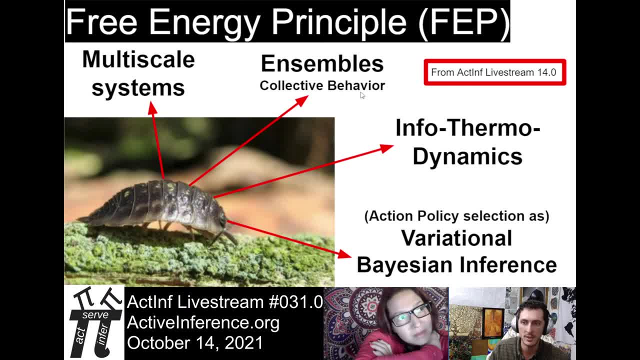 multiple particles or other system subunits, the nexus of information and thermodynamics, which is really like information, thermo like heat and dynamics dynamical systems. So often thermo and dynamics aren't really separated. but we're getting at that delineation And then 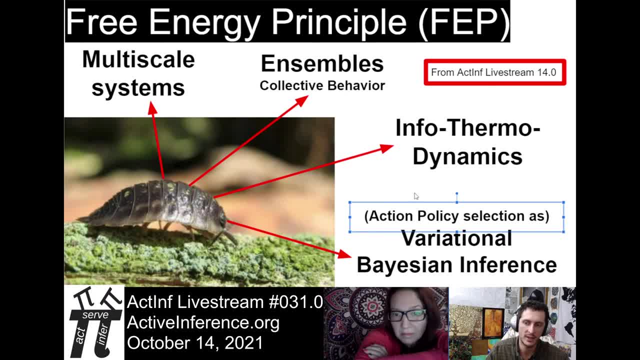 action policy selection as variational Bayesian inference, So using information dynamics to study how policies are selected. and then there's sort of FEP as it is today. And then there's: where could we go and develop with this framework, which is what we'll be exploring today? Any 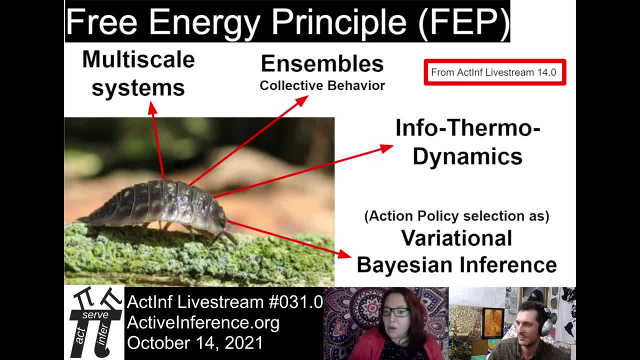 general comments before we get into the paper. Uh, only that, you know you, we haven't. thermodynamics has classically been one word, So like I'm starting to just use info dynamics as one word, just to be like non-discriminatory. 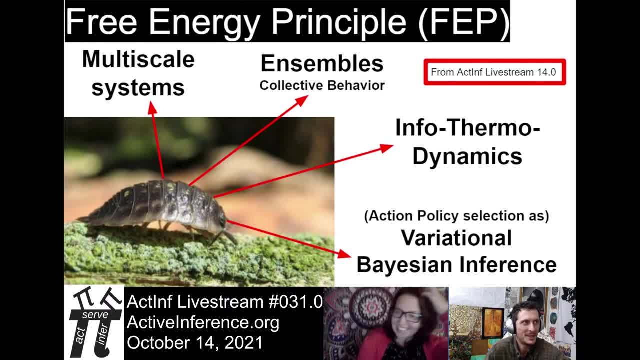 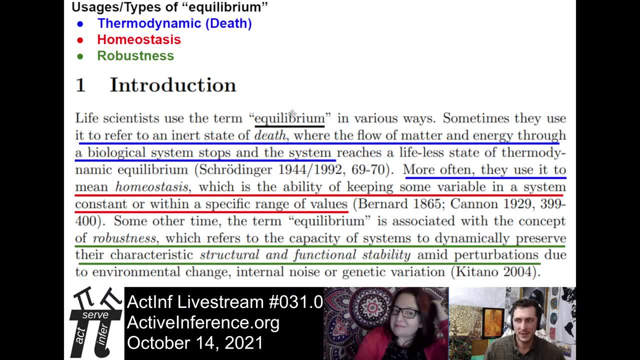 you know, or just dynamics. It's like it's all information, It's all thermo. So, yes, exactly. Okay, Here we go to the paper. This is the first paragraph of the paper, and it's very informative. Life scientists use the term equilibrium in various ways, And so we're. 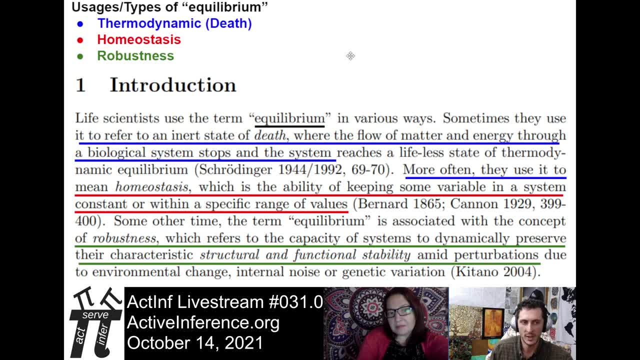 going to look at different definitions of equilibrium, And this is one reason why it's important to have ontologies and have ways of using terms that we can, if not distinguish, at least be clear about in their use. So sometimes life scientists use equilibrium to refer to. 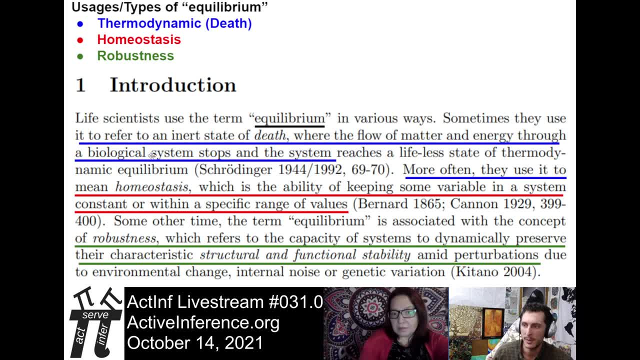 an inner state of death where the flow of matter and energy through a biological system stops and the system reaches a lifeless state of thermodynamic equilibrium. That's sort of the ultimate equilibrium. Then there's the term homeostasis. More often they use it to mean homeostasis, which is the ability 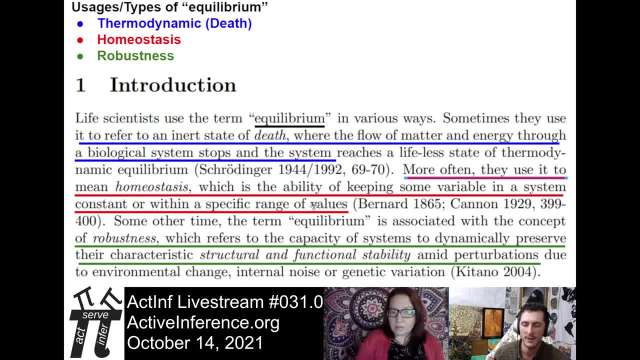 of keeping some variable in a system constant or within a specific range of values, Going back to these old citations for where the term actually arises from. And so that's sort of a living system, So there's parts of it that are consuming energy, hence not at the 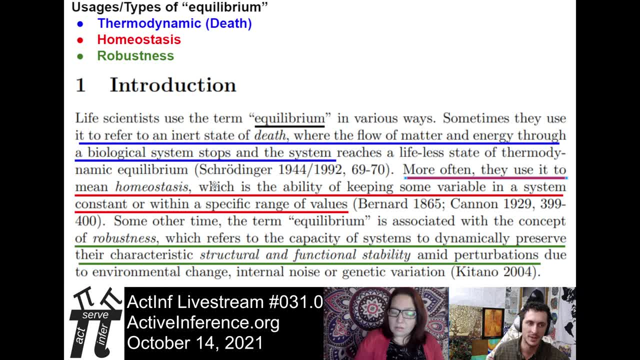 ultimate equilibrium, but there's also other elements of it, at least over certain timescales, that are invariant. Some other times the term homeostasis is the term homeostasis, which is the ability of a system to keep some variable in a system constant or within a specific range of values. Other times the term homeostasis is the term homeostasis, which is the ability of a system constant or within a specific range of values. Some other times the term homeostasis is the term homeostasis, which is the ability of a system constant or within a specific range. 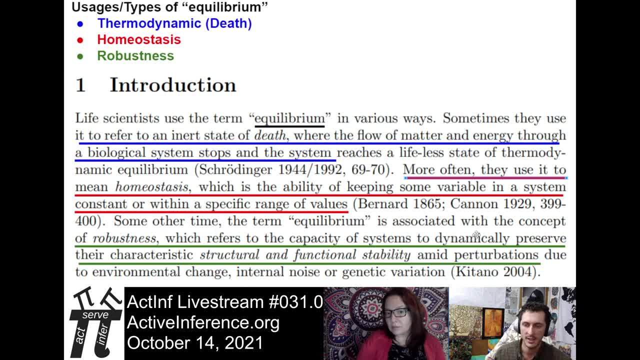 of values, Also called professional related technology. on health science, Some are called Well中共 Stone ad or down 담 than, but over all, products that accumulate results constantly in much larger numbers. I'm going to get these into olderanya, Just using whatever's available there. 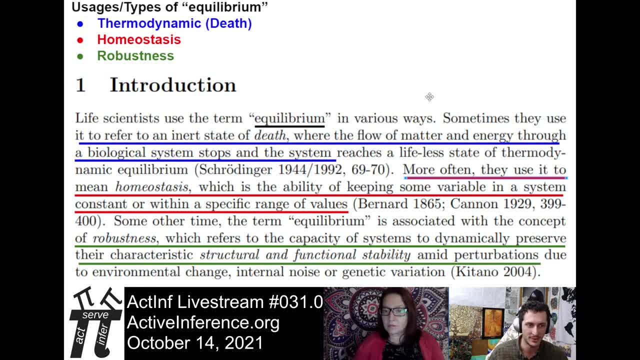 Should be nice. The hashtag is characterize industry of labor, discrimination, normalization, and there's something invariant about the living system, going up into even the idea of robustness, which is that the system is doing something to maintain its sort of equilibrium, like its balance. 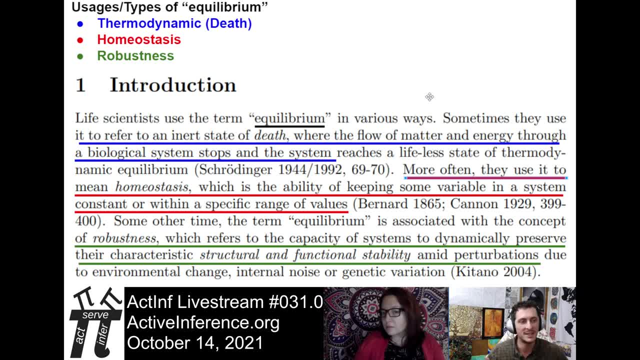 amidst noise, which is maybe seen as a type of homeostasis, but not exactly the same. so any thoughts on why, um these distinctions are matter, are mattering, or why start the paper this way? you know, i'm curious, daniel, like i, i mean, we've been in the life sciences for 20 some years. 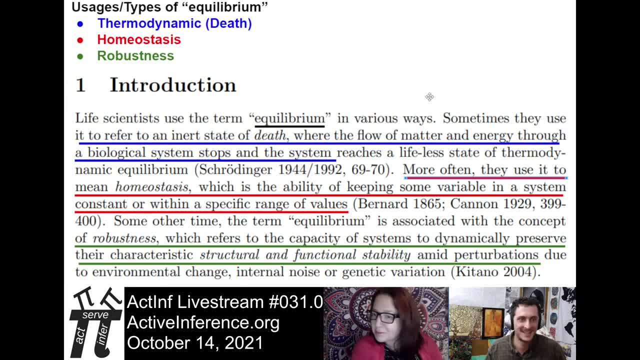 more maybe, um, and i've only used equilibrium, and in terms of life sciences, in the first way, to like as death, um. so i'm just curious, and perhaps this is the the inner chemist in me, but but are you familiar with all of these uses of equilibrium in the life scientists, in the life? 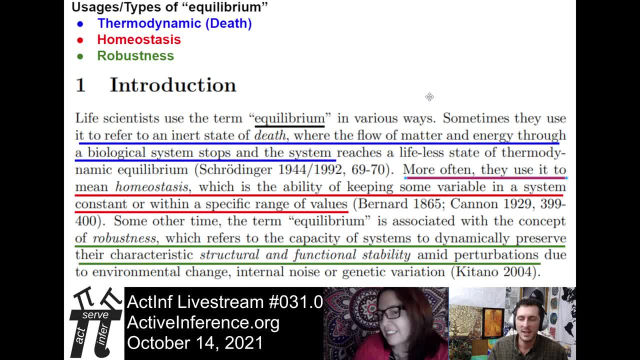 sciences also. i think i've seen the second one. people might not call it equilibrium, but like a buffer equilibrium. well, the carbonate and the co2 in your blood and it's maintaining a buffered, a ph equilibrium. so that's not death, it's a living system that's doing it, but it's. 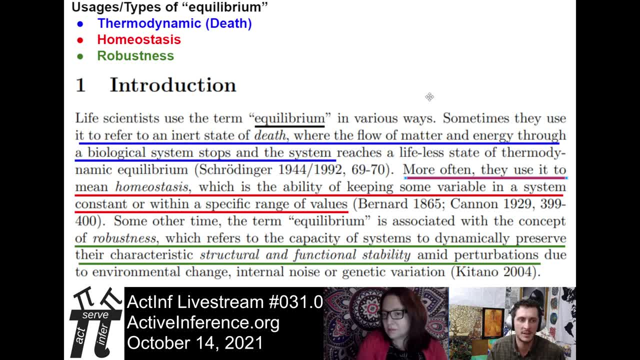 referring to some chemical process that's being kept at a dynamic equilibrium within the scaffold that a living biological system is providing. and, um, i'd also be curious- i don't think we dove into it this kitano 2004 like you. homeostasis to keep something within a range of values. it sounds a lot like robustness. so how are 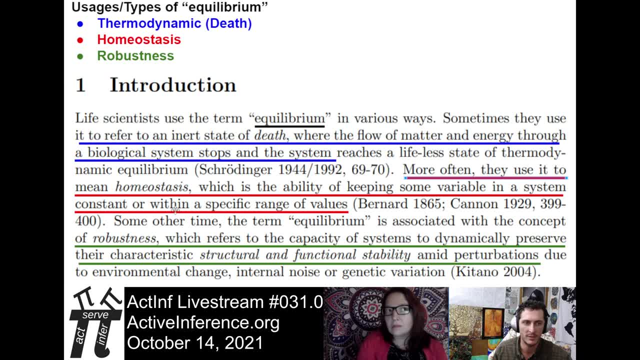 the how are the second and the third definitions different? because, like, anti-fragility is something different, where perturbations actually strengthen the system or cause it to develop, for example. but robustness is a little bit more like homeostasis, but open to anyone's thoughts. we'll. 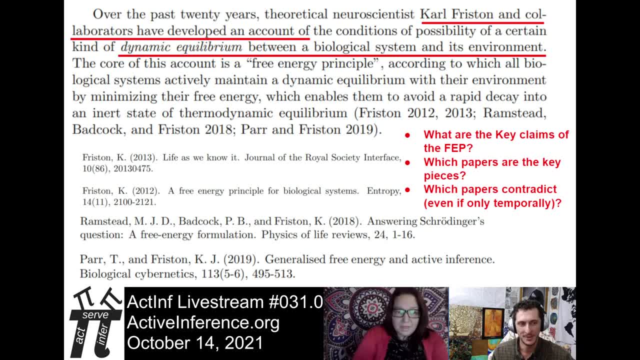 see now on to friston at all. so over the past 20 years, it's giving us some historical context. since the new millennium, theoretical neuroscientist carl friston and collaborators have developed an account of the conditions of possibility of a certain kind of dynamic. 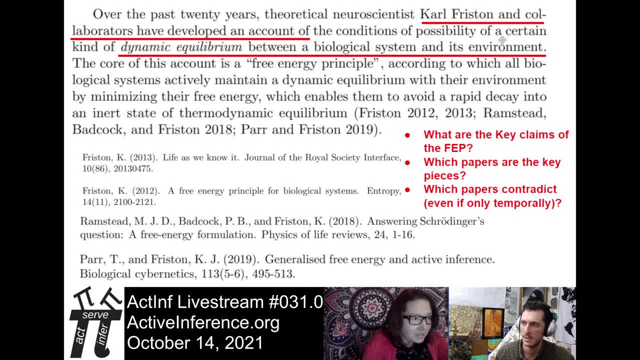 equilibrium between a biological system and its environment. the core of this account is a free energy principle, according to which all biological systems actively maintain a dynamic equilibrium with their environment by minimizing their free energy through inference and action, which enables them to avoid a rapid decay into an inert state of thermodynamic equilibrium. 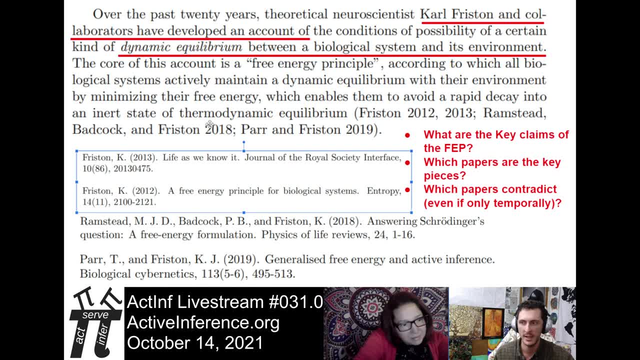 So here's a few of the citations: 2012,, 13,, Ramstead et al 2018, Parr and Frist in 2019.. So here are the papes. If people want to dive into the references, those are always really good places to start. 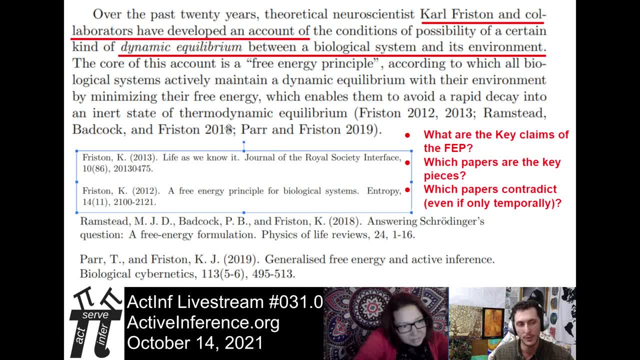 But whether you take the authors at their manifold dimensionally reduced word, or you go into these original papers, or you send a tweet to an author, or you come in a live stream and talk to them, what are the key claims of the FEP? 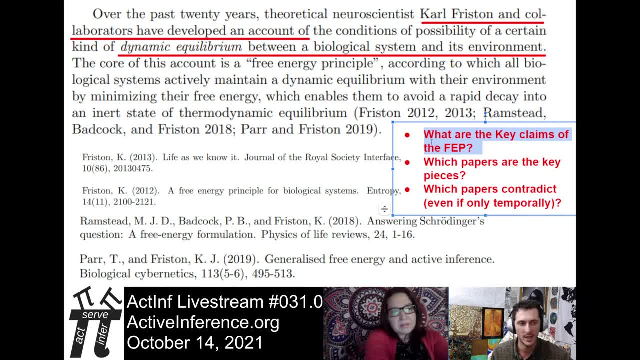 From a rhetoric perspective, what does the FEP assume and what does it claim? Which papers are key to FEP? Not what was important in 2005, from 2002, but today what is important. So how do we respect that? different citations from the past. 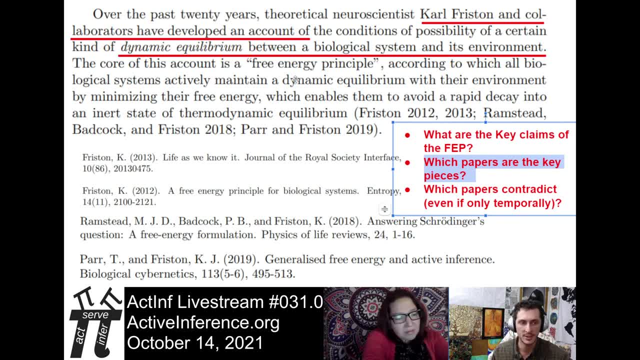 might have a partial picture or use a different formalism. and then which papers are contradictory, even if only temporary, So somebody might make a claim in a 2010 paper. You can't explain situation X And then, like you know, two weeks later, Frist in it all, write the response. 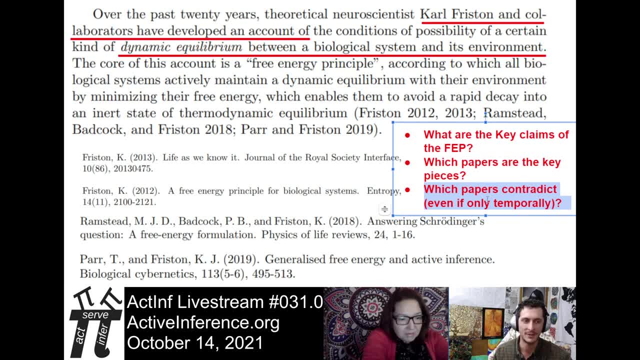 And then some people have. they bought the rumor but they haven't heard the news. So how do you keep a coherent narrative of the literature, as there are errors, contradictions, disconcordances, All kinds of things that just make it less easy than it could be? 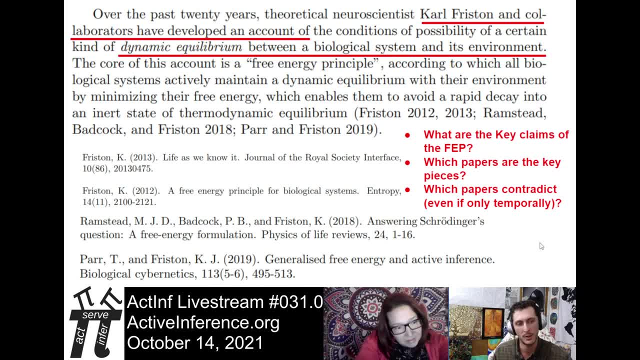 to understand what is happening with FEP, its proponents and its detractors. So just a thought on this and something that I was thinking about as I was reading the paper. and a lot of this is footnoted throughout the paper. but the FEP 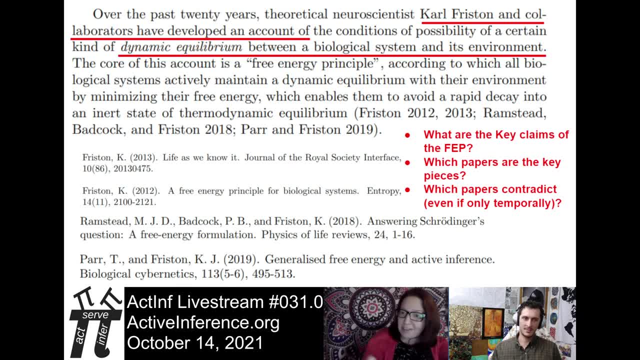 like, has evolved over the last 20 years, So it didn't start off like in the state that it is now. It didn't start off like a completely elaborated theory, And so it'd be really cool to develop a timeline of the FEP. 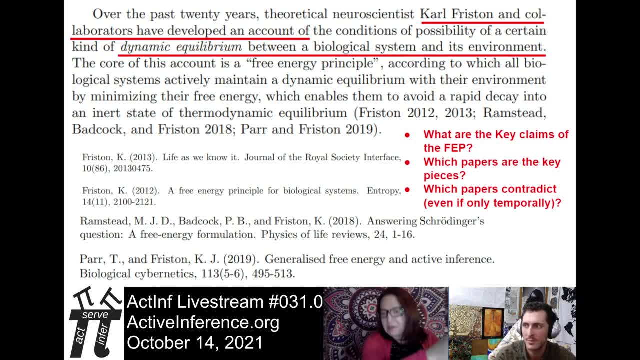 Like first concept, you know 2006 or whatever, And then at what point in time did, like the Markov blanket come into play? And then when did active inference separate from the FEP? and to kind of get like a good idea of 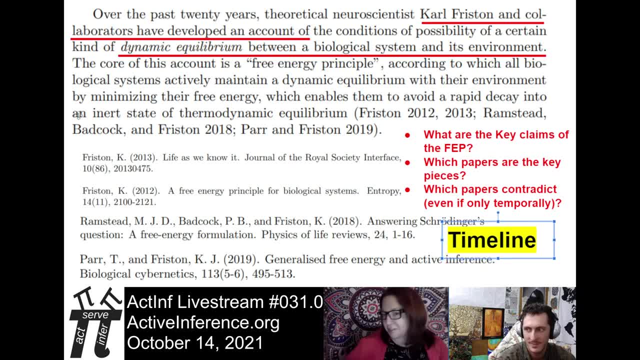 the situation as it's gone through several iterations now. Great idea Blue. I'd hope that in AccDimF, Lab and other groups groups we can collaborate to really make that happen, because to have the timeline of developments and cross-link that with the core terms which we'll talk about later today and then also just 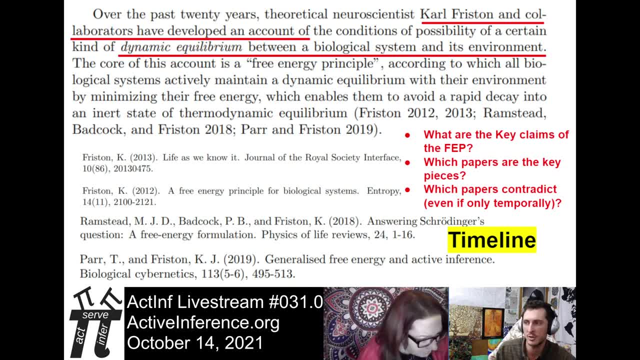 who was involved and what were the contributions. it would just make it tremendously easier instead of just going back to square one, sort of a scholar search, just when we're curious about. hey, has there been something written about free energy and X? okay, so that was sort of the neutral context, or. 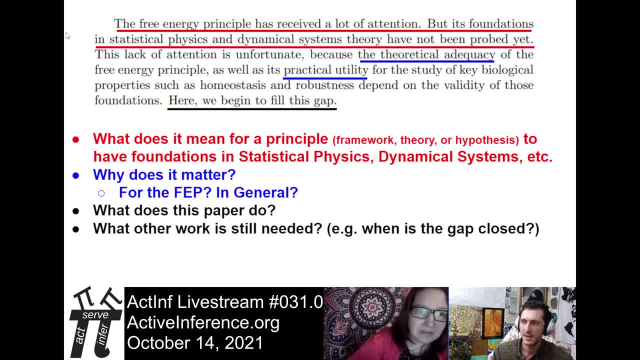 at least not so barbarous. but here's where the authors bring in the, the gap, the free energy differential in the literature and their contribution. what actions are they going to take to reduce the differential? the free energy principle has received a lot of attention. no citations from whom? a lot relative to what? 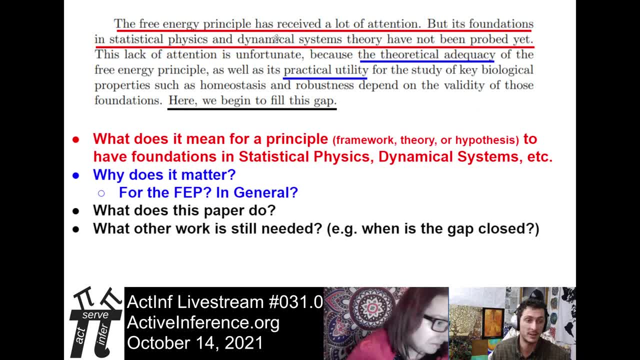 I, it's not. I'm not saying it's incorrect in the paper, just it would be awesome to learn what does it look like to have a lot of attention? What does a Google trends or a book engram viewer search result in? Are we on the up or are we going down from some period of time? So? 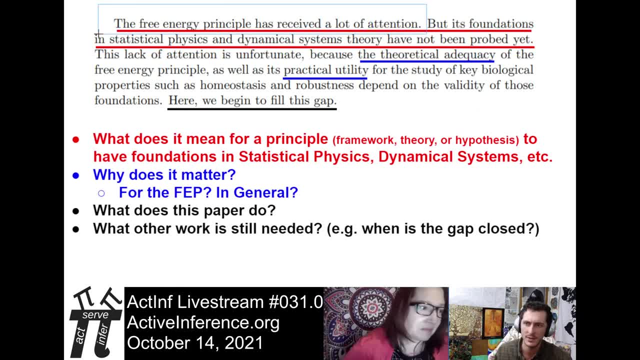 what attention, what regime of attention has the FEP received and from whom? But the foundations of FEP in statistical physics and dynamical systems theory have not been probed yet. That's a claim. Maybe some people will think that they have. So we'll look forward to learning. 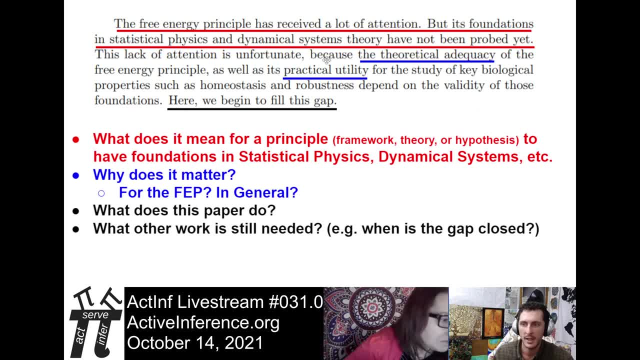 about that. This lack of attention is unfortunate because two reasons: One, the theoretical adequacy of the FEP and, two, its practical utility for the study of biological properties- depend on the validity of the foundations. So it's like we want the house to be beautiful and useful, And if the 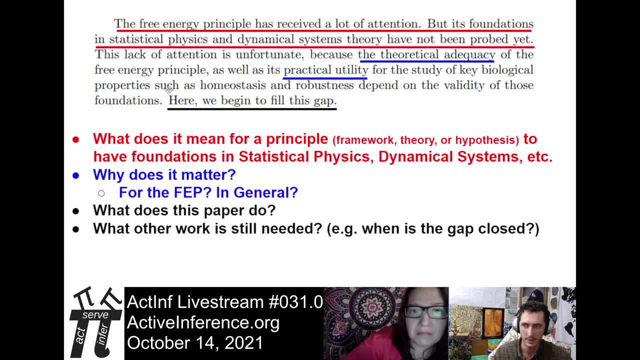 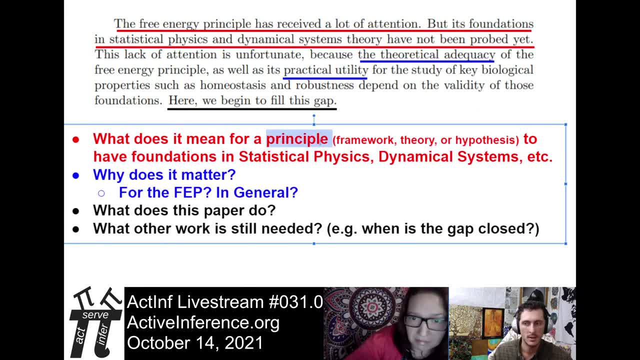 like: what does it mean for a principle FEP? And we can of course have some subtlety with like what's a principle, a framework, a theory, a hypothesis? So let's just kind of roll with it together: What does it mean for a scientific principle to have foundations in statistical 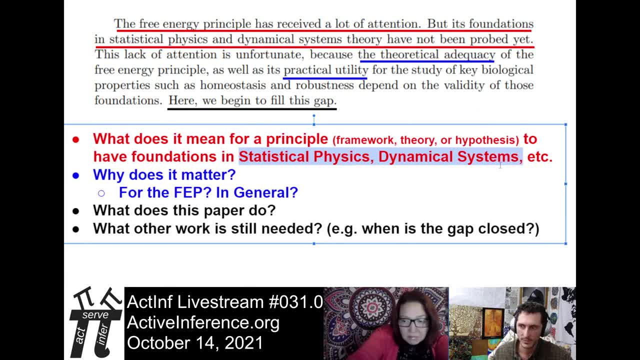 physics? What does it mean for it to be grounded in dynamical systems? Why does that matter? Why does it matter how it's grounded or who thinks it's grounded in what? for the FEP and in general, And then always trying to connect the generalities. 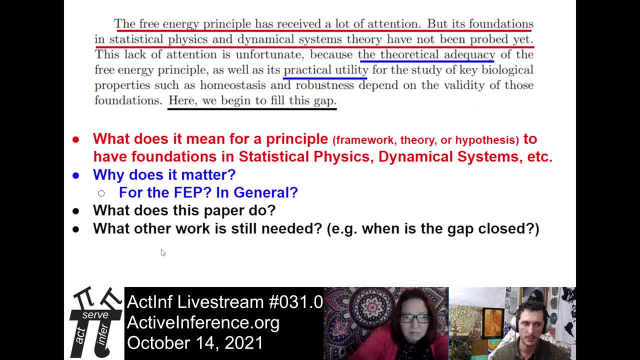 with the minute particulars. What does this paper actually do? And then, what work is still needed? Because it's easy to get caught up in some of these big, sweeping, multi-decade, many person research trajectories And it's helpful sometimes to just separate out what. 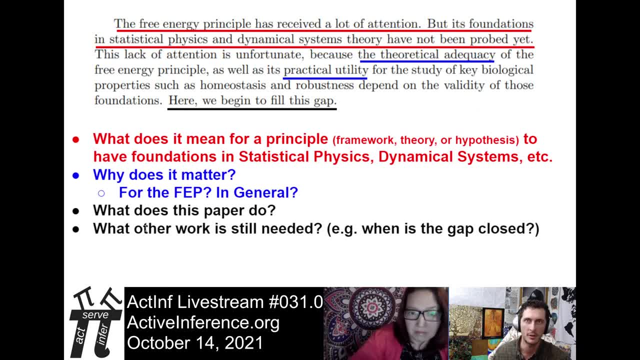 is the purpose of the paper, And then what is the purpose of the paper, And then what is the paper doing? And then what is the bigger picture, like the grand synthesis that has to be done between FEP and some other field, Anything here. Okay, Here's from a footnote and it's to forestall. 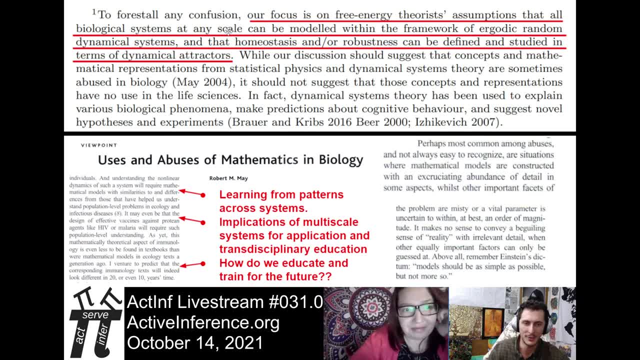 any confusion. Okay, great, All my confusions are about to be forestalled. I love footnotes like that. Our focus is on free energy theorists, not principalists. by the way, theorists: Assumptions that all biological systems at any scale can be modeled within the framework of ergodic random. 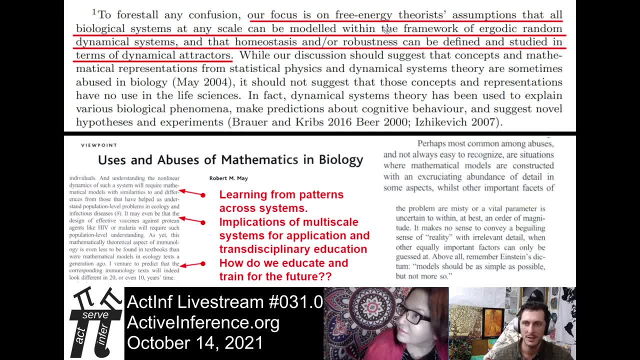 dynamical systems and that homeostasis and or robustness can be defined and studied in terms of dynamical attractors. So I don't know if that's a assumption of all FEP colleagues. I don't know if it's a rather than an assumption but rather a consequence, Like there are assumptions that 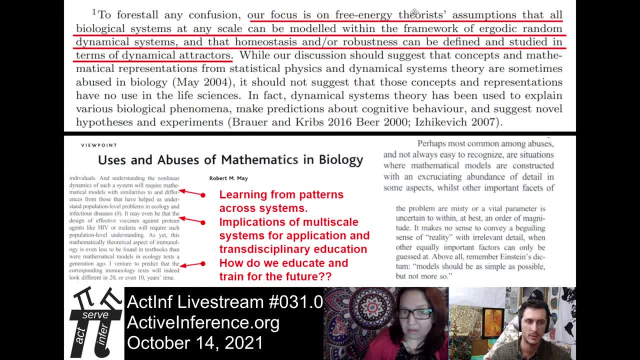 people use, but then actually they have come to this claim as a consequence, not as an assumption or an ungrounded axiom. And while our discussion should suggest that concepts and mathematical representations from statistical physics and dynamical systems theory are sometimes abused in biology, it should not suggest that those concepts and representations have no 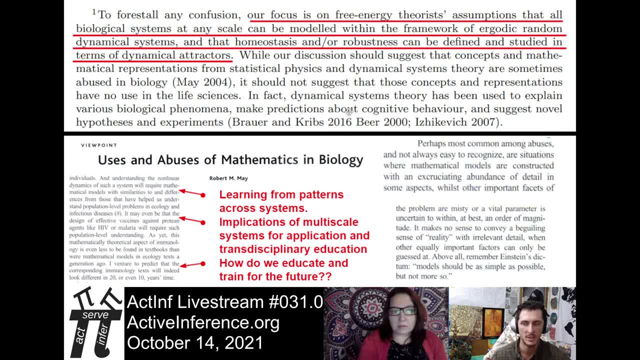 use. So it's saying: in fact, you can have good explanatory predictive models that involve dynamical systems. So it's not saying math and biology is hopeless. And then also this 2004 paper by Robert May, a famous biologist, who says that you know, math gets abused in biology. So this is. 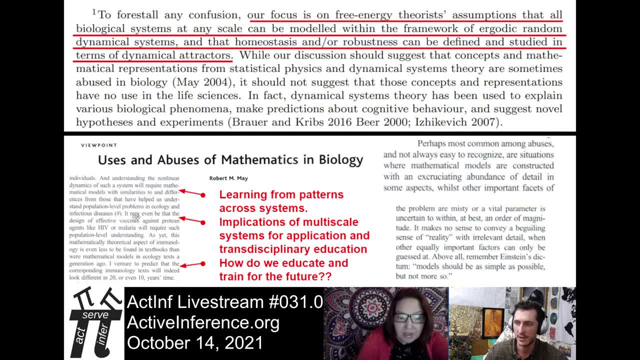 Robert May, a famous biologist, in 2004.. And this was just very interesting, like understanding the nonlinear dynamics- And this was in the case of a virus and health situation, just extracting some of the key memes. It's like we're going to have to learn across systems. We're not just going to 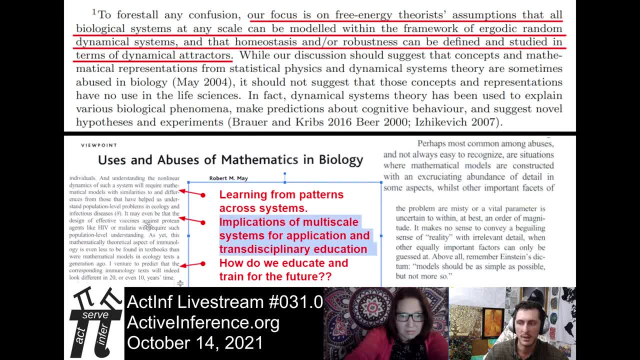 be able to have one default system. We need to think about multiple systems. We need to think about multiscale systems for applying and educating in transdisciplinary contexts like having an understanding of viral dynamics is going to require population and ecological understanding as well as protein, And then I venture to predict that the corresponding immunology 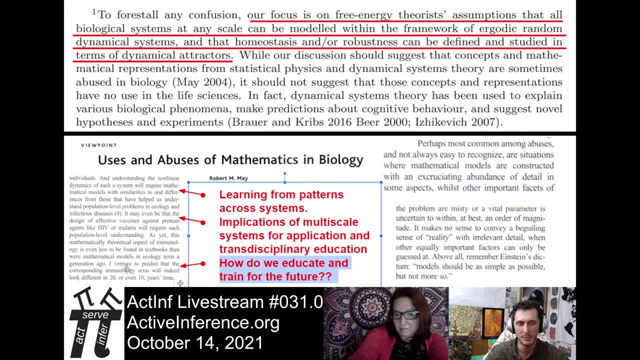 text will indeed look different in 20 or even 10 years time. Okay, well, we're right, between 10 and 20.. And maybe immunologists are starting to go. oh yeah, you can't just talk about what's in. 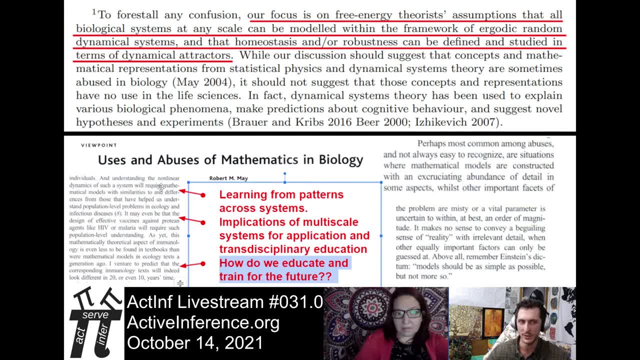 the what's the white blood cell touching the pathogen? There's a bigger picture, there's a society. And then what are those abuses? And they're not always easy to recognize, especially because few have the expertise or the confidence or the personal narrative that they're able to. 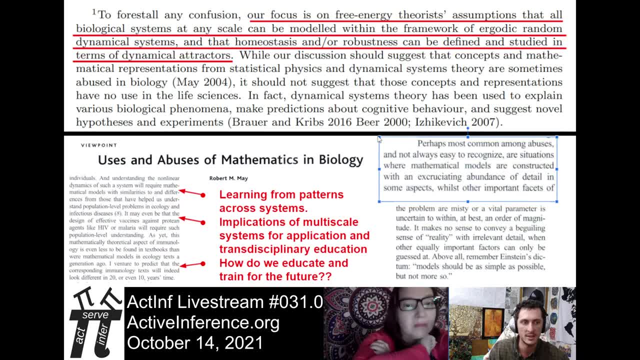 ask questions across disciplinary contexts. So it's easy sometimes for something to be transdisciplinary And then like, the biologists don't question the physics and the physics don't question the biology, And all of a sudden something is not really getting questions. So it's totally a great. 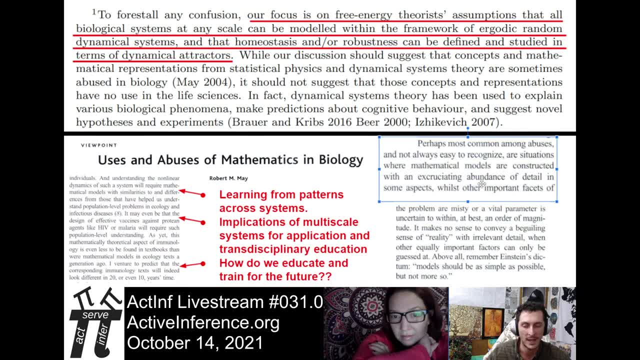 point- And this is a really important kind of fallacy, essentially- where a mathematical model is constructed with an excruciating abundance of detail in some aspects, while other facets of the problem are misty or vital parameters uncertain within a massive range, And this happens just so. 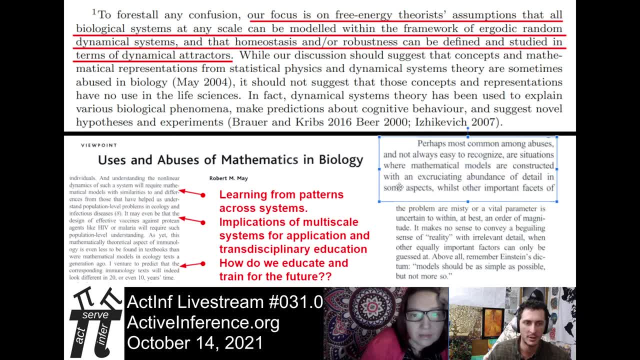 many places It's unreal. We made a mathematical model of this. oh well, you know, of course we didn't consider other factor, ABC. So it's not that everything has to be a theory of everything, But we have to recognize that. 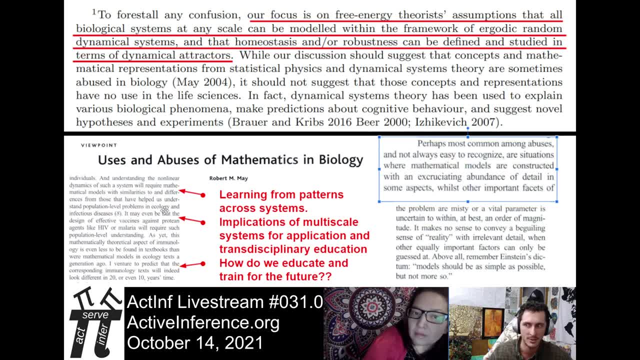 extremely partial. mathematical models in biological systems may be less helpful than people claim them to be, And it might be better if people pooled their efforts and work towards better models. Any thoughts on that? Just you know, I mean I think I'm definitely guilty of, like I remember back to Mike Levin's. 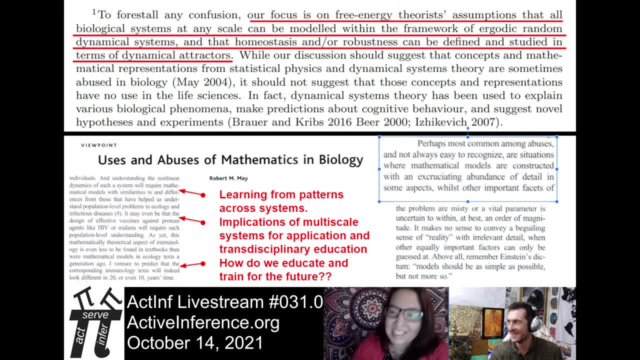 live stream when we were abusing physics. Um so guilty as charged sometimes, But but it's. it is important to you know, have an open dialogue and to ask questions, like if there's a concept or something that you don't perhaps understand. 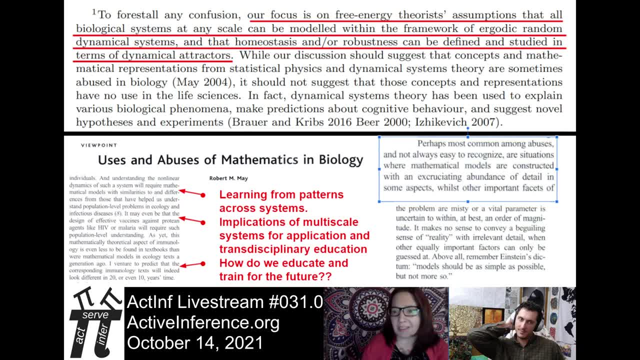 maybe, like you feel like you're a beginner. I mean, I've definitely felt this way, like maybe I'm just being dumb, But you know. and then there's actually a very valid question at the end of that sentence. So if you don't understand something, be sure to ask until you do. I think 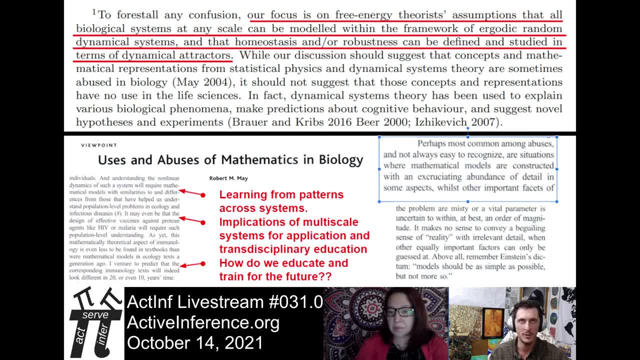 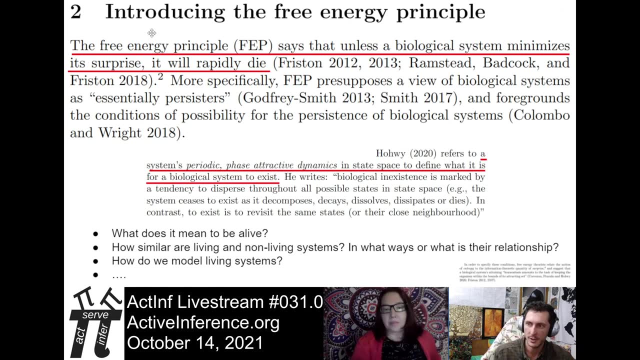 Yep. Sometimes somebody has said: oh, FEP, does that apply to living systems? And so yeah, it's a done deal. Well, you know it's not a done deal, So the conversation is still happening. Here we get to section two, introducing the FEP, The free energy principle, FEP. 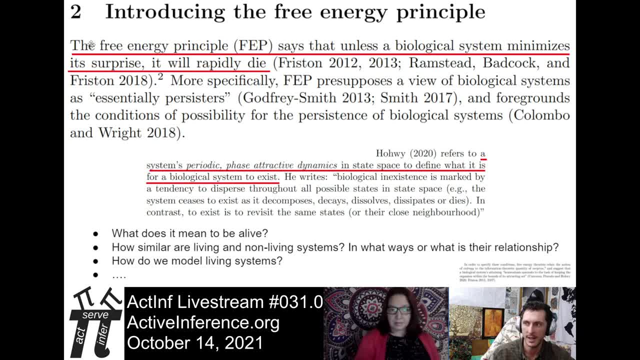 says that unless a biological system minimizes its surprise, it will rapidly die. Now, what do those citations say? Do they talk about system death Or do they talk about system persistence? More specifically, FEP presupposes a view of biological systems as essentially 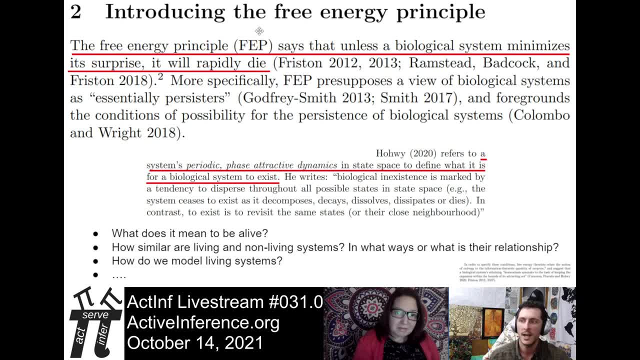 persisters- different authors here- and foregrounds the conditions of possibility for the persistence of biological systems. So that's their top level. take on FEP And then to connect a few of the keywords in Howie 2020 refers to a system's periodic phase, attractive dynamics, so 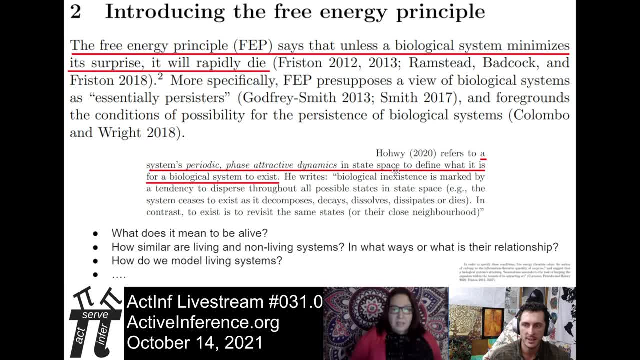 attractors in the phase. Howie writes, biological inexistence is marked by a tendency to disperse throughout all possible states in state space, eg a system ceases to exist as it decomposes, decays, dissolves, dissipates or, alliteratively, dies. In contrast, to exist is to revisit the same states or their 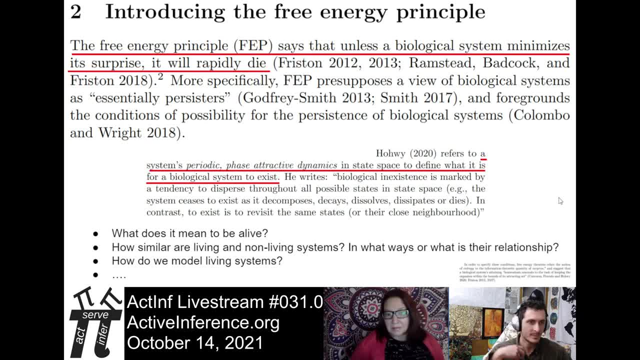 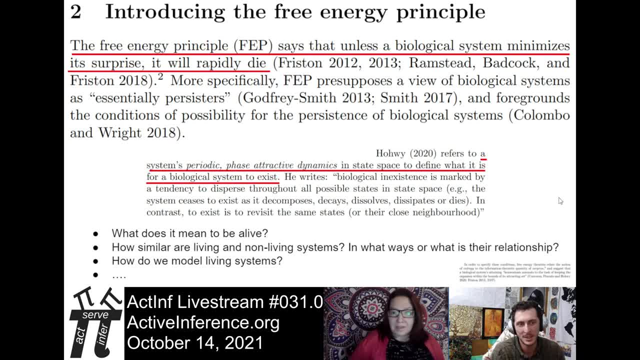 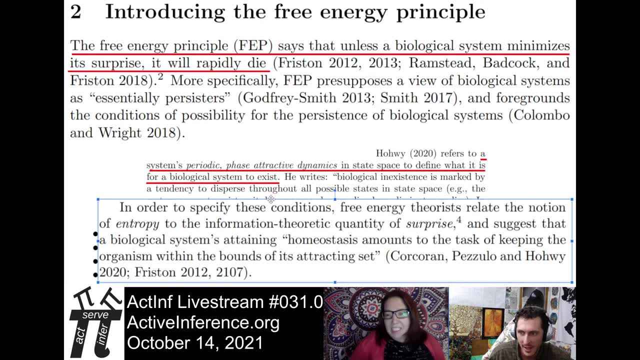 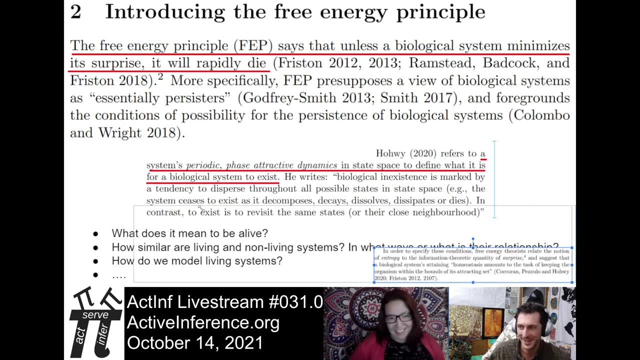 that resist dissipation, systems that have a dynamic equilibrium. What is the phase space we're talking about? These are the big questions we're getting at. And how does one disperse oneself? exactly, Yes, And how. I think we heard that from somebody earlier today: somebody was getting dispersed. 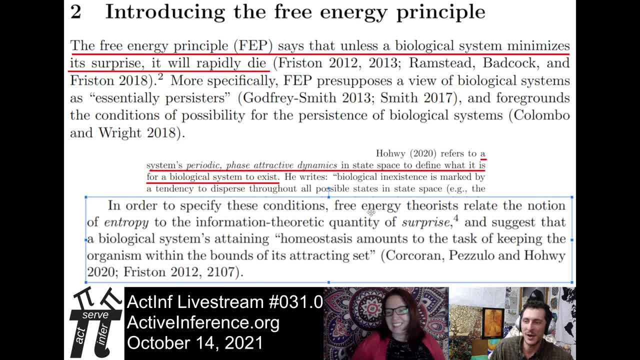 during a practice, this talk, it happens. and where's surprise come into play, not just the psychological like wow, i was surprised, it was a surprise birthday party. but how do we go from attractors and dynamical systems to this statistical, bayesian concept of surprise and attracting sets and lower dimensional? 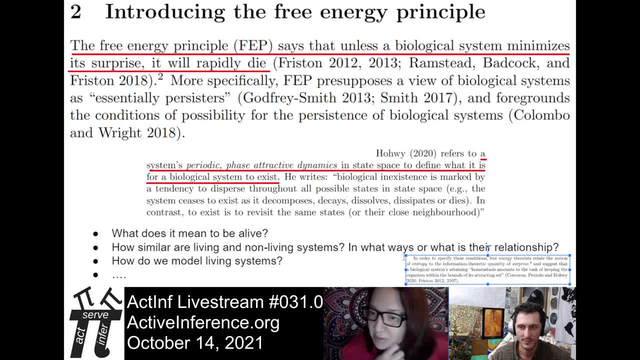 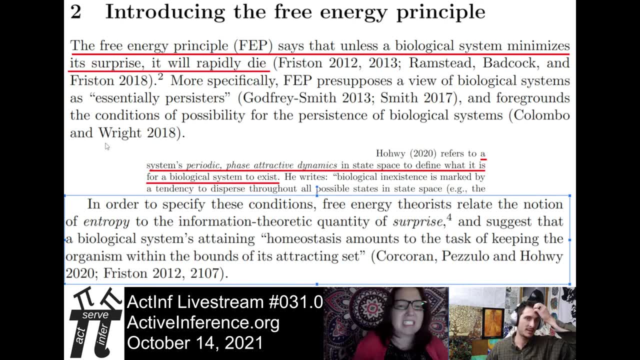 manifolds in attracting sets. make that, make that quote big. one more time for me, okay. so something i i thought was um just unique or or maybe remarkable, was it says: free energy theorists relate the notion of entropy to the informatic information theoretic quantity of surprise. 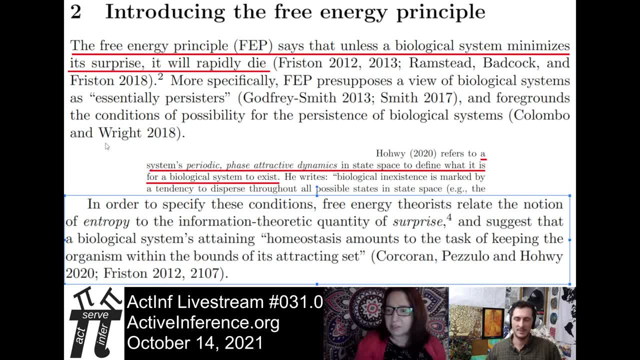 but i think that this is done before the free energy principle arrives like. so in information theory that's claude shannon makes the relationship between information and entropy and surprise. so i don't think that that's a something that the fep started doing well. two: 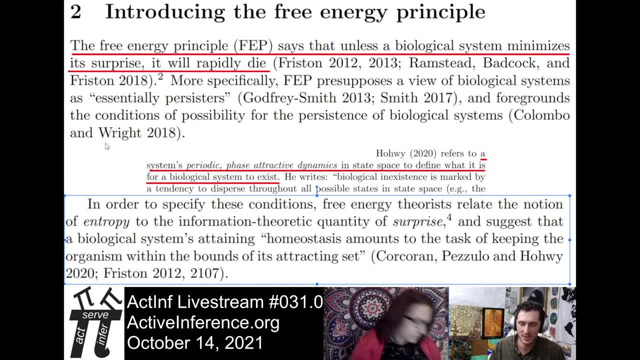 two, two. the themes will return to today and again and again, which is like first. this shouldn't be a pate versus pape battle. this isn't a battle royale, for whose hot take will reign supreme. we should be collaborating on bigger research agendas and so clarifying the contributions. 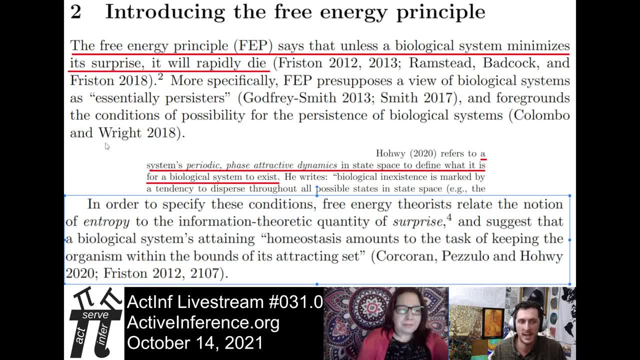 that different people have made will help demystify and make active inference and fep more accessible, because which claims or which contributions were made like a hundred years ago- not that that makes it more valid- but weren't made recently. but sometimes when we only see recent citations it can be easy to get swept up. but 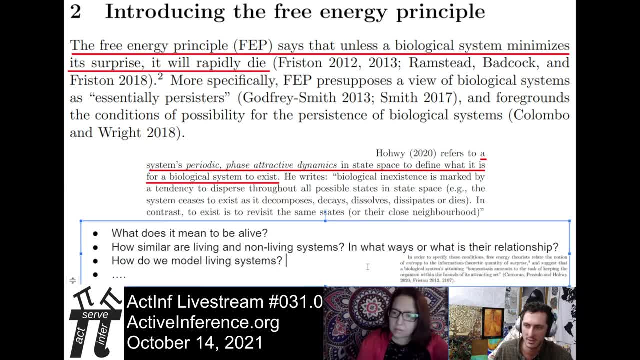 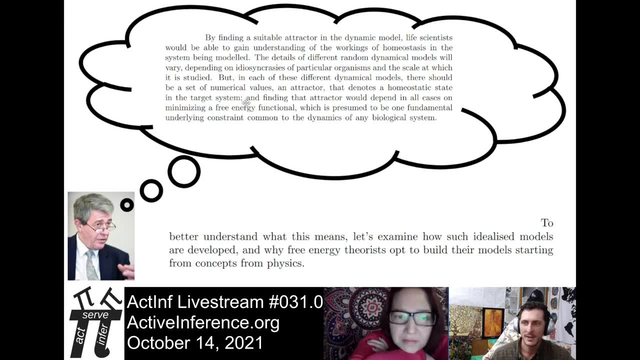 actually, the authors of this paper do a good job of going back to some original citations, but these are big, eternal questions. here's a fun paragraph in the paper, um, because it's sort of like: uh, i i reformatted it slightly because it it shows that we're in. 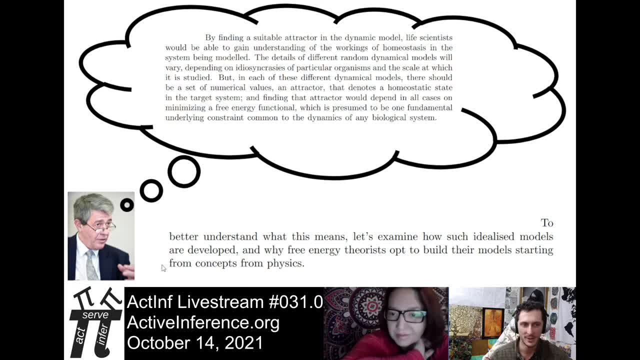 synchronous and asynchronous discussion with friston at all. so here is, like you know, here's him thinking slash, saying first and saying: by finding this is friston's claim pseudo-first and claim not actually his quote- by finding a suitable attractor in the dynamic model life scientists. 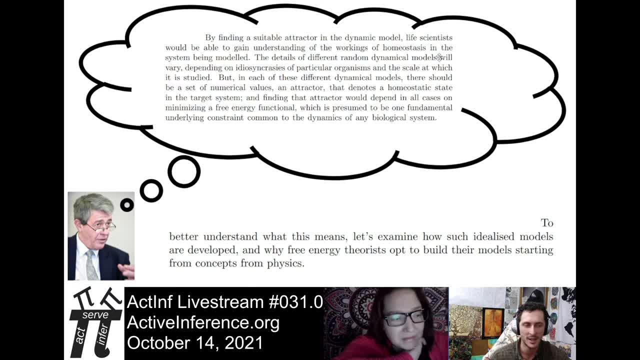 would be able to gain understandings of the workings of dot dot dot. basically like. this is the dream of active inference that if we had a tractor, phase bays, all these terms coming together, then we could just make it work for diverse biological systems. and then the authors of the paper right to better understand what this means. let's examine how such 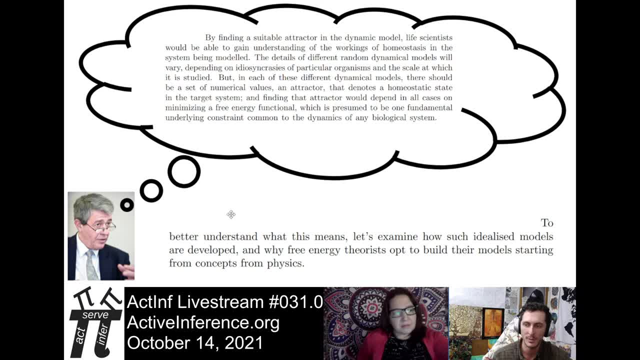 idealized models are developed and why free energy theorists opt to build their models starting from concepts and physics. so this is like the dream of active inference and physical groundings for biological systems. and then the authors do the right thing, which is to um to steal person. the 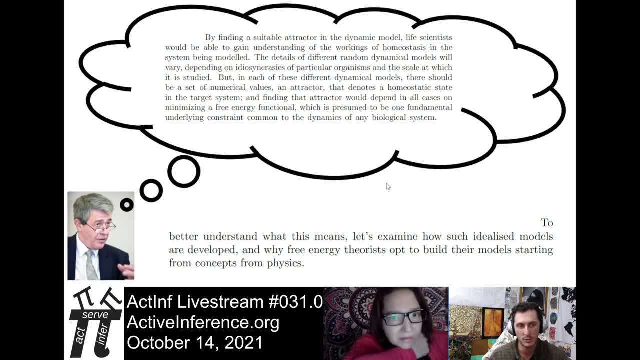 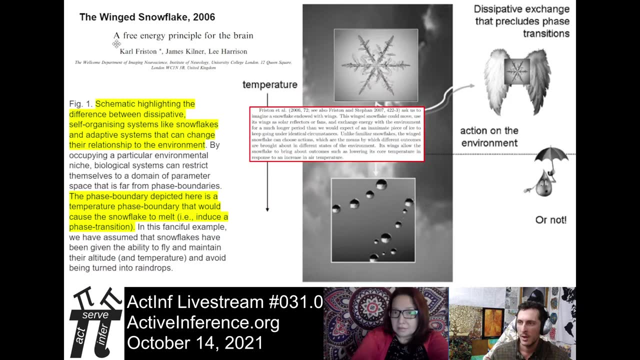 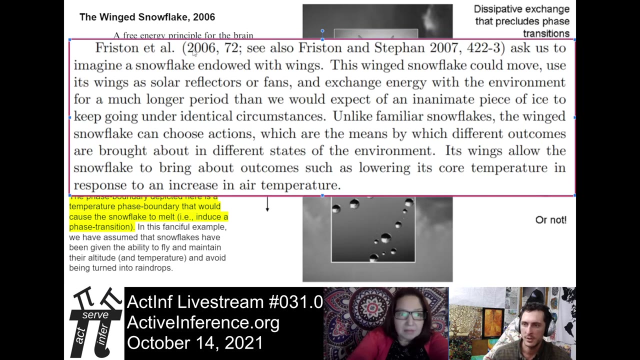 argument, to investigate what its actual strengths are and why somebody would want to make that argument or why this is something that we're motivated to pursue, instead of just immediately critiquing it as, like, not an important thing to want. okay, all right. so here is in the red quote from the paper. so friston at all 2006. 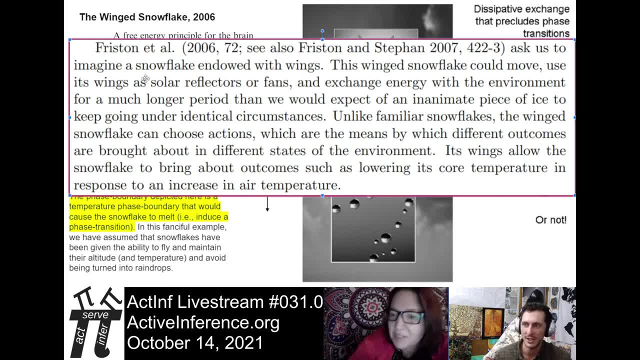 way long ago, way, way long ago. ask us to imagine: were you even born? were you even born yet? oh please, blue, oh please. ask us to imagine a snowflake endowed with wings. this wing snowflake could move, use its wings as solar reflectors or fans and exchange energy with the environment for a much longer period than we. 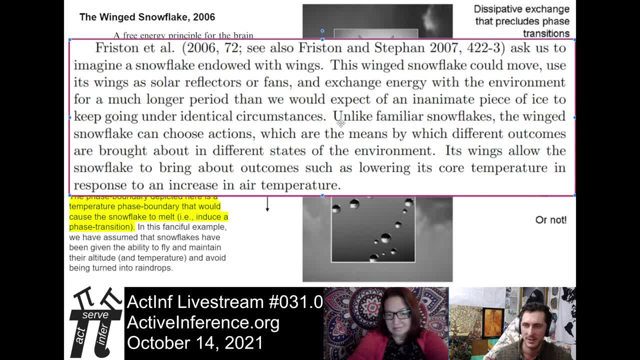 would expect of an inanimate piece of ice to keep going under identical circumstance. unlike familiar snowflakes, the winged snowflake can choose actions, which are the means of by which different outcomes are brought about in different states of the environment. its wings allow the snowflake to bring about outcomes such as lowering its core temperature in response to significant 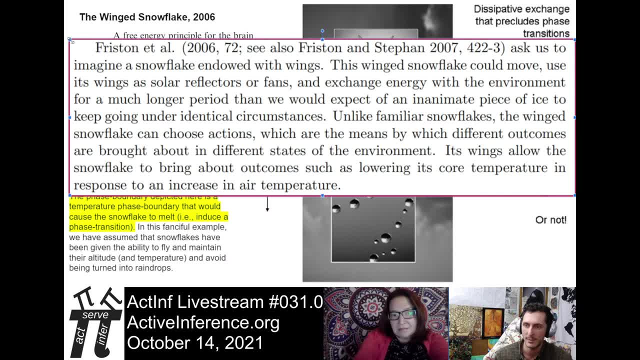 sanctions the wings of the snowflake allow activity while the opposite allows activity although this will bring other 동ậ� � but sensENEGpied Arizonae in a new way is not a antes de laumesna this lowering its core temperature in response to an increase in air temperature so let's go to first 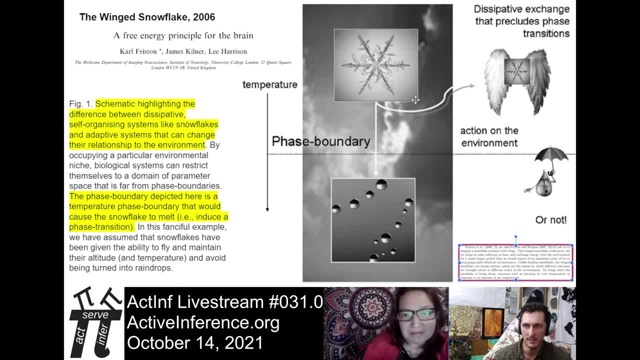 in 2006, and this is figure one, so we're imagining they're sort of on the left is like a traditional snowflake model. they're sort of. it doesn't have any action affordances, so it's just being tossed around in the soup and it freezes when it's cold and then when the temperature gets below this. 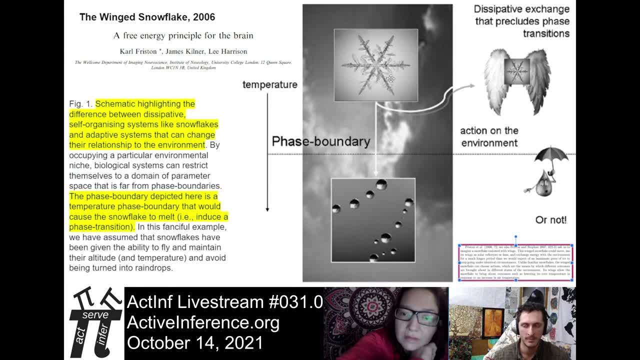 critical phase boundary. it melts and the system fails to persist. so it's, like you know, checkpoint. are we good with systems persisting versus dissipating? this is kind of our simple physical example: a piece of ice freezing in the sky and melting all right now. let's imagine if the ice 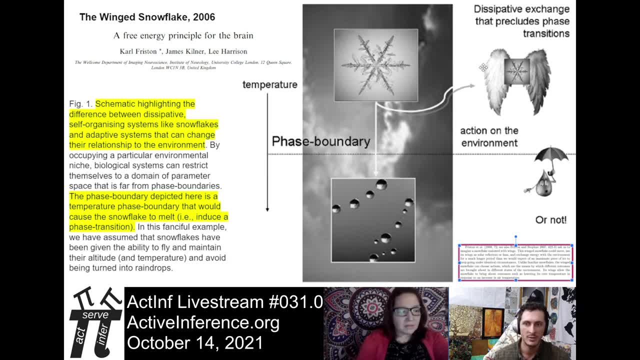 froze in a way where it had wings and slightly different colored wings, but it has these two different wings and that allows it to engage in action on the environment. so, for example, if it detects or predicts, or acts as if it's predicting that it's going to head. 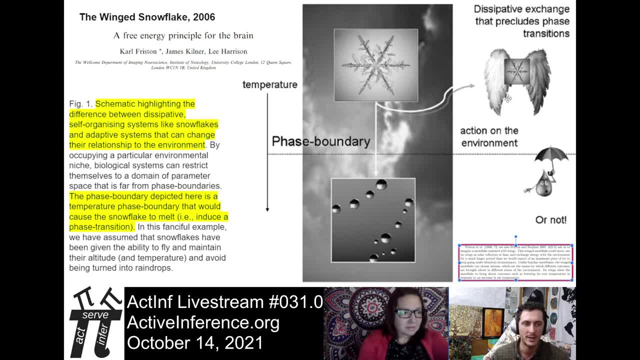 towards a warmer area. that's like you know, lower down or something. all of a sudden it can flap a few times and get into a colder area. so here this snowflake just falls, but this one is able to flap and stay cold, and so, through action, it can get into a colder area, and so that's why it's called. 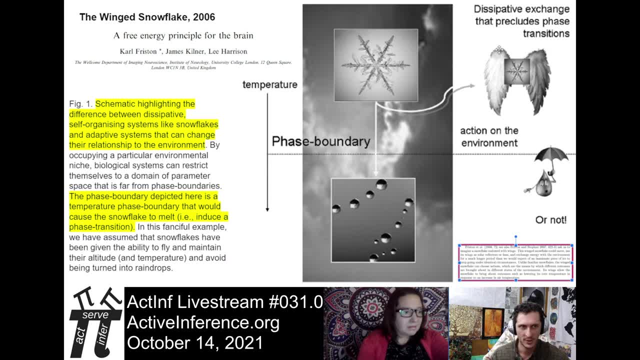 the ice freezing system. it's able to persist longer, so it's precluding a phase transition from solid to liquid through this active exchange with the environment. so that's like the winged snowflake model. that's kind of a nice thought experiment from yonder to help us understand like. 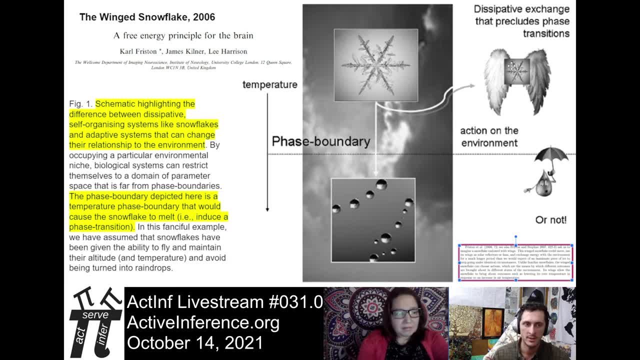 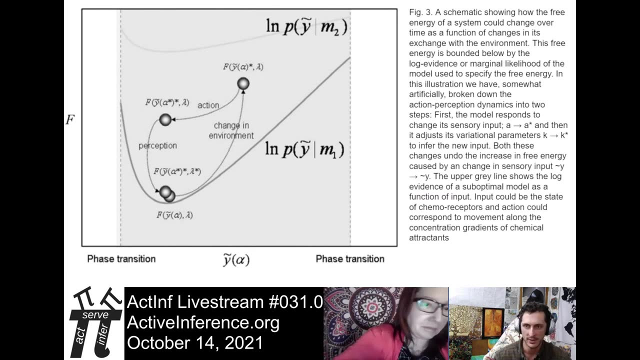 the steps from mere physical system to systems that start to engage in actions on the environment, especially those that keep persistence of the system. anything here? okay, here's figure 3 from that same friston 2006 paper, and this is really an awesome figure because it shows some concordances between active, even though it it's not even really used in those. 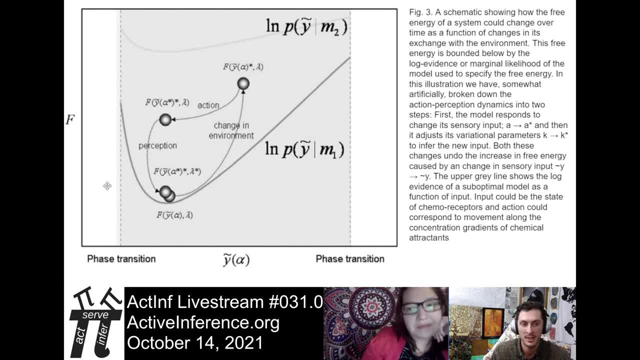 terms. so that's why we need the timeline like is active, even mentioned in this paper in 2006. it might not be actually, but But we can see. there's this perception action cycle And this is related to a few other kinds of action perception cycles. footnote paper- incoming. 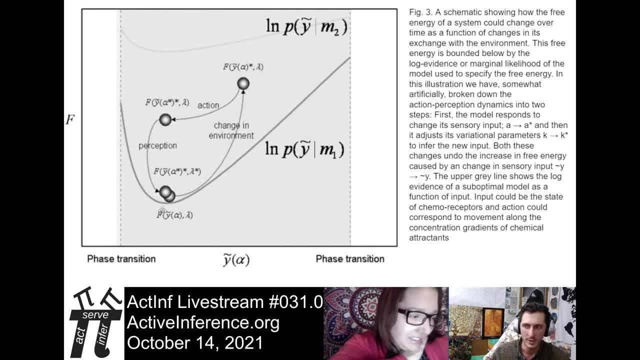 We can think of this as like a bowl, And then the ball is rolling to the bottom of the bowl. It's an image we return to again and again. Now, the Y-axis is the free energy, And so here's the minimum possible free energy. 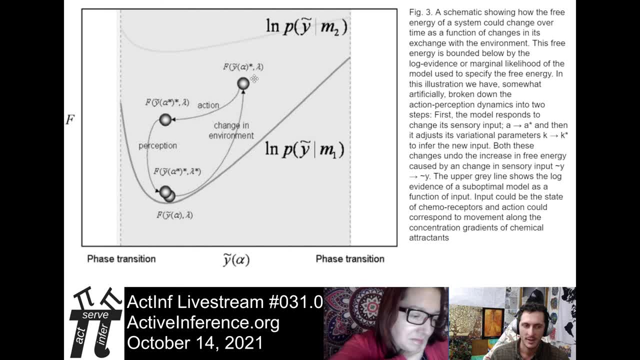 And it's like the system starts here. There's a change in the environment And that causes a mismatch. That mismatch can be reduced through two different types of updates of a model: One is an action and the other is a perception. So which order happens? details, details, details. 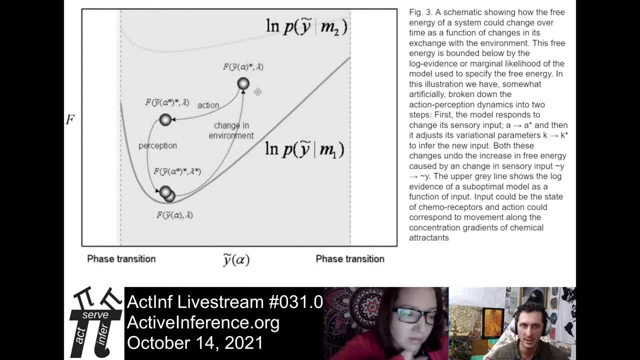 But the idea is like at each loop there's an environmental change which is then renormalized or returned to something through perception and action which relates to an active inference, how we say that the two ways that free energy can be minimized. 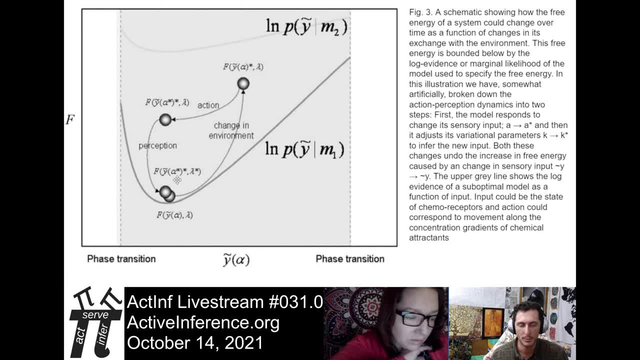 are through updates of the generative model, like learning or parameter updating, or through action. How do we reduce surprise, Inference and action? Why reduce surprise? Because if we have an optimistic generative model, we don't want to be surprised about our model. 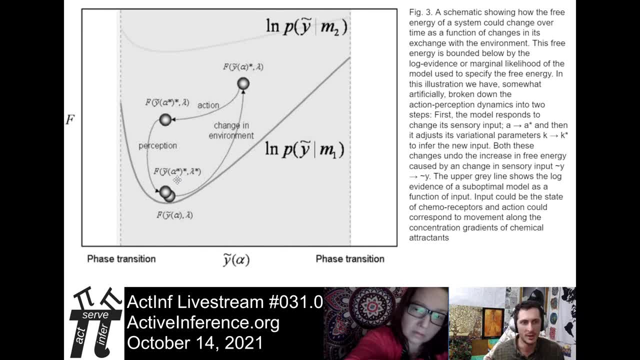 where we're living. So we act and we infer, so that we persist. Any comments here. But it's just a cool like input could be the state of chemo receptors. You know already we're going from these sort of physics formalisms. 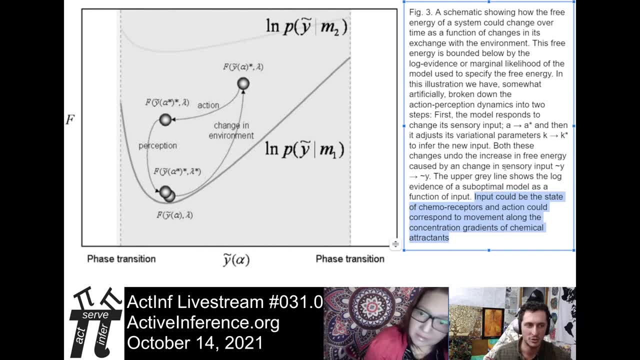 and dynamical systems, formalisms towards just, oh yeah, you know, drop it. It could be like chemical and biological, but was it justified in 2006?? Well, looking back on it, not as much as it is justified today. 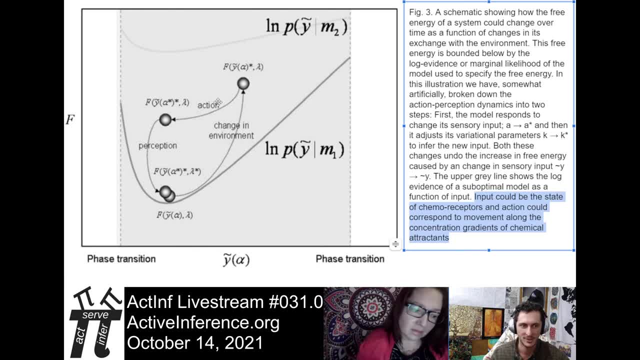 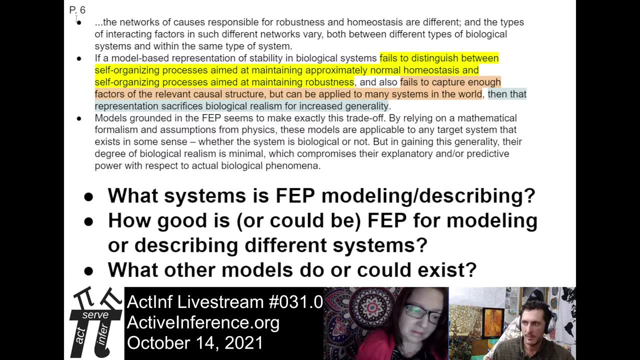 And what will they say in 2033, looking back on this? So all work in progress, Okay, So this is from page six of the paper And won't read the full quote, because we've kind of gotten at this trade-off. 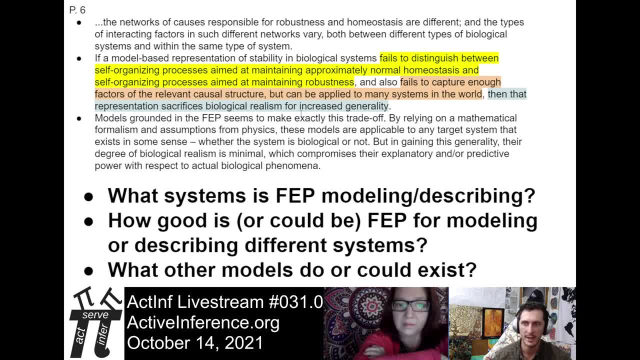 between utility and accuracy and generalizability. But the big questions here are: what systems is the FEP modeling or describing? Where has it been used? Where could it be used, Where shouldn't it be used Or can't it be used? 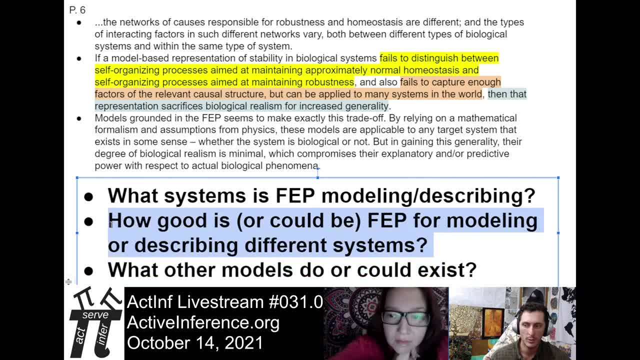 How good is the FEP for modeling or describing these different systems? How good could it be And what would it take to get it there? And then also an important question for those of you who are FEP or ACT-IMP fans and you have a challenging conversation. 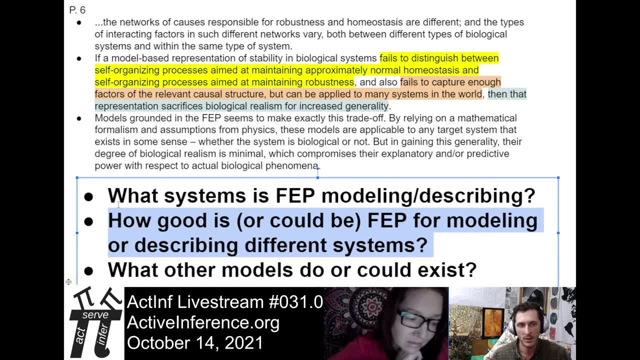 take a step back and ask your colleague: what models do you prefer with similar or different explanatory scope, Just what else is out there? Because it really helps ground the discussion in what that person's understanding or preferences are, And a lot of times people will come up. 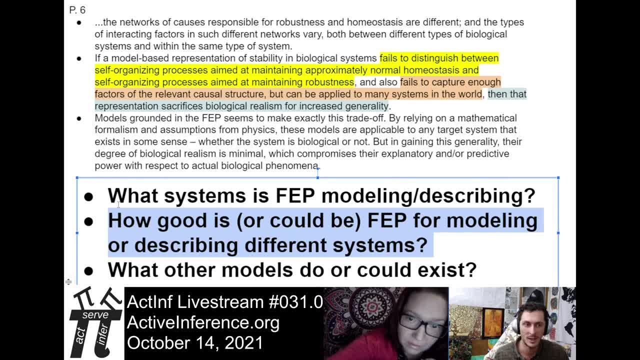 they'll say: I'm critiquing your unified model of perception, cognition, action. Okay, great critique away. That's what I'm doing too. What do you prefer? Oh, nothing. So it helps us stay positive with the contributions that we're making to this field. 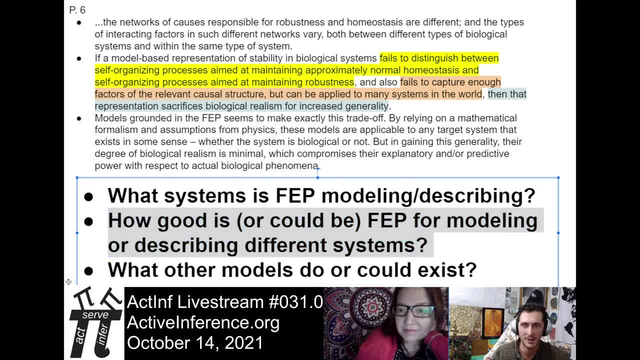 while also recognizing the discrepancy. And that combination of recognizing discrepancy and taking action is active inference. You know this is funny. This is a good contrast to the Sims paper that we just published, And it's a good contrast to the Sims paper that we just published. 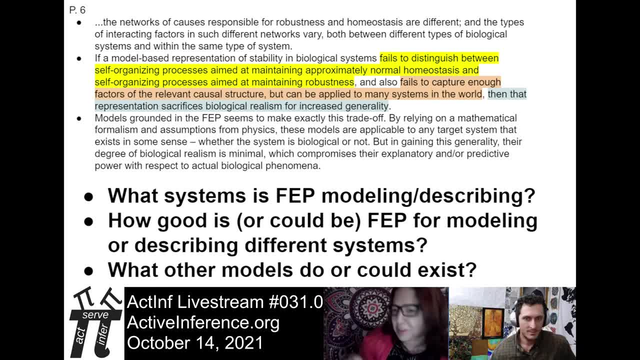 It's a good contrast to the Sims paper that we just published, And I feel like at the end of the last live stream we were just talking about thermodynamics and information theory and the relationship between those two things, But I always want to take the FEP. 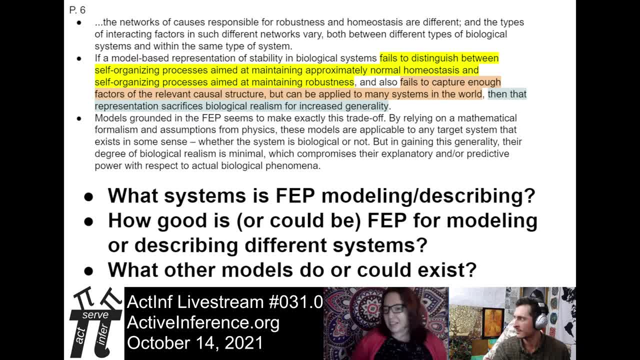 and use it for non-biological systems. I think I veer toward panpsychism more than most people And I have a hard time with the line between mere active inference and adaptive active inference, or the evolutionary late, evolutionary comer late whatever. 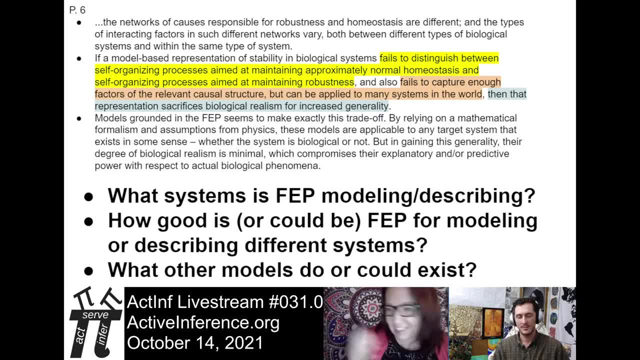 Like, the brain is the ultimate source of cognition and organ-capable cognition, And so would the FEP apply to a set of molecules in a beaker Like? does it have preferences? Do the molecules prefer to be in an equilibrium state, Or how does that work out? 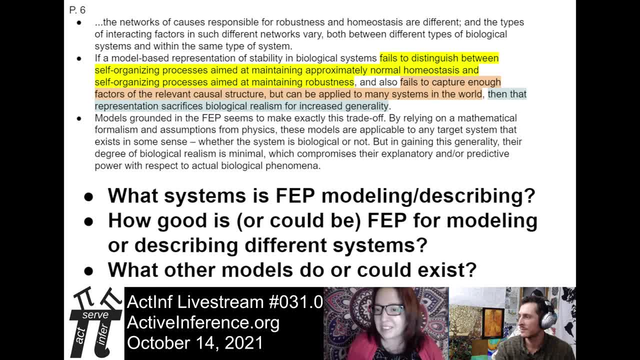 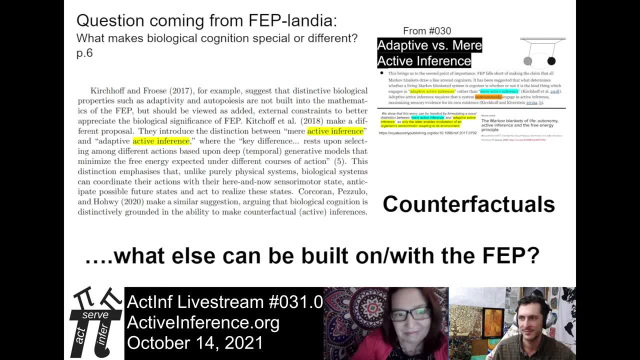 Like I want to take the FEP and use it in systems that maybe it's not designed for. I don't know. I tend to want to go the other way. Makes sense. Here's that adaptive versus mere active inference slide from 30.. 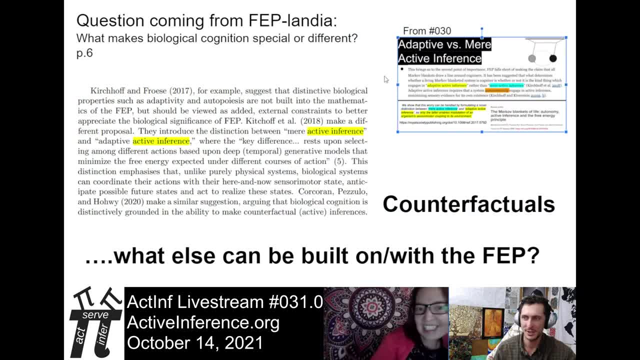 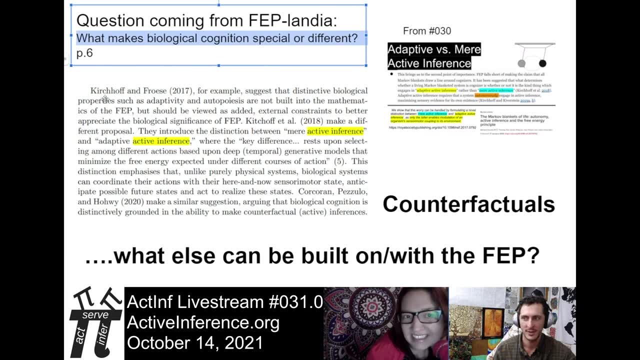 Good segue, Perfect segue, And so here's a question from FEPlandia: What makes biological cognition special or different? So we're not going to go too much into it here. We talked about it in live stream, number 30 a ton. 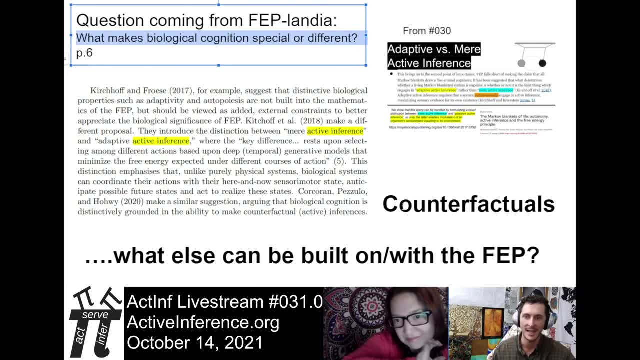 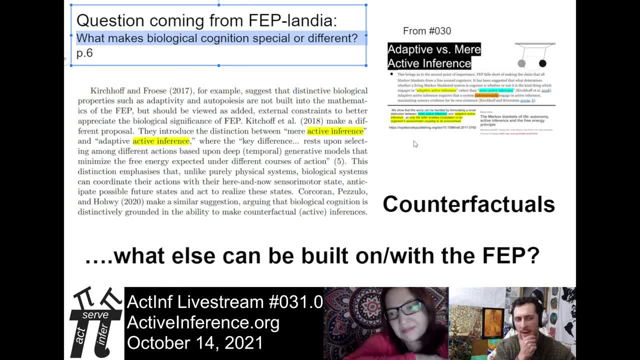 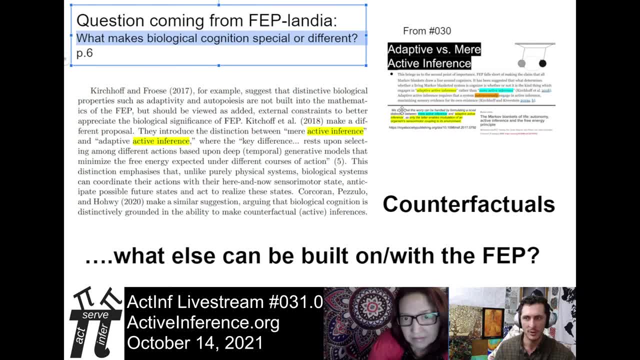 Where does energy dissipation come into play? So these are big questions. What is cognition, And is there just one kind of cognition And biological systems do a special combination of it, but it's different in kind of decimal point, but not in the top level. 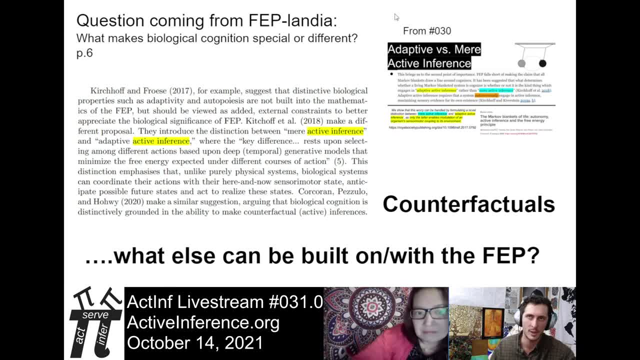 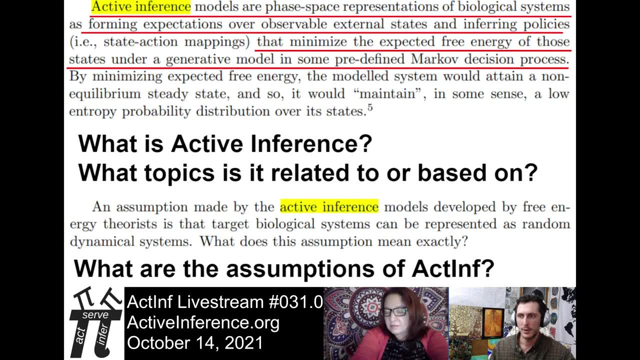 Like: are they or are they really different in type? Or is it such a great quantitative difference that it's different in type? Big questions here. More from the paper: Active inference models are phase space representations of biological systems, So that's like a full stop moment. 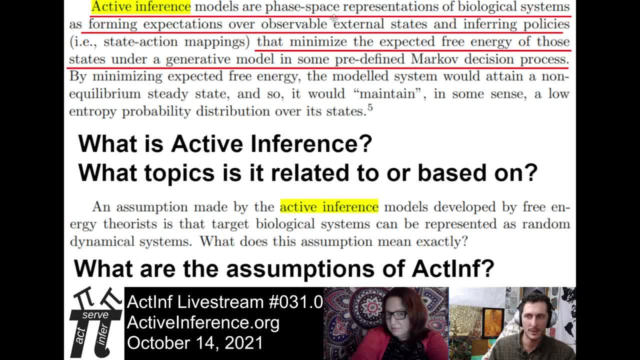 This isn't what biological systems are. It's a phase space representation of systems. Here we're talking about biological systems As forming expectations over observable external states and inferring policies, state action mappings that minimize the expected free energy of those states under a generative model. 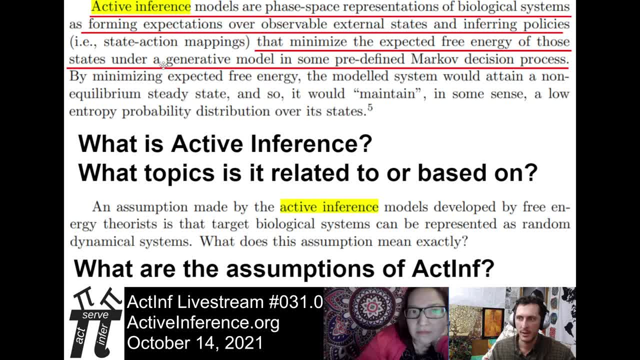 in some predefined Markov decision process. By minimizing expected free energy, the modeled system would attain a non-equilibrium steady state, And so it would maintain in some sense a low entropy probability distribution over its states. So what is that? It's an effective inference. 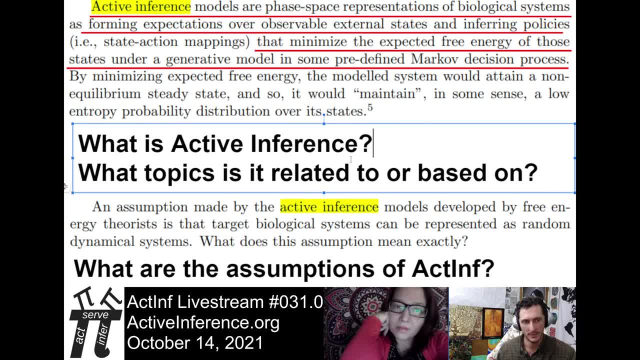 What topics is it related to? What is it based upon? We look at that ball in the bowl and it's easy to say, well, the way, that the imperative that's pushing the system forward is that the ball wants to be as low down as possible. 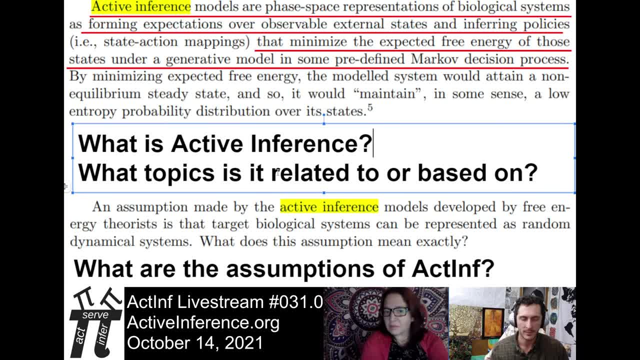 And it's gonna be minimizing its potential energy that way. Another story about the bowl is the ball is going to end up or act as if it's going to end up with the tightest bound through time on how far left and right it goes. 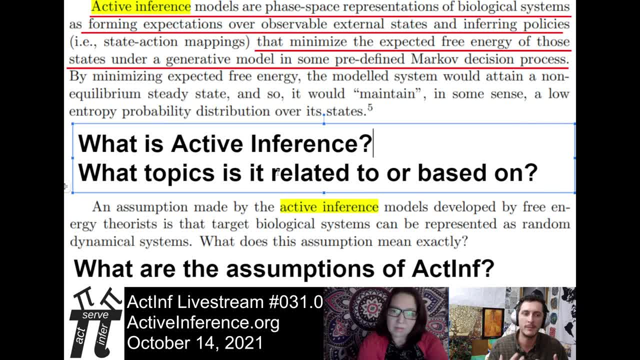 Now that also takes you right to the bottom of the bowl, but you didn't have to mention that you want it to go down. It was just that the desire to minimize the uncertainty led to the bottom of the bowl in that structure. And so how do we think about some of these different ways? 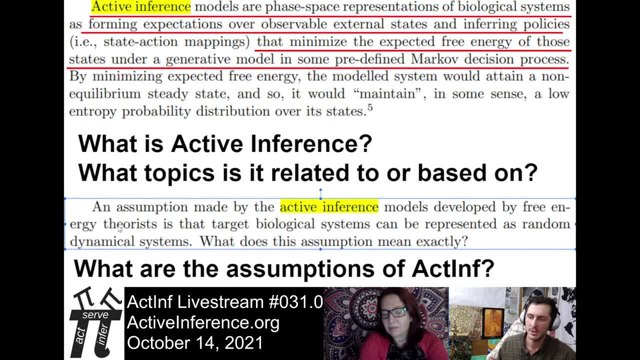 and what are the physics metaphors? And then an assumption from the paper, an assumption made by the active inference models developed by free energy theorists is that target biological systems can be represented as random dynamical systems. What does this assumption mean exactly? 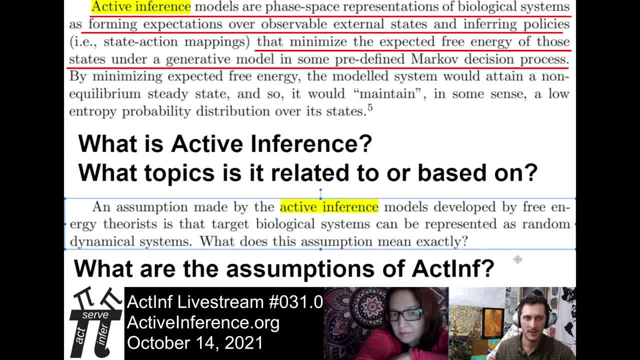 What does it mean And what are the assumptions of ACT-DIMF? What are the assumptions of other frameworks? Does ACT-DIMF have the same assumptions as other frameworks? Does it have fewer or different? Does it have more assumptions? Are there assumptions of ACT-DIMF? 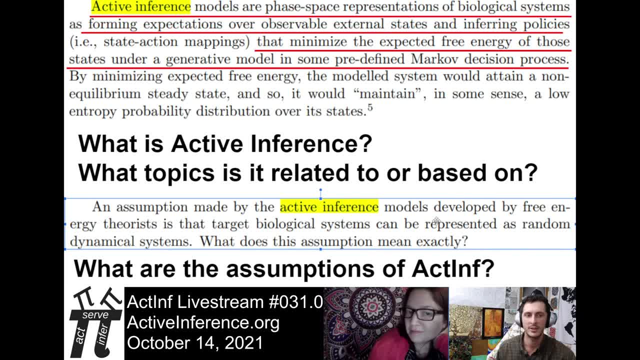 that are consequences of other ideas or vice versa. So these are just awesome questions that the authors are raising and that their work is like a jumping off point into Good Good. So one question that I always have is: what if the so active inference 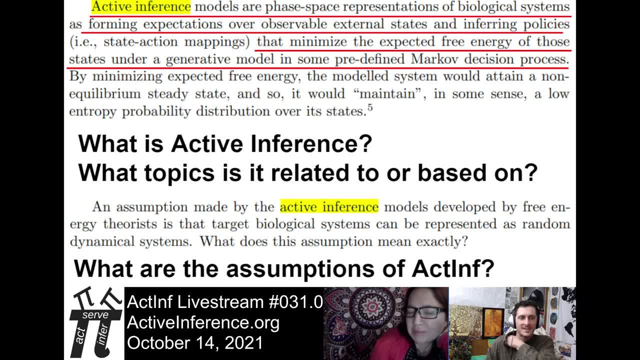 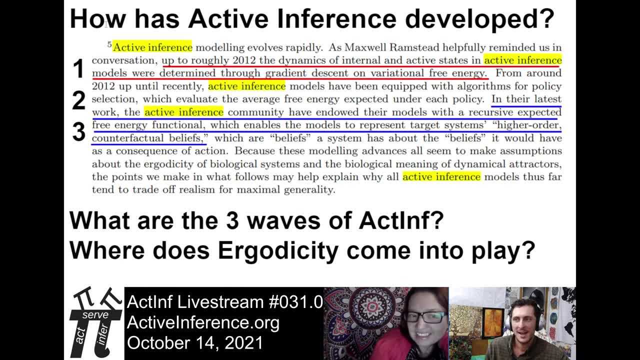 and the free energy principle presumably have the same assumptions, but do they have to? And so that's always something I wonder. How has active inference developed? This is a fun paragraph. Active inference modeling evolves rapidly: Eats, shoots leaves. 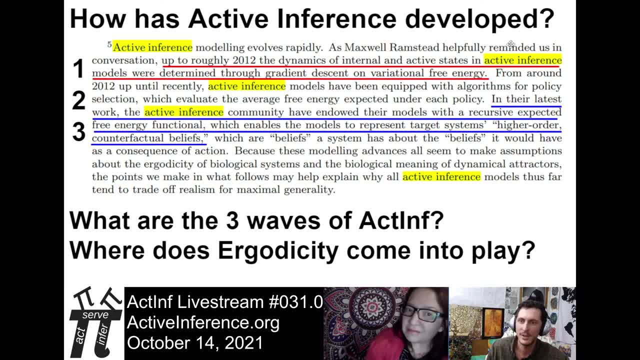 As Maxwell Ramstead. Dr Maxwell Ramstead helpfully reminded us in conversation- up to roughly 2012,. the dynamics of internal and active states in active inference models were determined through gradient descent on variational free energy. So let's call that phase one before 2012.. 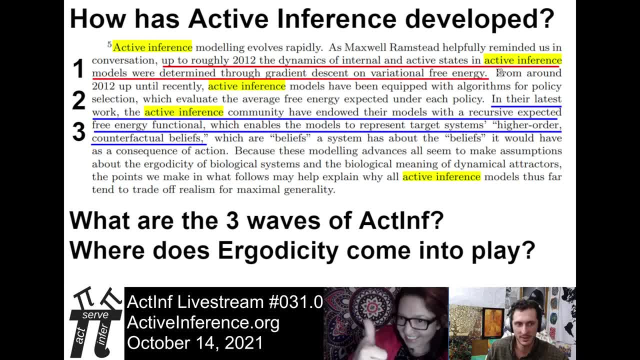 We need a real timeline for this. This is just informal, but this is why we need the timeline: Figure out if we're truly on the best timeline From around 2012 until recently, like 10 minutes ago, or 2019,. 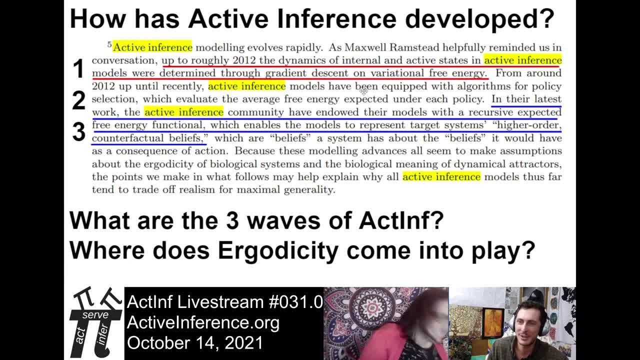 active inference models have been equipped with algorithms for policy selection which evaluate the average free energy expected under each policy. So expected free energy, not just variational free energy. In their latest work, the active inference community have endowed their models with a recursive expected free energy functional. 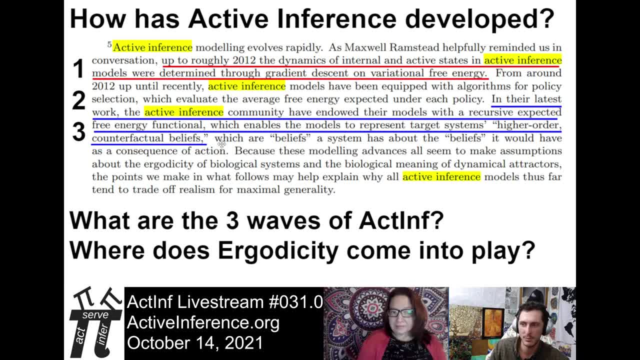 which enables the models to represent targets, systems, higher order, counterfactual beliefs, which are beliefs a system has about the beliefs it would have as a consequence of action. So that's the deep parametric active inference, That's sophisticated active inference. 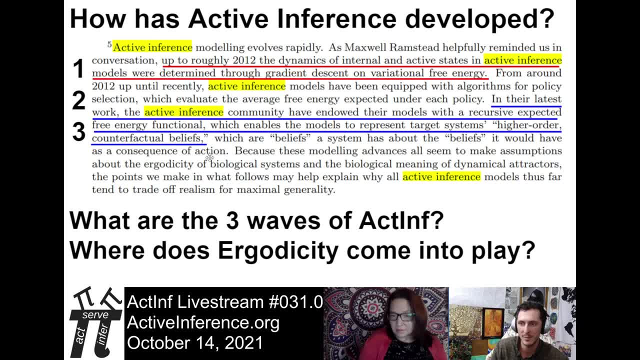 That's what we spoke about with a mental action paper- Sanford Smith et al. Okay, so those are three waves that are important to distinguish in the development of active inference models, because these modeling advances all seem to make assumptions about the ergodicity of biological systems. 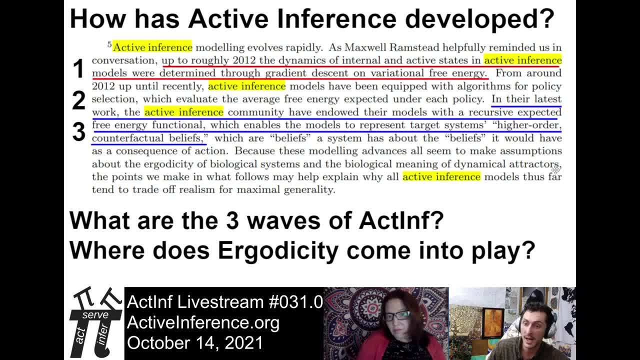 and the biological meaning of dynamical attractors. The points we make in what follows may help explain why hashtag. all active inference models thus far tend to trade off realism for maximal generality. So they're respecting the developments on the framework and encompassing it, summarizing it: 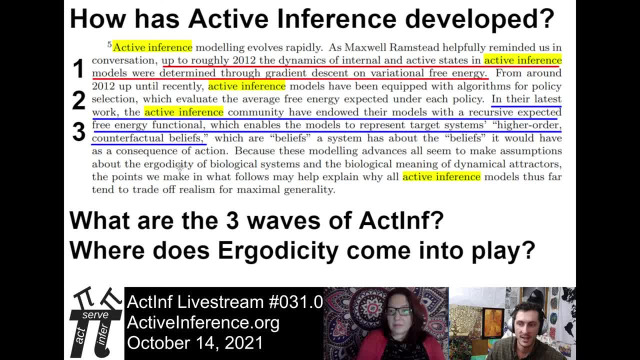 maybe accurately, maybe not, And then saying: because they all make some common assumptions, they're all. they're all making some common assumptions. they're all making some common assumptions. they're all victim to this trade-off of realism for generality, or is it utility for generality? 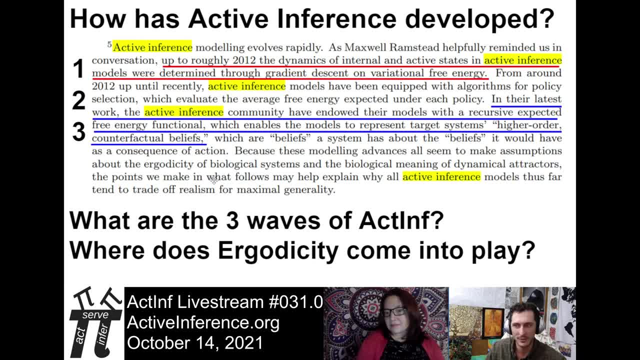 Which one was it again? Realism, utility. What are the trade-offs? So? what are the waves of active inference? How does ergodicity come into play in these different waves? So I know there's a lot on there, but this is really an important piece to understand. 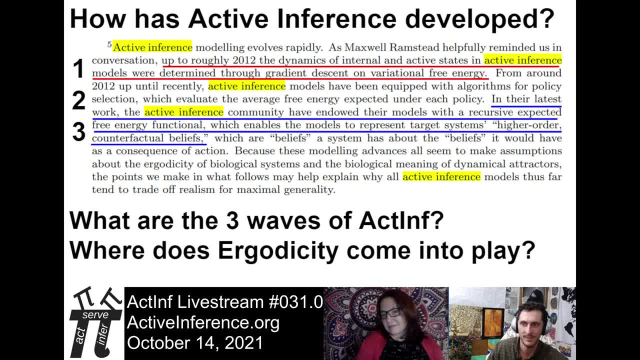 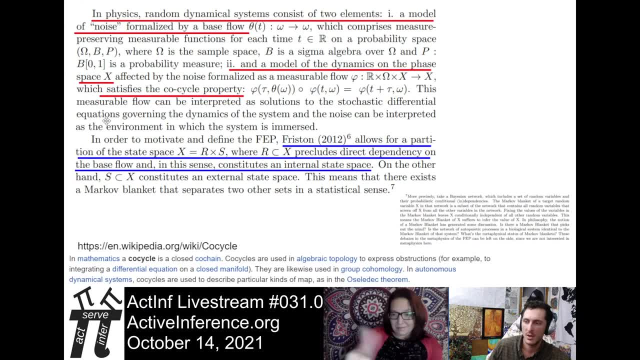 that there's been recent developments. There's been a lot of work done on this, but there's been a lot of work done on this and I think it's still in progress. So, yeah, it's still in progress. Okay, here, this is some technical details. 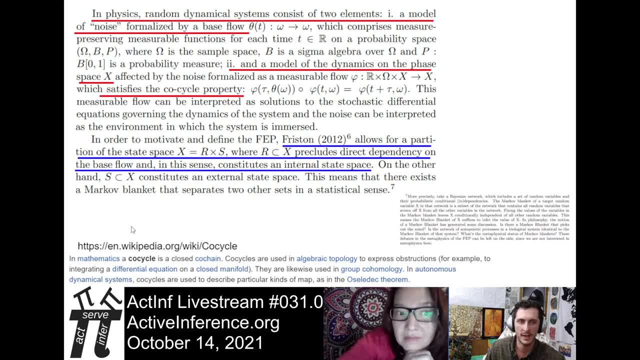 that it'd be awesome to just learn more from the authors or from anyone else who sees this and gets excited by it. This is about some of the physics formalizations of noise and dynamics and phase spaces, And just a term that I was curious about. 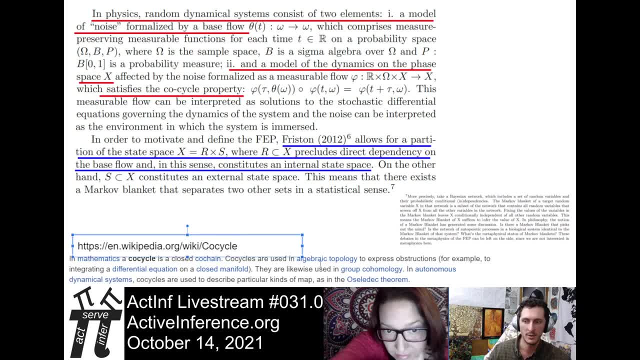 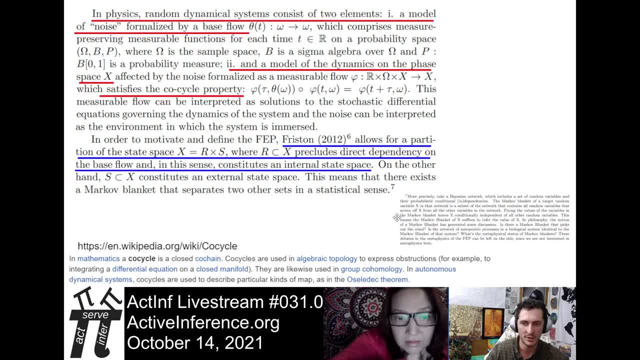 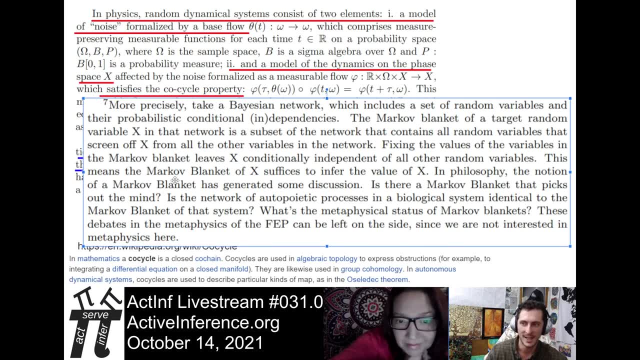 to some other ideas like a co-cycle, But these are just things to learn and discuss about. And then this is sort of the classic Bayesian network Markov blanket. Is there a Markov blanket that picks out the mind? Is the network of autopoetic processes. 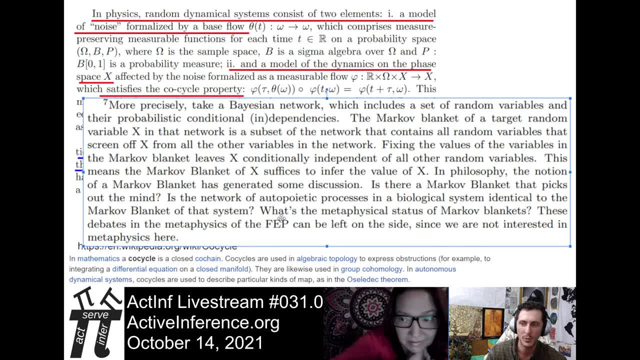 and biological systems identical to the Markov blanket of the system. What is the metaphor? What is the metaphysical status of Markov blankets? And then the author's right? These debates, in the metaphysics of the FEP, can be left on the side. 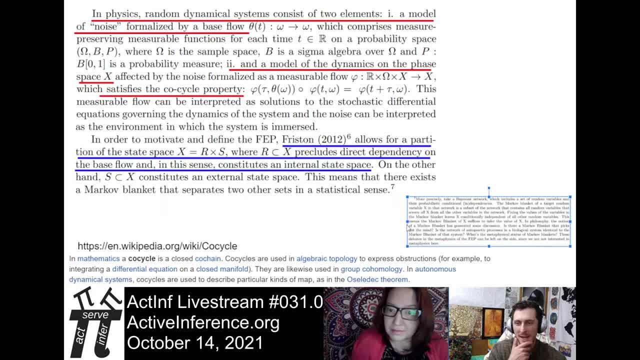 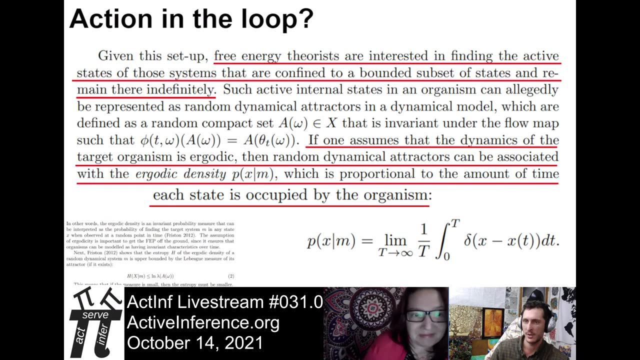 since we're not interested in metaphysics here. Hmm, I thought we were having a discussion that was meta to physics, So where is your metaphysics now? Okay, anything else there? Action in the loop. Given this setup, free energy theorists are interested. 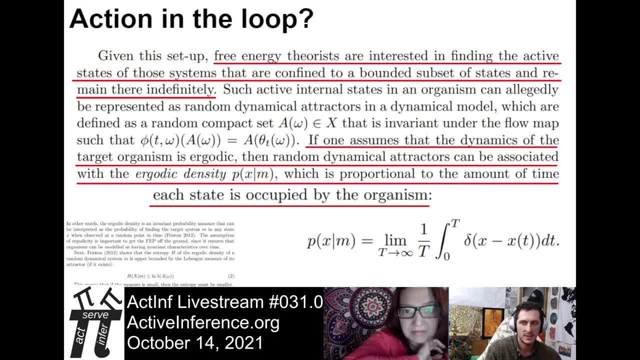 in finding the active states of the systems that are confined to a bounded subset of states and remain there indefinitely. So we wanna have our internal states be at a certain level, like thinking about our temperature being at a certain value or anything else. And now we wanna talk about the control theory question. 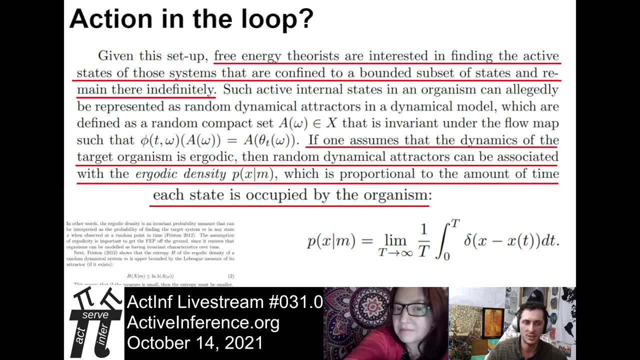 which is what active states should the system engage in, conditioned on internal and sensory states, such that the internal states do remain bounded within a subset of states? More technical details: If one assumes that the dynamics of the target organism is dynamics is ergodic. 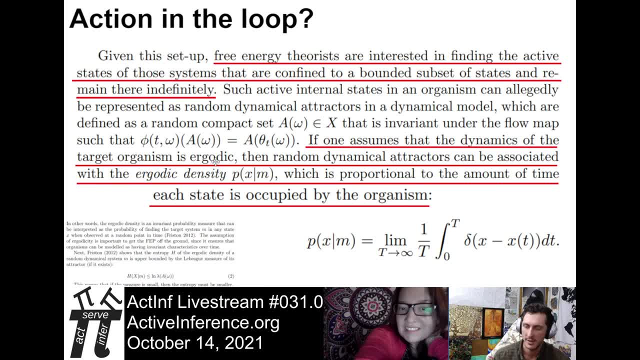 If one assumes that the dynamics of the target organism is ergodic, It's grammatically incorrect. If one assumes that the dynamics of the target organism are ergodic, that's why you can't read it, That's why the compiler failed Then- That's it. 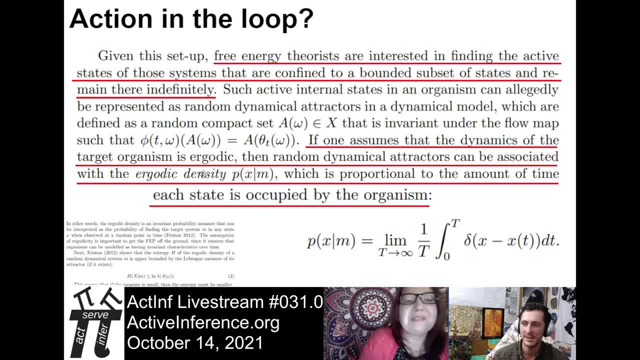 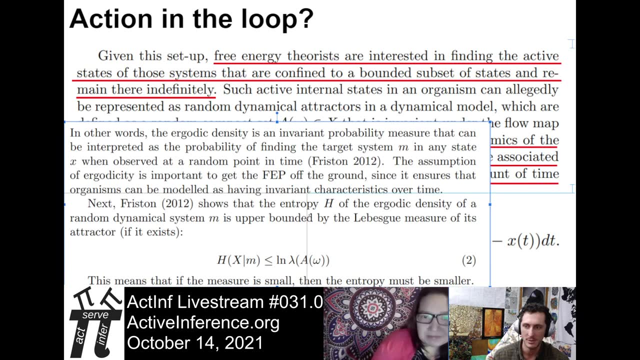 Random dynamical attractor- can be associated with the ergodic density: a P distribution of X given M, which is proportional to the amount of time each state is occupied by the organism. So here's where we return to their definition of the ergodic density as the invariant probability measure. 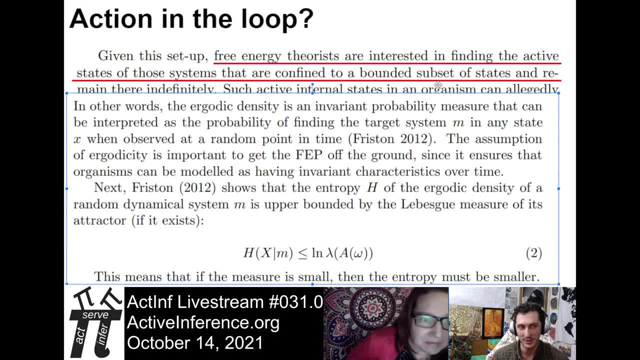 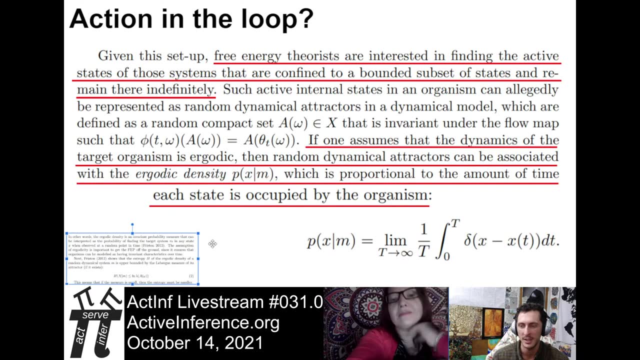 There's a few other terms that I know some listeners know about. whether they'll help us with it, it's another question. but what does it mean to talk about the, the Lebesgue measure of the attractor? How is that connected to dynamical systems and entropy? 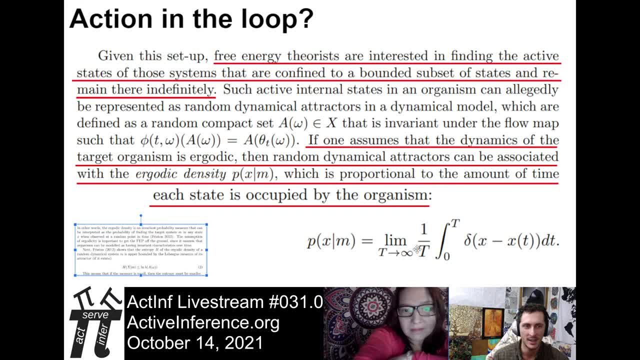 and whatever this integral is calculating in the limit of time approaching infinity. But this is kind of this thing that we see in space and in time like one over space, So like what's the tiniest infinitesimal space for all space, or what's the tiniest? 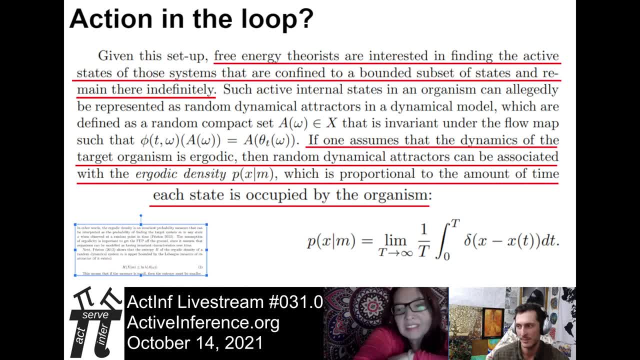 tiniest moment for all time. How does that connect to action control theory? More on that later, but here, even in this, even in this slide, it raises the question. So here it says: such active internal states in an organism. 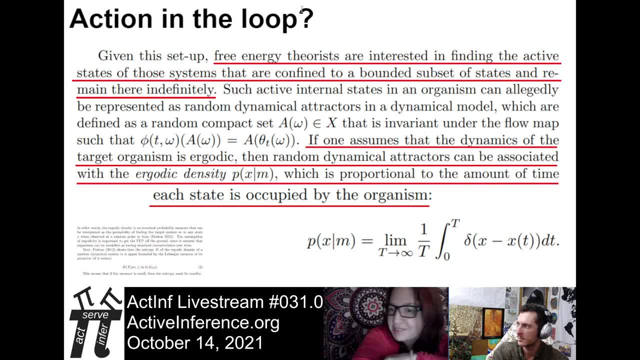 And so maybe it's the way that the diagrams are usually drawn for active inference, but I don't ever think of active states as internal states, Like there's active states, sensory states, internal states, external states, And I always think about the sensory. 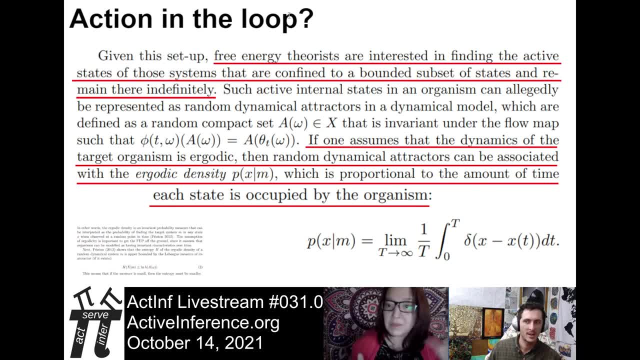 the active states as the on the boundary between internal and external. so absolutely there um are internal, external, sense and action states. so what are the active internal states? there's a few ways of thinking about it. the particular states are the sense, action, the blanket states and the internal states. so maybe that's what's being referred to, or we can well. 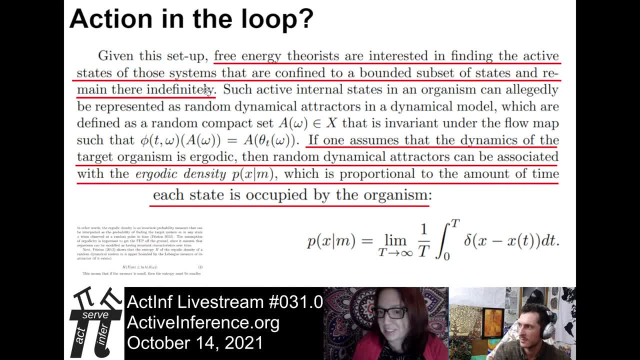 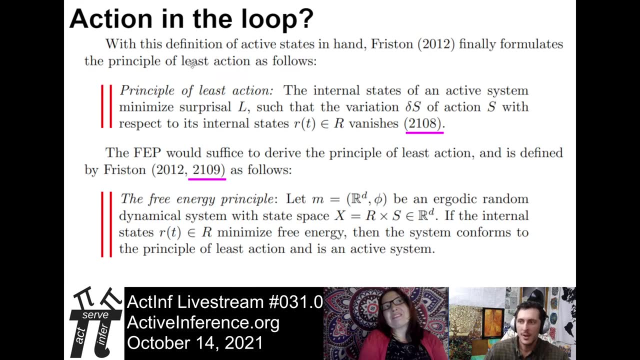 when we're talking about mental action, i guess then the active states are internal, yes, between the past and the future, but still internal, right, like in mental action, right, yes, with this prince, with this definition of active states in hand. so i believe that we're now working. 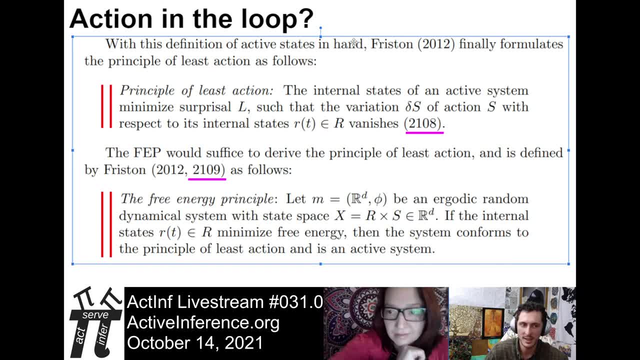 with the friston ontology of action being not the internal states, but who knows first in 2012- finally formulates the principle of least action as follows: the principle of least action: the internal states of an active system. so that wouldn't be the action states, that would be. 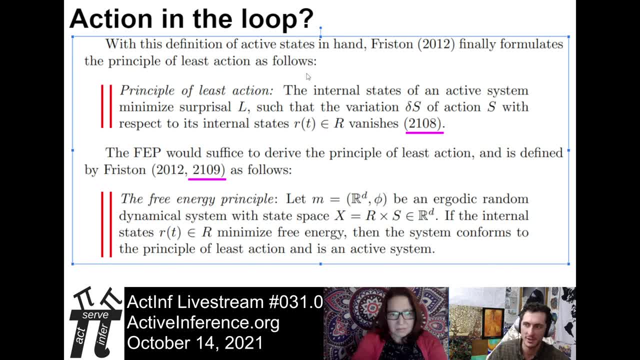 the internal states of a system with on the interface having action. they minimize surprisal l such that the variation delta s of action s with respect to its internal states, r of t existing in r, vanishes. and then classic future friston. look at that, the 2100s are going to be just so. 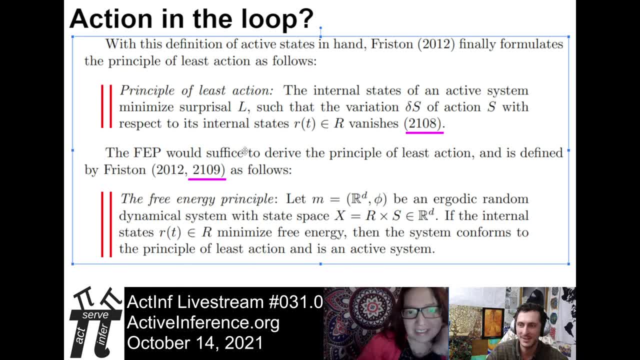 good. the fep would suffice to derive the principle of least action and is defined by friston in the past and the future as follows: the free energy principle, technical, technical, technical. if the internal states minimize free energy, then the system conforms to the principle of least action. 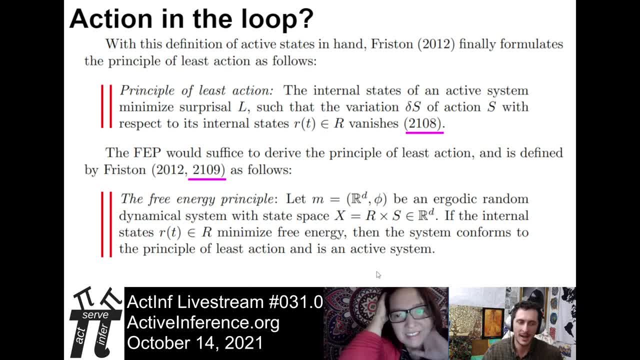 and is an active system. this will be good to to unpack and learn more from the authors, as well as from those who study these areas, because it's sort of something we all ask is like wait least action, but then they're engaging in action. couldn't they just do less action? wouldn't that be more of a fulfillment of the least action? 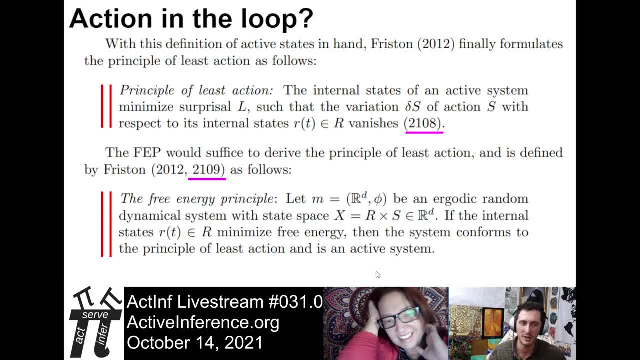 principle, but what is it actually? it's like a stationary principle, it's an invariance, so there's a little bit more nuance than just staying on the couch. and i haven't heard this term active system before. i've heard like active inference system or inactive. 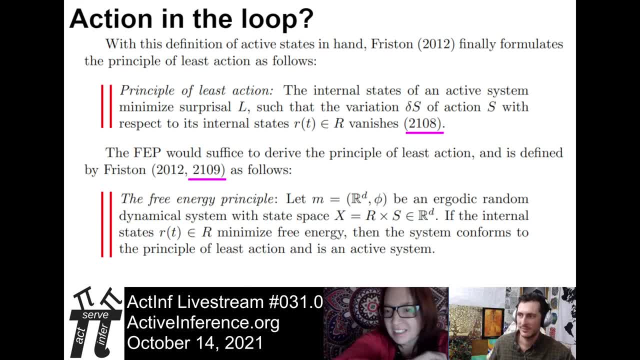 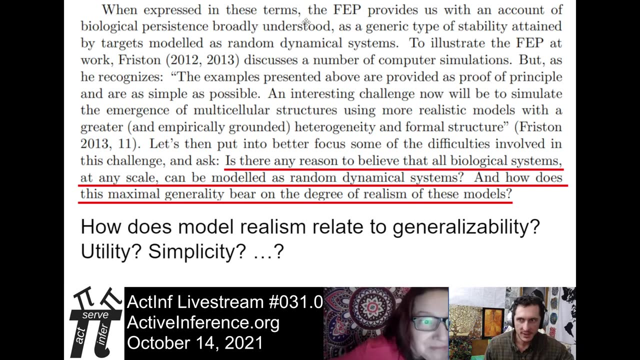 system, but this active system is is new to me, and indeed friston was a very forward-thinking guy. uh, is a very forward-thinking guy all the way into the 2100s. um, when expressed in these terms, so in the terms of physics, the fep provides us with an account. 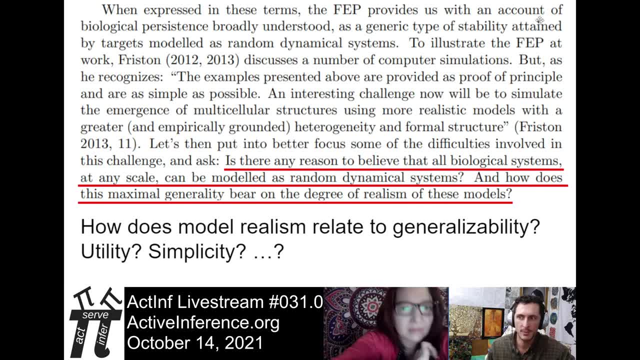 of biological persistence as a generic type of stability of random dynamical systems. so then they talk about, first, in 2012 and 2013, some simulations, and then here's what the author's challenge is, and say: let's then put into better focus some of the difficulties involved in this challenge and ask: is there any reason? 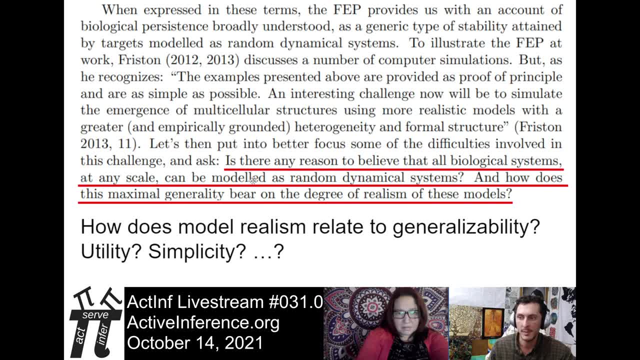 to believe that all biological systems, at any scale, can be modeled as random dynamical systems. and how does this maximal generality bear on the degree of realism of the models? so we had a few previous discussions ago. we had um, we had realism, we had utility, we had instrumentalism, we had all these different axes, and how are we going to? 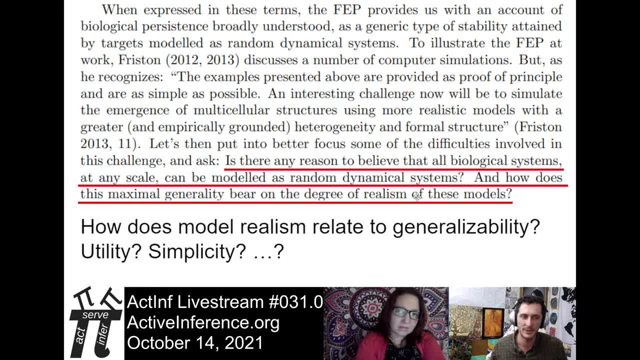 manage that trade-off, because sometimes the most- quote- realistic description of a system isn't the most useful or it's not the most general. so there's a lot of trade-offs happening. how does model realism relate to generalizability and how does that relate to the utility of the 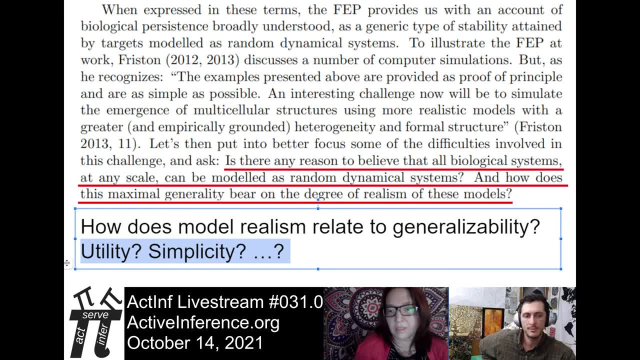 model as well as other attributes like its simplicity. that's like the relationship between the map and the territory- if you wanted territory then you wouldn't need a map- yeah, and then, almost like the compass, um, or a piece of paper that just you know, says like you are here, it's like it's so General, you can always look. 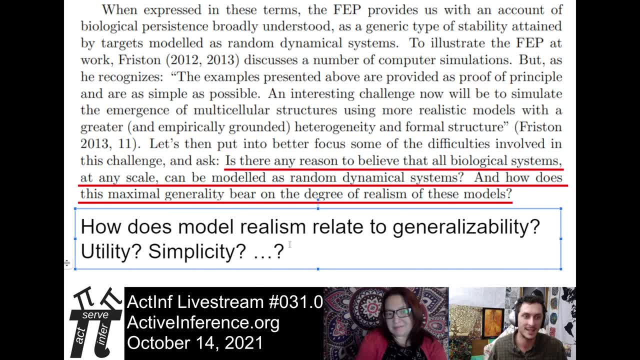 down and that map is going to be at least not telling a lie. you know, this is your left, or something like that. this is, but is that useful? it generalizes really well, but have we lost this question of navigation in the desire to find the simplest map? so something that I wonder about, like 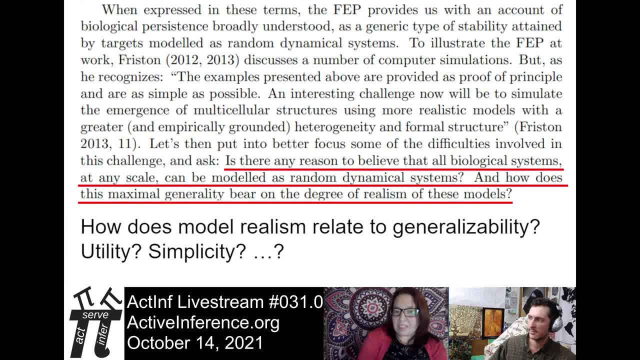 um, you know, our biological systems, random dynamical systems, like what's a non-random dynamical system? like a dynamical system, as opposed to like a static system, like statics, dynamics and so like. what other system could a biological system be like if it, if it's not a? 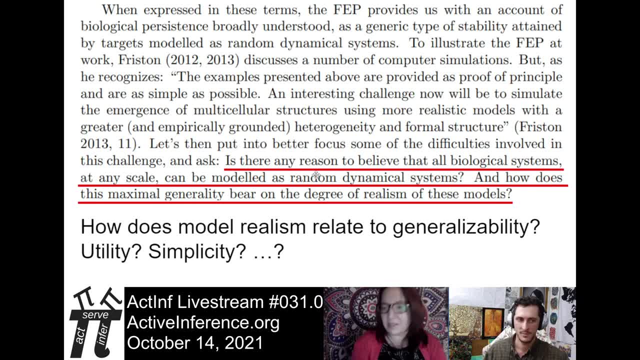 random dynamical system? it's not a random dynamical system. it's not a random dynamical system. what is the alternate hypothesis, just like what you said about like okay, well, what is the better model for cognition? if not, you know, active inference, then what model is the better model? 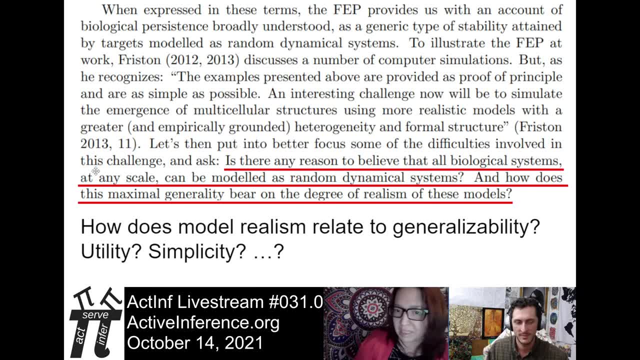 right like so. but what about for a biological system if it's not random dynamical system? what is the best model for a biological system? yes, dynamical through time dynamics, random, used in a lot of different ways. but is that statistical? is it stochastic, whereas determinism? 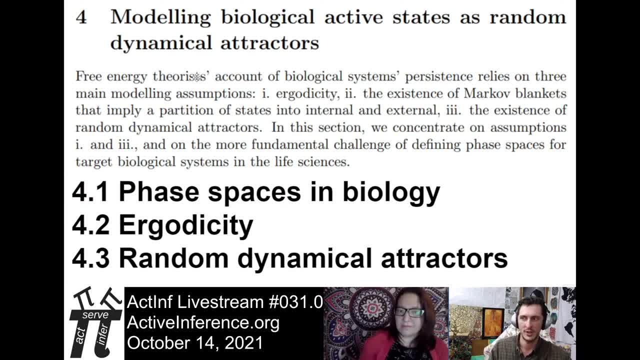 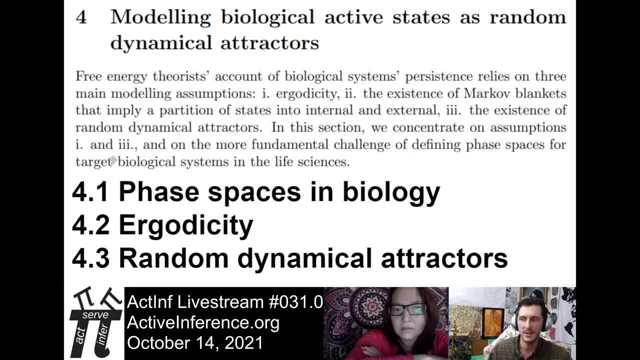 three and on the more fundamental challenge of defining phase spaces for target biological systems in the life sciences. So the three core ideas that they're saying are underlying FEP work in biological systems are ergodicity, Markov blankets and random dynamical attractors. 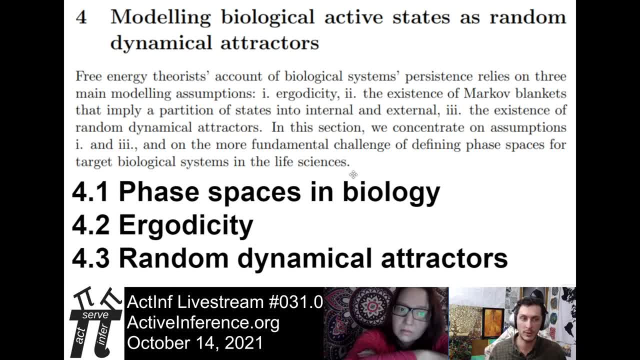 Are those the main three? That's a really important question. This paper is going to focus on the first and the third, not going as much into the Markov blankets discussion, because there's been a huge amount of discussion on Markov blankets and we've talked about them. 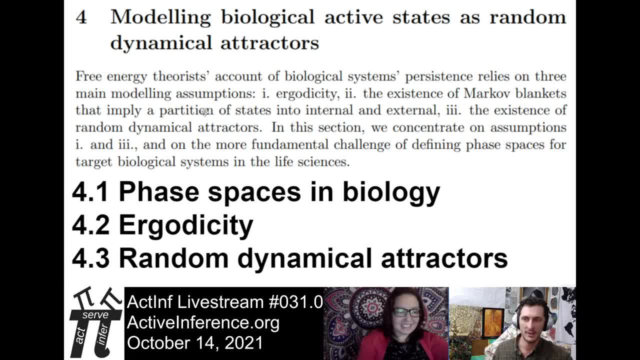 severally. So they're going to focus on ergodicity and random dynamical attractors. That's 4.2 and 3, but that's going to be interesting. This is introduced by discussion on phase spaces in biology, So that's what the authors. 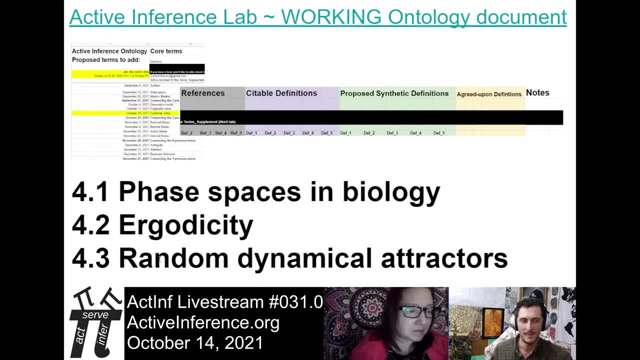 have set out to do Now, shameless lab plug. we're working on an active inference ontology in a participatory way that includes references, definitions, translations into multiple human languages. It will be many things and it will scaffold educational content that will. 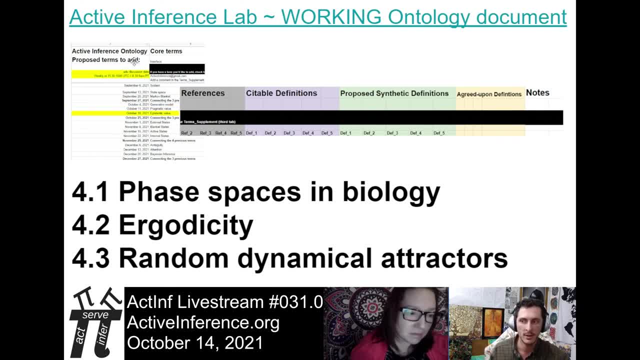 make this entire field more accessible and rigorous. So terms like phase space we've talked about. we talked about state space on September 13th. So every week we're bringing together different perspectives and sharing resources and working towards common understandings. in this document to really get at what are the core assumptions. 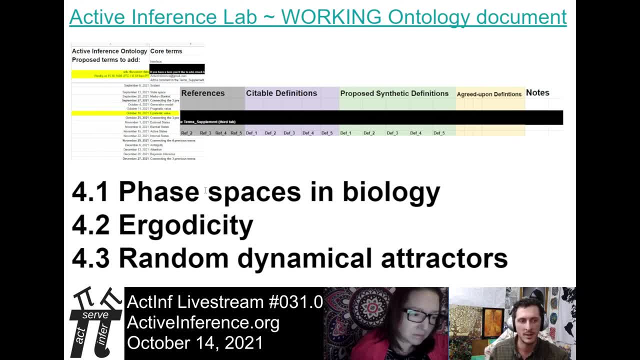 of FEP or ACT-INF. What do these terms mean? What would somebody need to learn if they wanted to understand more? So it's really important work and we're definitely going to draw upon the authors' contributions here as we work to scaffold an active inference ontology so that 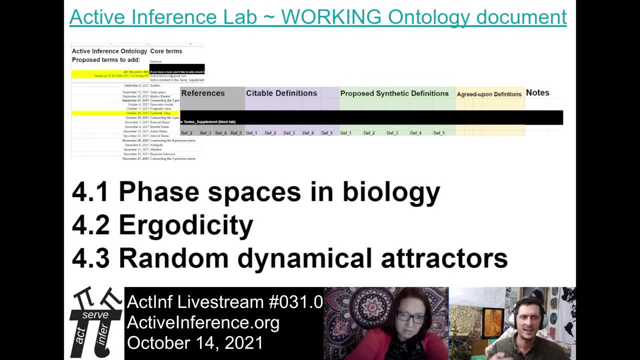 we don't get tied up in active state action, state systems with action. We can be clear about how we're talking about this field And in fact we really have to be Anything on our ontology document before we continue back to the paper. 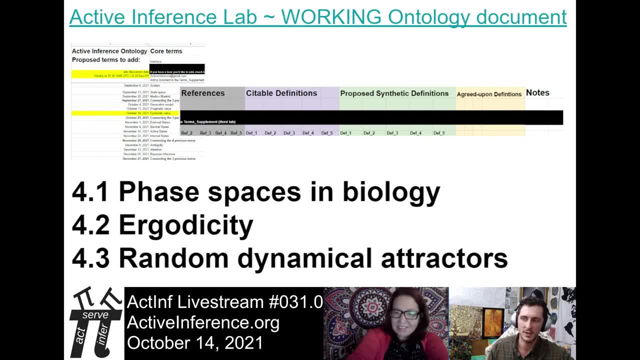 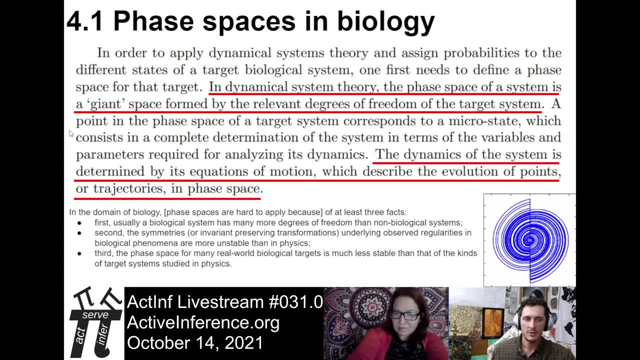 Okay, But this has been a fun project with many contributors. So let's talk about phase spaces in biology. Right, we introduce this in the earlier keyword section. So the phase space, the system, is a giant space formed by the relevant degrees of freedom of the target system. 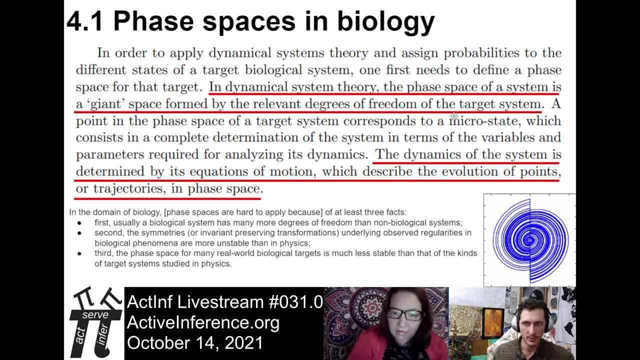 What is it? e, Six bridge sections, and then that's the space of the possible, a point in a face- face corresponds to microstate, which completely determines the system in terms of the variables and parameters required for analyzing its dynamics. And the dynamics are determined. 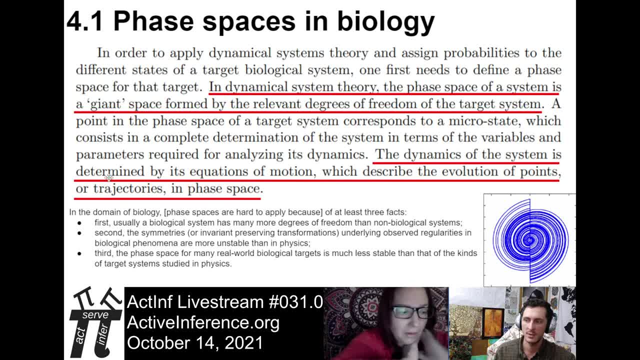 by the equations of motion which describe the evolution of points or trajectories in phase space. So here's that phase space kind of model, and then the authors are going to suggest that there's at least three facts, cold hard facts, that make phase spaces. 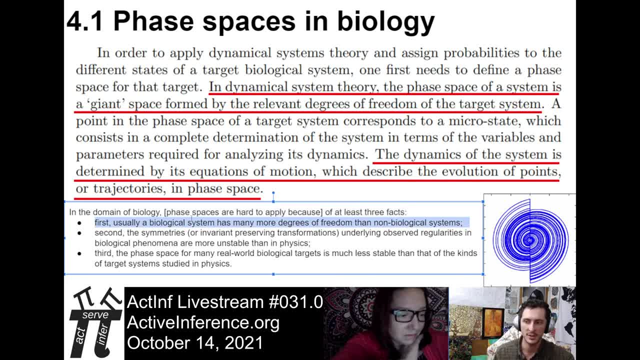 in biology hard to apply because, first, biological systems have many degrees of freedom, It's not just a pendulum. Second, the symmetries which are invariant, preserving transformations underlying the observed regularities in biological phenomena, are more unstable than physics- Okay. And third, the phase space for many real-world biological targets. 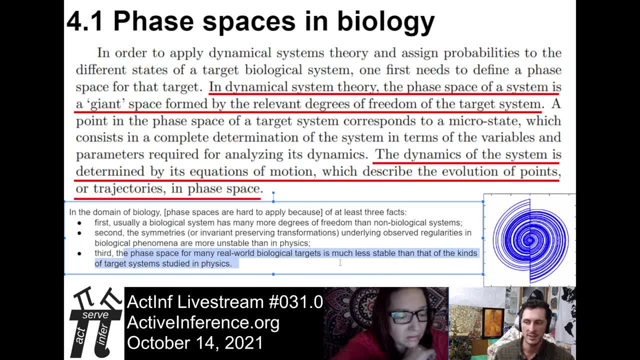 is much less stable than that for the kinds of target systems studied in physics. So what do you think about that? or about phase spaces in biology? Yeah, I mean, I think I mentioned the multidimensionality in the beginning when we were talking about the phase spaces in biological systems. 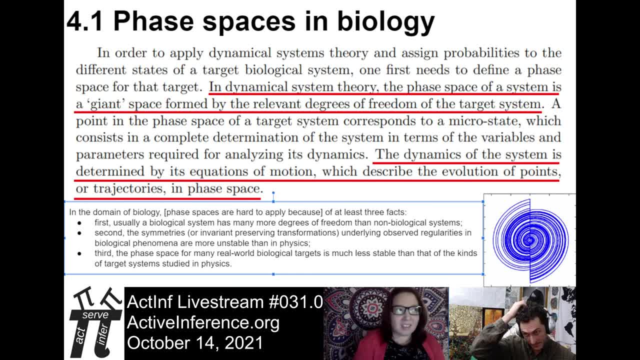 And I think that it just comes to that with any system, right, Like you can always include too many parameters, Like you can have the territory or you can have a dramatically reduced map, And so finding that correct balance is hard. And if we're looking at, you know, say, states of a system and 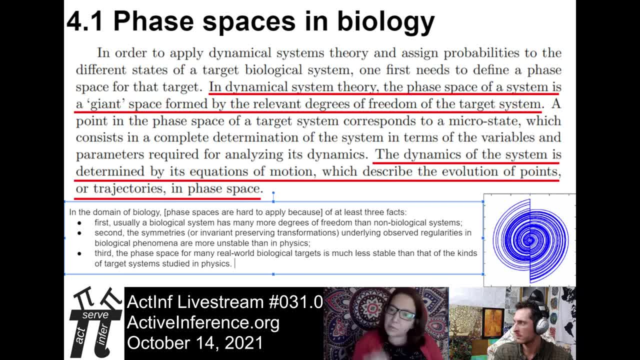 trying to predict the next state. aren't all of the factors conditionally independent? Is there some you know mingling of the variables There? And is it okay to just model a couple at a time? And what if we don't know? if there are some, 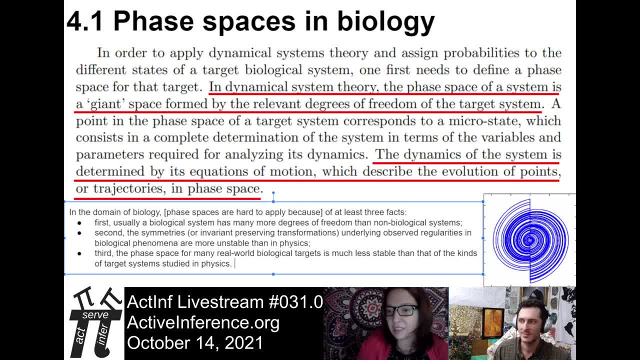 confounding variables in the system too. So it's it's a difficult task, but it's. how do we start to get a grip on it as hard? Yes, And a big question in the background here is: does this matter for? 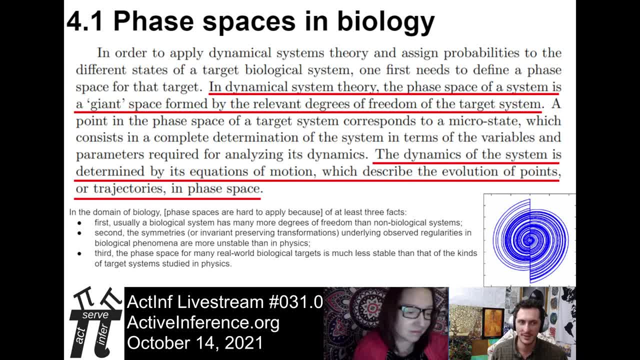 applications. So, yes, these are in principle critiques of doing dynamical phase space models of biology, But we know that, you know we're not going to be able to do that, We're going to have to dynamics which was models of neural systems, of hormonal systems, of ecology. These are all really 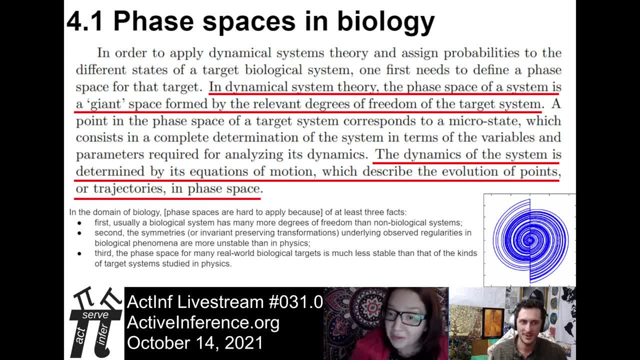 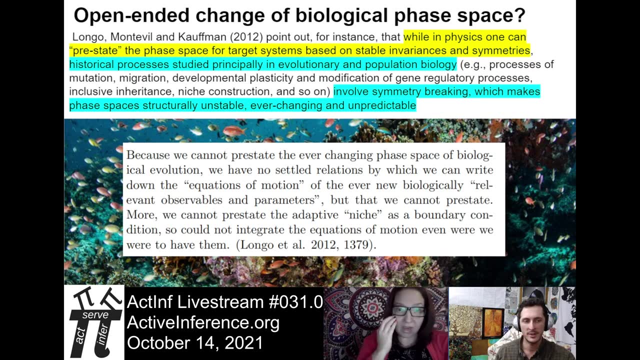 useful and people use them every day. So, Jane, regulatory networks, don't forget those. How can we forget? but does something having these sort of fundamental critiques prevent it from being useful? Not always. This is a really nice points about the open endedness of biological phase space. So this is the work, and I have been doing this a couple of years now. It was actually a really nice and fun project I did. I just found out that there's so much information in that And I have been doing a ton of thinking about that. I have been doing a lot of research. I have done a lot of 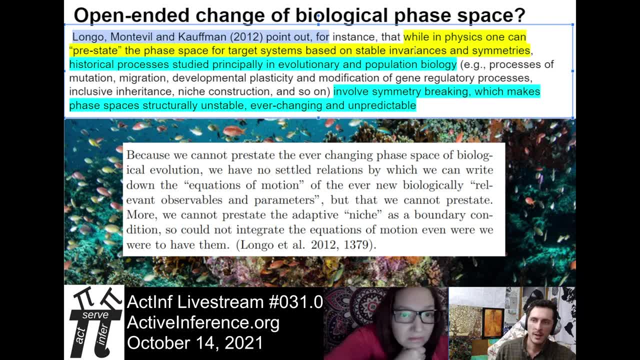 research on that. I have been doing a lot of research, I have been thinking about this, But somehow it was so hard for me to even. Vlango Montvale and Kaufman 2012,, who said that in physics one can pre-state the phase. 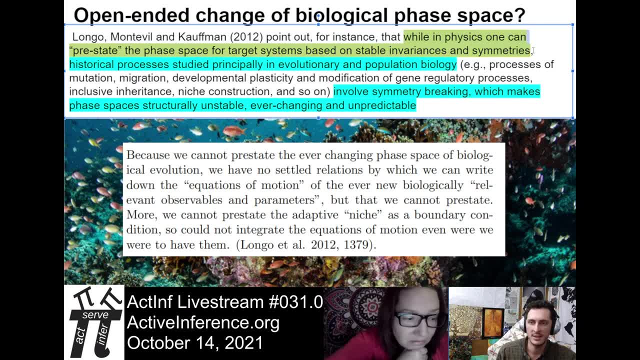 space for target systems based upon stable invariances and symmetries. So we can like say: the ball is going to be rolling around in the box. Those are the boundaries and here's the invariances. Historical processes studied in evolutionary and population biology. 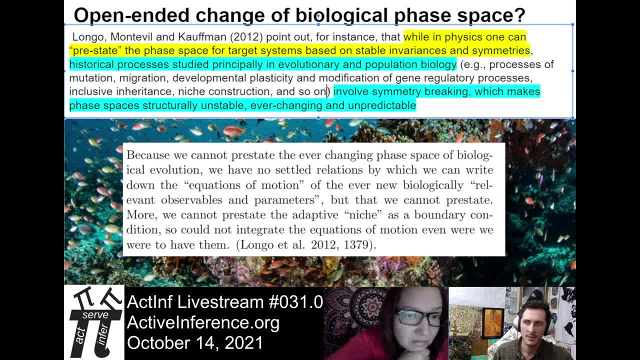 like all these processes that we know and love in biology involve symmetry breaking, which makes the phase spaces structurally unstable, ever-changing and unpredictable. Now, unpredictable is a little bit of a tough one, because that's a continuum. What if you can? 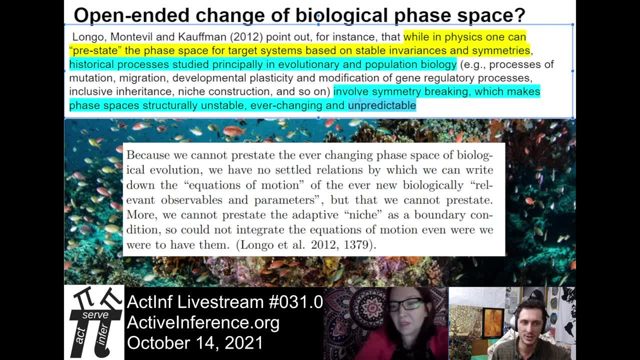 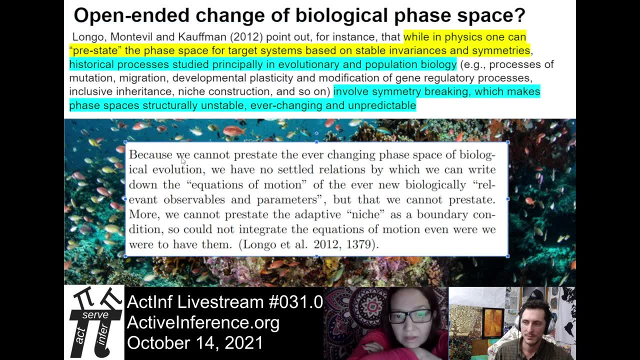 predict one percent of the variance in great evolutionary transitions. Is it unpredictable or is it predictable? You know, is it half full or half empty? And then this is from the paper, because we cannot pre-state the ever-changing phase space of biological evolution we have. 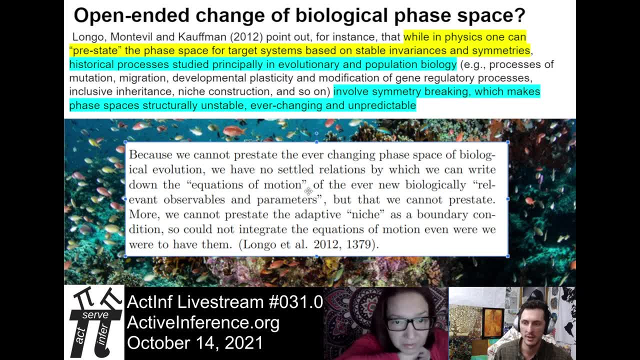 no settled relations by which we can write down the equations of motion, the ever-new biologically relevant observables and parameters, but that we cannot pre-state More. we cannot pre-state the adaptive niche as a boundary condition, so could not integrate the 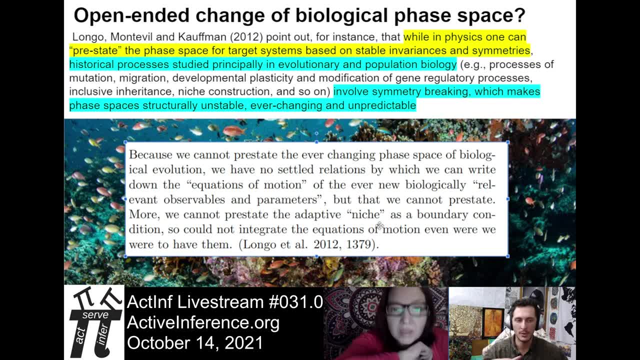 equations of motion, even were we to have them all. So it's like there's the ball rolling around on the billiards table, but now there's mutations in the genome of the ball, so that there's like totally new mechanisms arising in a way that might have a historiosity. Oh yeah, and the table is. 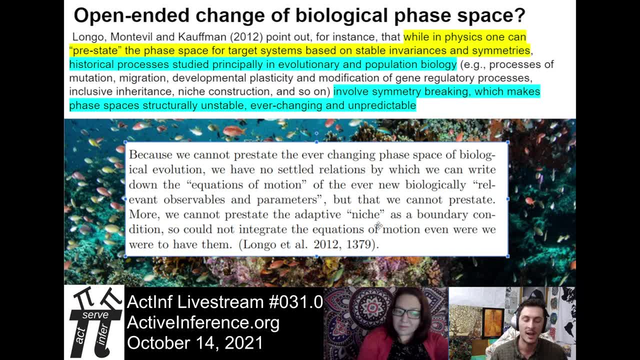 mutating and it's made up of other organisms. So it's easy to see we get lost in the complexity. yet adaptive action exists and useful models exist. So how do we reconcile the fundamental open-endedness and creativity and novelty of evolution with our desire to explain some portion of the variance so we can act effectively? 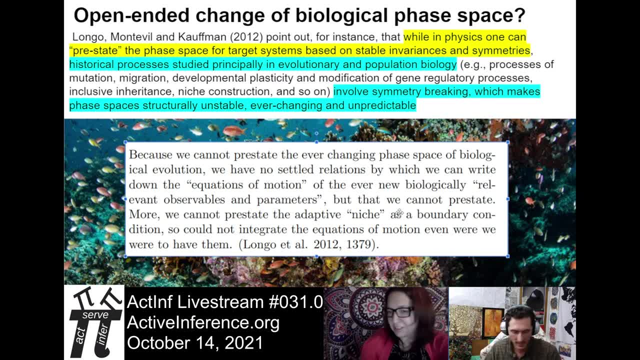 Well- and this relates like to a question that I had brought up to you yesterday, Daniel- I think about like what about discretizingSpace, And so I know that some of the physics principles rely on infinite time, like the Ergodicity relies on the possibility of infinite time, and this is all stuff that's like kind of beyond me. 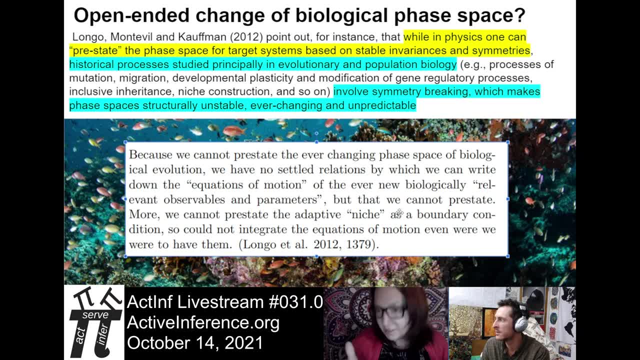 but. but what if we have a temporarily restricted moment, right, like what if we're just interested about now and five years from now? or what if we're just interested in now and five years ago? right, and and so in each moment, is this symmetry breaking happening, or at what scale? and so is. 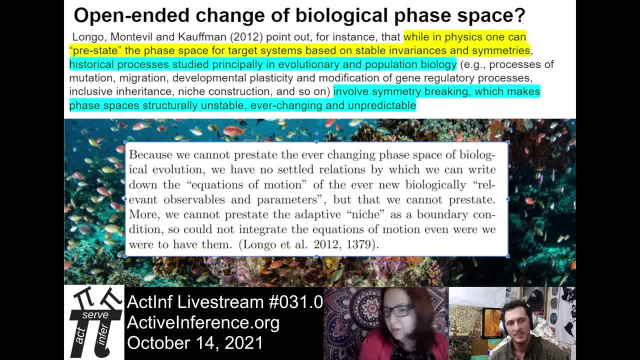 there perhaps a chunk of time, a small, discrete chunk of time from, you know, a microsecond to 100 years, where these types of inferences can be used and where the equations are applicable and where we can use the model with, under the, you know, specification that this model is not. 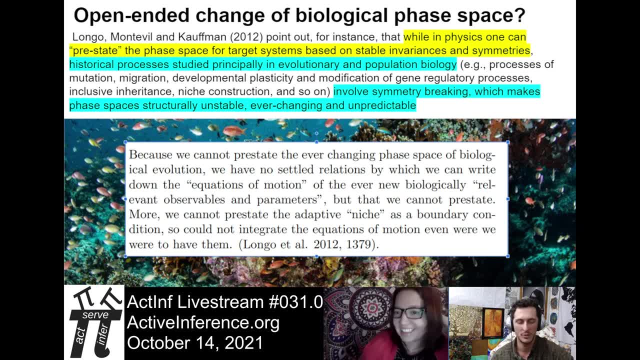 good for the next two million years, but it will last you 20, right like so. it's a model of the phase space of blood glucose versus ph in a person as measured by the devices we have. it's not of blood sugar over a million years, because that doesn't even make sense given the system of 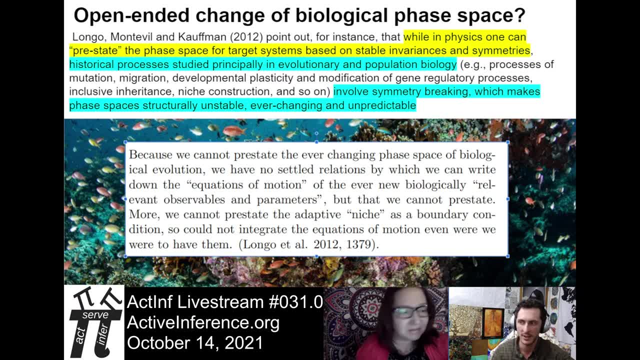 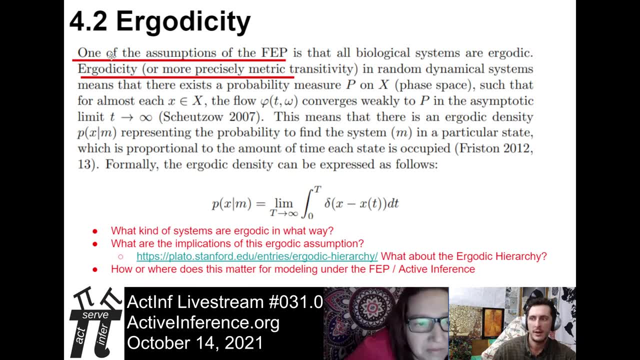 interest. so how do we do that? we reconcile pragmatics and utility with these really important philosophical questions. so that was four one phase spaces. word two: ergodicity. one of the assumptions of the fep is that all biological systems are ergodic, so paging ramstead at all at all. this is something we really want to. 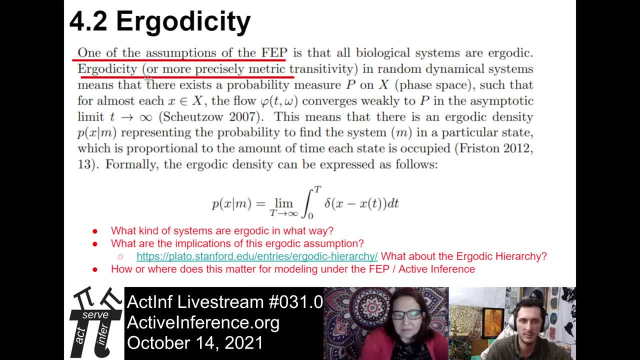 unpack and understand, like how? how does it mean ergodicity or, more precisely, metric transitivity in random dynamical systems, like what is the math and the physics? and is that an assumption of the fep? what does this mean? to assume that biological systems, quote- are ergodic, which is different than saying biological systems? 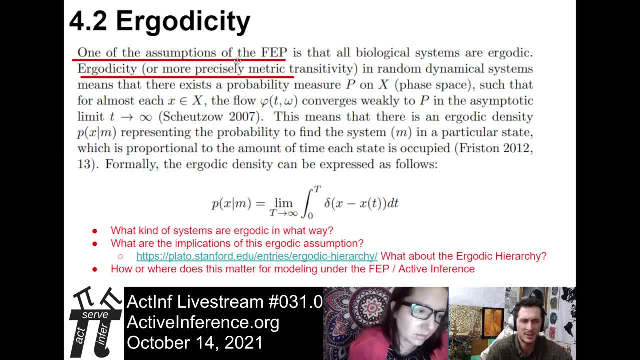 for some spatial temporal scales can be modeled using statistics that involve ergodic assumptions. so there's a lot of nuance there, like whether we're making relist claims about how biological systems are or whether we're using statistics in an instrumental fashion to make useful um models of organisms. but the big questions are like: 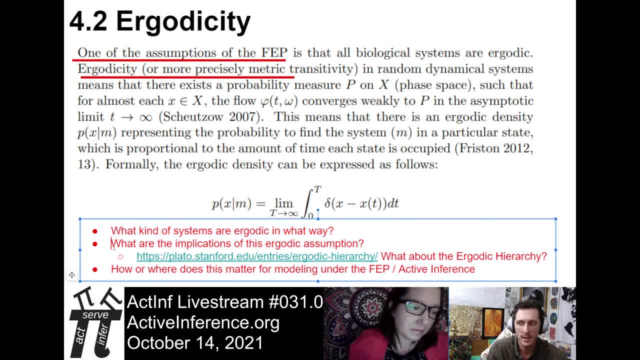 what kinds of systems are ergodic and how? what are the implications of ergodic assumption? is it ever not an assumption? but it's actually like a consequence of some empirical grounding. there's the ergodic hierarchy. so ergodicity it's not just like yes or no. there's a total continuum with a 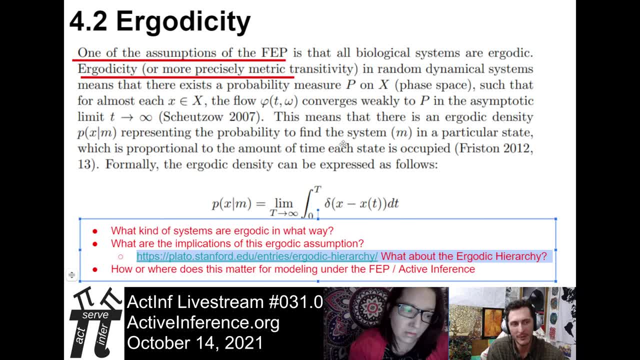 lot of complex math. and then, just for everyone, how or where does this matter for modeling under the fep or active inference in real world situations? and they did call out in the paper um a reference to ramstead and the local ergodicity which is, you know, for a biological organism. i'm like something like the you know boundaries, in which 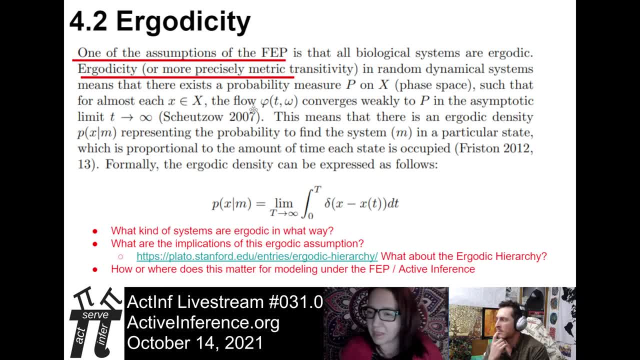 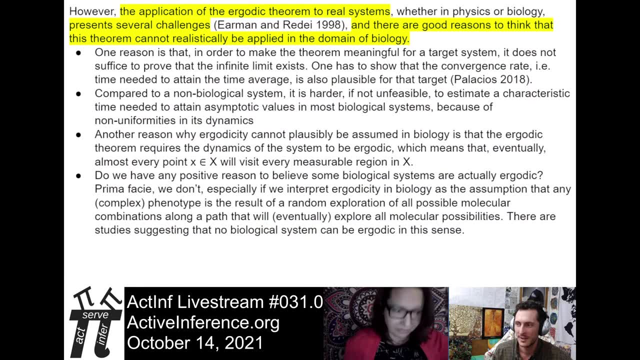 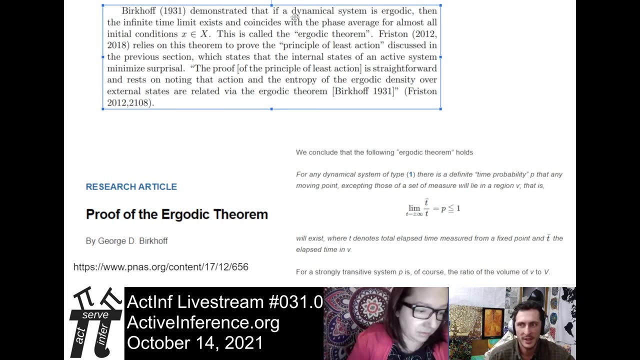 the organism can exist, um, anyway, i think. uh, maxwell, come come explain it to us please, but um, um, they, the authors, did mention that, so here's a quote from the paper. birkhoff 1931 demonstrated that if a dynamical system is ergodic, then the infinite time limit exists and coincides with 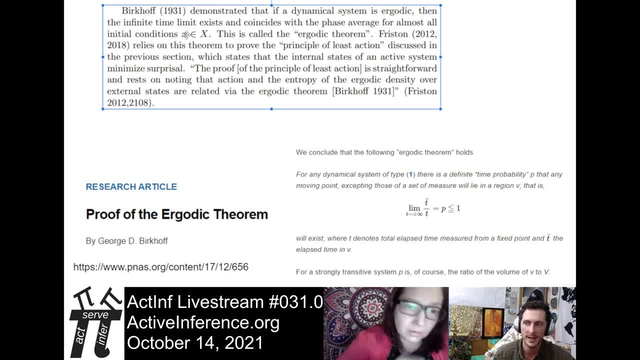 the phase average for almost all initial conditions: little x like the realized conditions within the bigger x like the space of the possible. this is called the ergodic theorem and that is going to get linked to everything we were just discussing. surprisal minimization as ergodicity. 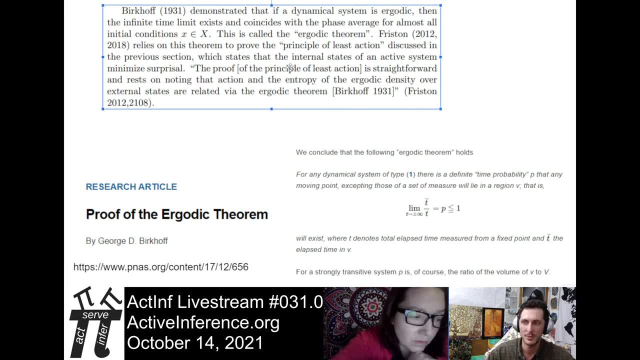 maintenance. and then here the proof of the principle of least action is straightforward, okay, and rests on noting that action and the entropy of the ergodic density over external states are related via the ergodic theorem, first in past and the future. so pnas birkhoff, 1931. 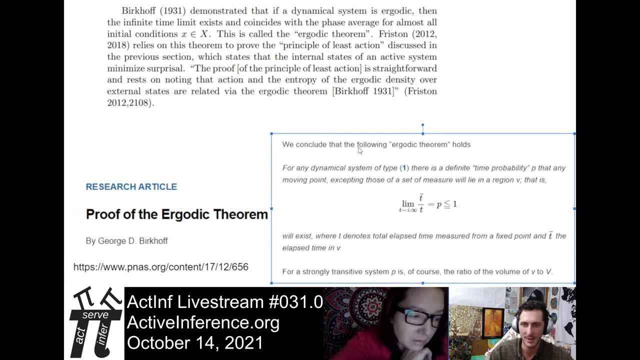 pretty interesting paper And just it's amazing to think like how much you know a hundred years of mathematics after this. but this is kind of that initial formalization of what if the space average and the time average were going to be related to each other. So it's a cool topic We've brought up. 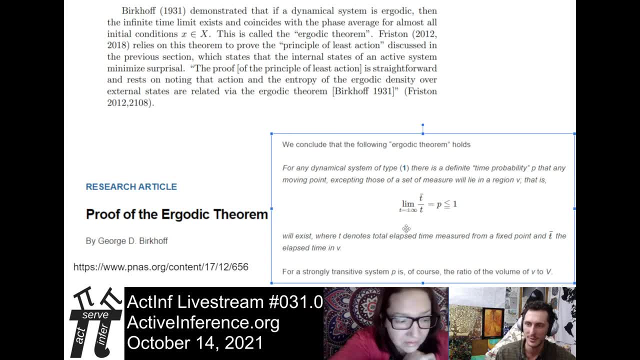 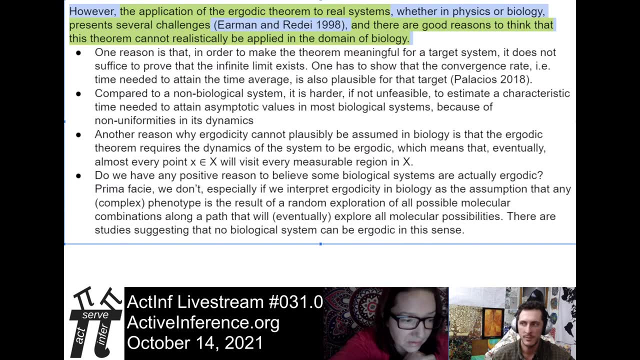 ergodicity before, and it would be really helpful for people who know some of the technical details to help work with it. This is one analogous to how they brought up like: here's the facts that challenge phase spaces in biology. So here's some facts that challenge the application of. 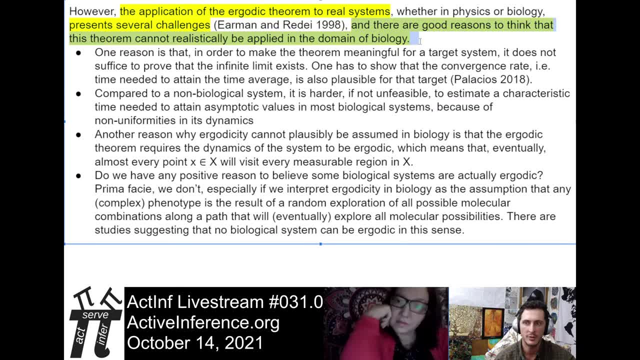 ergodic theorems to real systems, And there's good reasons, the authors say, to think that the theorem cannot be realistically applied in the domain of biology. So, first off, it's not enough to show that the infinite limit exists. It also has to be shown that the convergence rate is plausible. We're going to talk about that in a 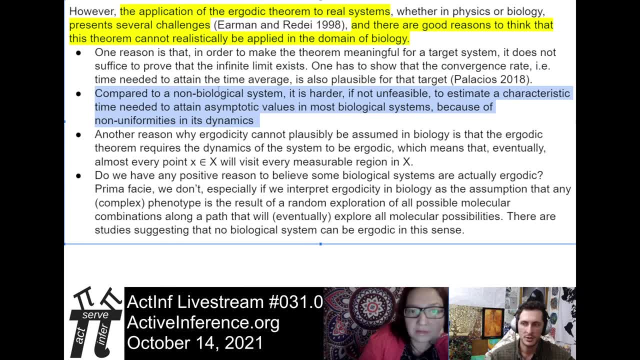 second. Second point: comparing biological to non-biological systems, it's harder to estimate the amount of time that they need to kind of asymptote because of the non-uniformities. Another reason, and this is going to be one that I know people will have things to say: 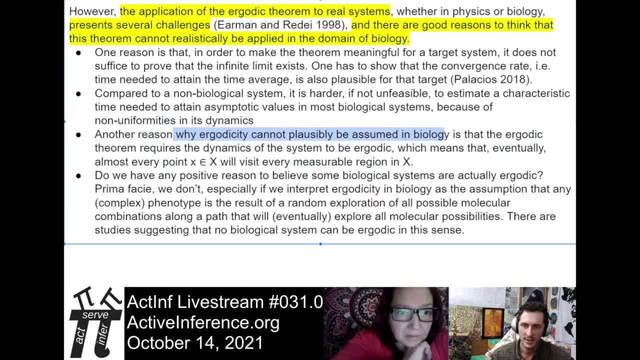 why ergodicity cannot plausibly be assumed in biology is that the ergodic theorem requires the dynamic of the system. So it's not enough to show that the convergence rate is plausible, It's not enough to show that the dynamics of the system to be ergodic, which means that eventually, 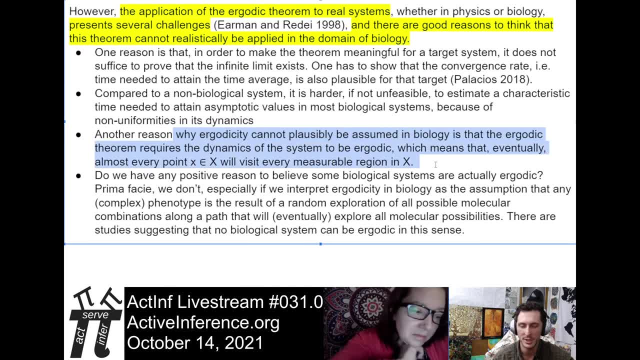 almost every point, will visit every measurable region in X. We've talked about that before like, but biological systems never revisit the exact same state if you think about every molecule constituting the phase space, But if the phase space is just temperature versus blood sugar, 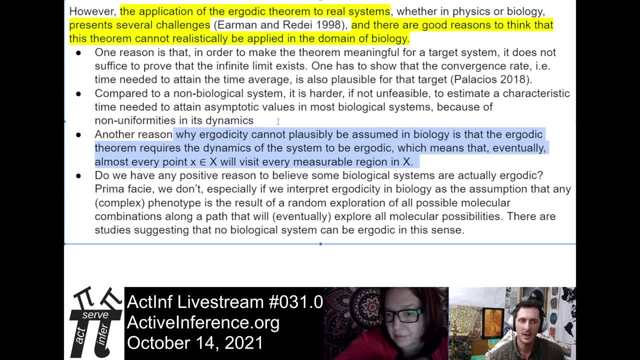 yes, you pretty much will revisit some points, but will you revisit every point? Are you going to reach a value of negative 5,000 sugar and 5,000 blood sugar? Are you going to reach a value of 900 degrees Celsius? No, we're talking about bounded states And that's kind of a nuance. 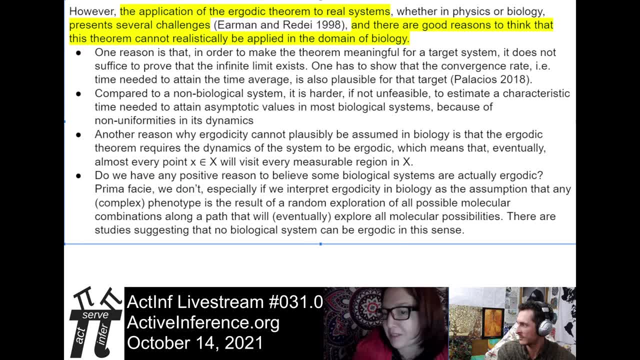 And then it's also. it's also the arrow of time, is is moving forward right, It points one direction And so, like you know, at at age 40, my skin will never have the collagen it had at age. 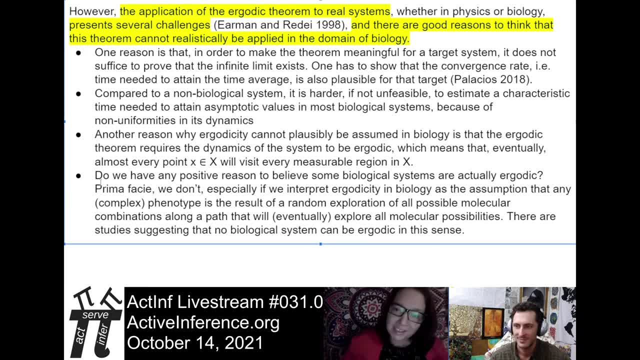 four, Like that's never going to happen again, Right? So I mean, and there are some things that just decrease as you age? Yes, So there are, yeah, Yeah. Let's look at this Palacios 2018 paper. So this is, I guess, an earlier paper by the first. 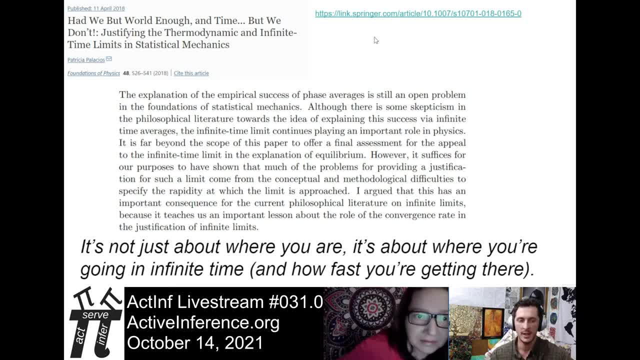 author. So it kind of gives a little context. Had we but world enough and time? but we don't. exclamation point: colon justifying the thermodynamic and infinite hyphen: time limits in statistical mechanics. Great title, Well punctuated. 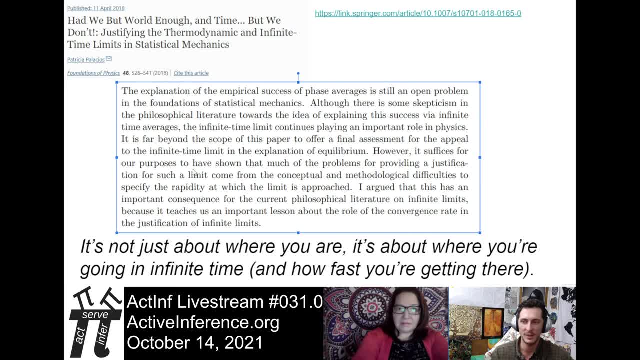 A bevy of punctuations And this is just a very interesting paper that we skimmed over And I'm sure there's a ton to say. it'd be great to speak with the author about it. but they argue that this has there's an important consequence for the philosophical literature on. 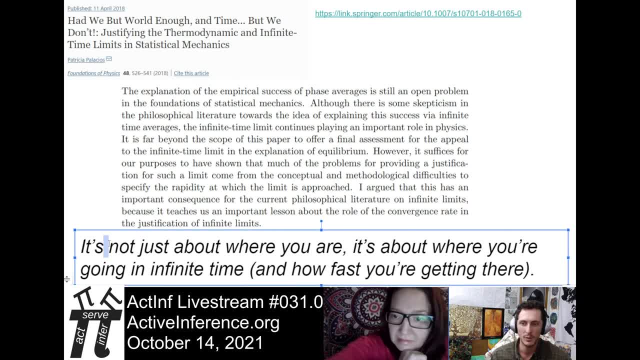 infinite limits And that's basically. it's not just about, like, where you are, that's where you are in phase space, It's about where you're going. That's the asymptote in infinite time, And it also matters how, how fast, you're going to get there. So it's like kind of the asymptote for a pane of glass. 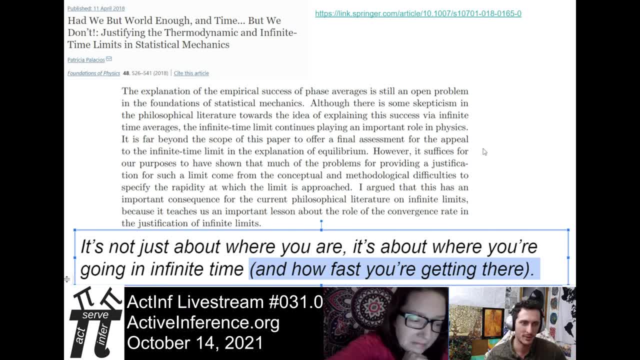 is like in a puddle on the ground because it's a liquid or it's a glass. but that might take so long that over some timescale it can be modeled as if it's not changing, for example. So that's kind of a cool notion that it's not just about where a system is or where it's being. 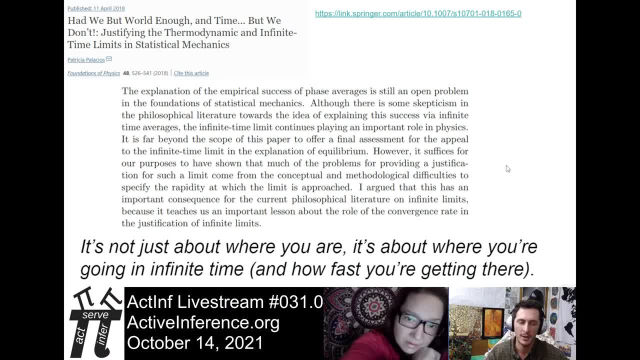 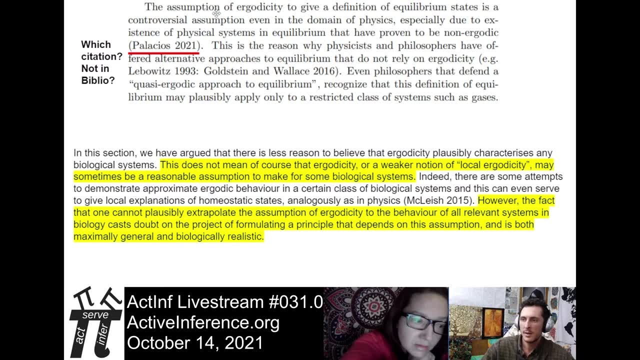 attracted towards. but actually the dynamics of the approach matter a lot, And that's certainly true in biological systems. The assumption of ergodicity to give a definition of equilibrium states is a controversial assumption even in the domain of physics, especially due to existence of physical systems. 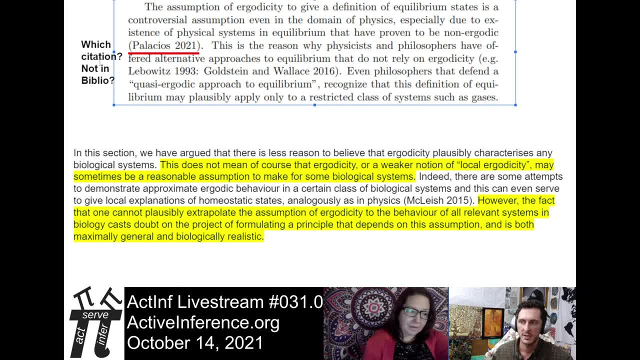 in equilibrium that have proven to be non-ergodic. So I didn't find this Palacios 21 citation in the Biblio. This is the reason why physicists and philosophers have offered alternative approaches to equilibrium that do not rely on ergodicity. This is the reason why physicists and philosophers have offered alternative approaches to equilibrium that do not rely on ergodicity. 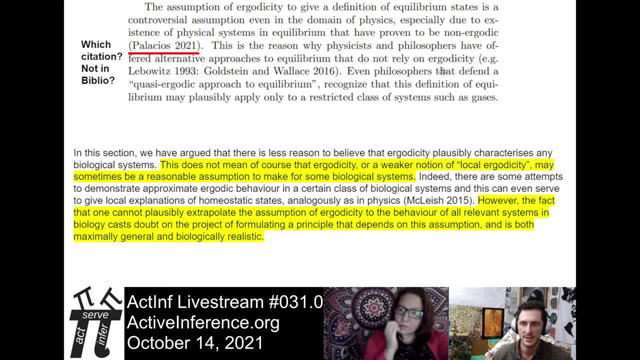 So I didn't find this Palacios 21 citation. in the domain of physics, even philosophers who defend a quasi-ergodic approach to equilibrium recognize that this definition of equilibrium may plausibly apply only to a restricted class of systems, such as gases. 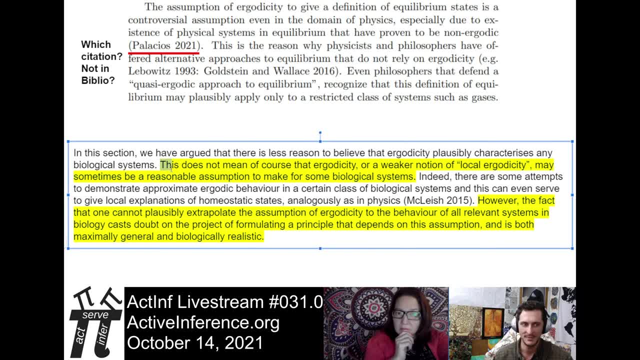 So sounds bad, but then we go. okay, the authors say it doesn't mean, of course, that ergodicity or a weaker notion of local ergodicity may sometimes be a reasonable assumption to make. So in other words, it might be useful for specifically defined systems anyway. 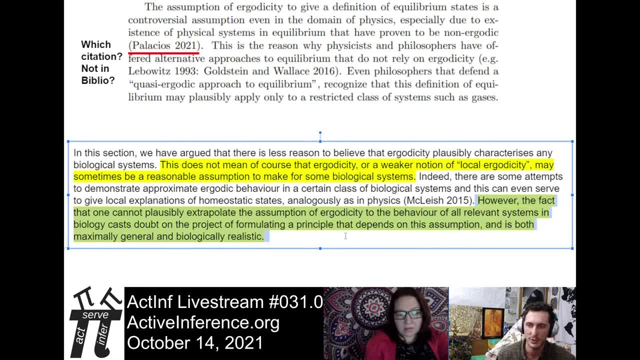 However, the fact that one cannot extrapolate the assumption of ergodicity to the behavior of all relevant systems in biology casts doubt on the project of formulating a principle that depends on this assumption and is both maximally general and biologically realistic. So ideas that we've heard a little bit about. but how are we going to finesse realism and generality and grounding in physics when biological systems might be grounded in things that are not fulfilled? 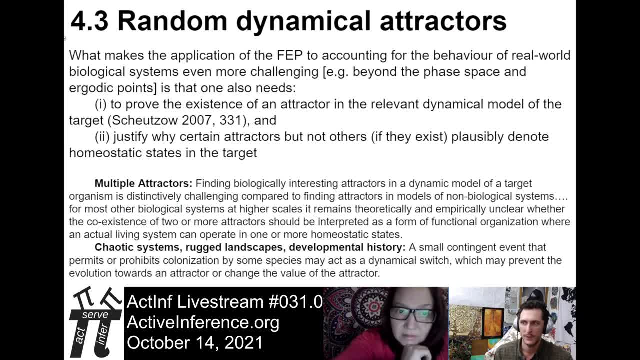 So that's 4.2.. All right, 4.3, random dynamical attractors. What makes the application of FEP to account for real-world behavior of biological systems is even more challenging. Beyond 4.2. And 4.1, because one also has to show the existence of an attractor and also justify why certain attractors but not others plausibly denote homeostatic states in the target. 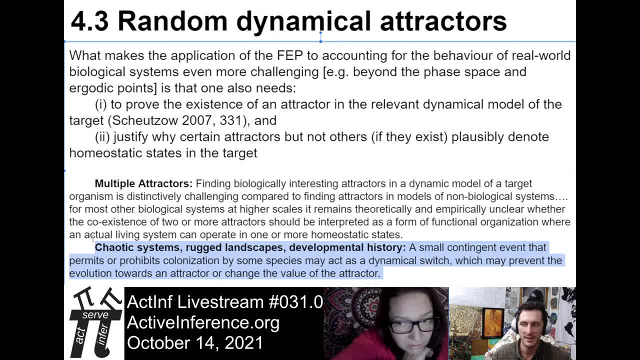 There might be multiple attractors. And then there's this question of chaotic systems. Do you want to add anything on these? Basically, it's non-trivial to say that there's an attractor and it's the right one, and it results in adaptive behavior. 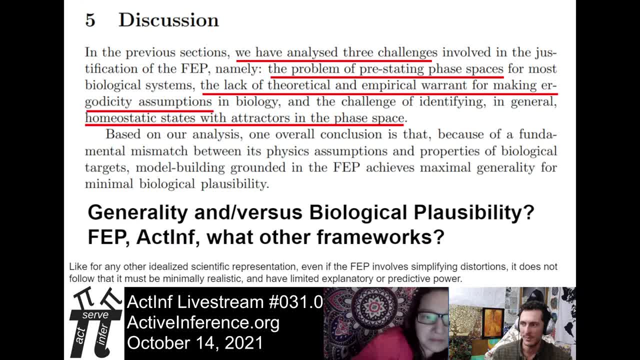 There's a lot that goes into it, So, but we can learn more. We'll hear more questions later. And then just to go quickly to 5 and 6.. So 5, discussion. In the previous sections we've analyzed three challenges involved in the justification of the free energy principle. 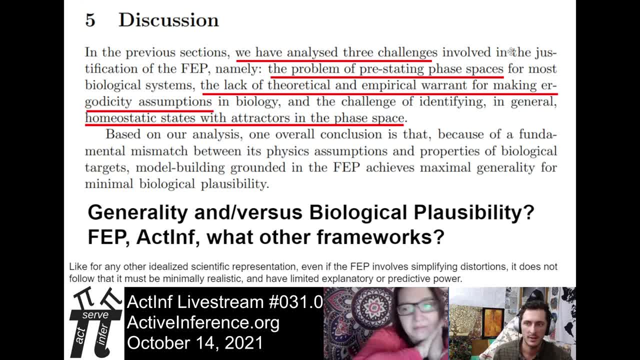 So one was pre-stated phase spaces for most biological systems. Two was the lack of the warrant for making ergodicity assumptions in biology. And three was the lack of the warrant for making ergodicity assumptions in biology. And three is the challenge of identifying homeostasis with attractors in a phase space. even if one and two were accomplished, 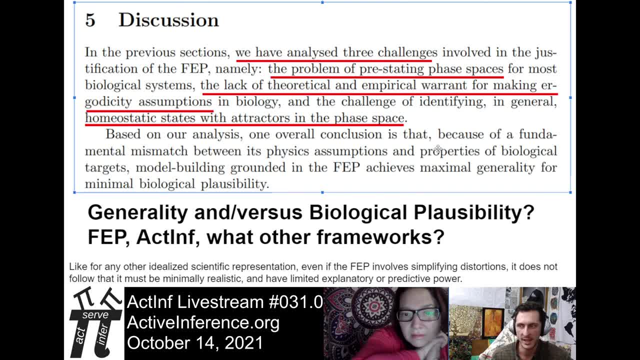 Based on our analysis, one overall conclusion is that, because of a fundamental mismatch between its physics assumptions and the properties of biological targets, model building grounded in the FEP achieves maximal generality. yay for minimal biological plausibility- Bad. So how do we do that? 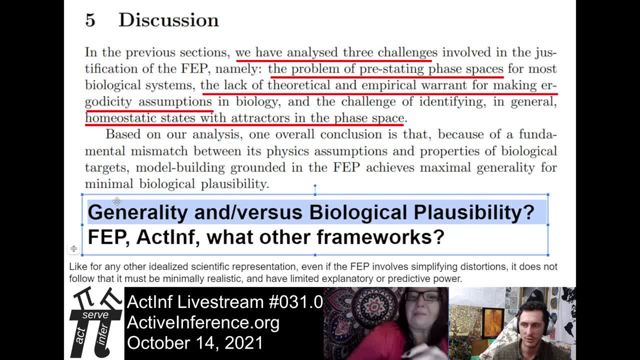 How is that going to work? As we raised earlier, how does generality versus plausibility get traded off for real systems In the FEP, in ACT-INF and in what other frameworks? Let's always have another one if people want to or can think of one, so that we're not just asking whether it's like as good as it could be. 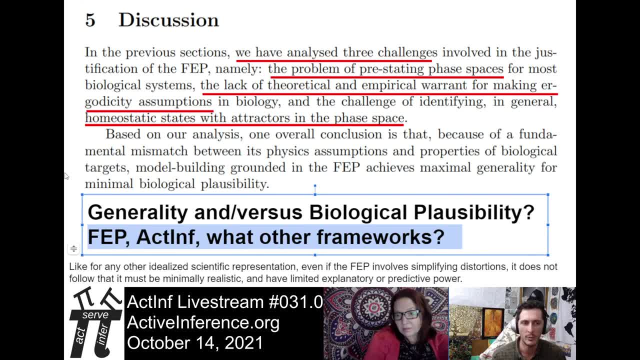 Because- here's a hint- It's not as good as it could be. We're always going to see ways to improve the theory and the literature, If only. If only by organizing other work and making it more accessible. So what is its relative biological plausibility? 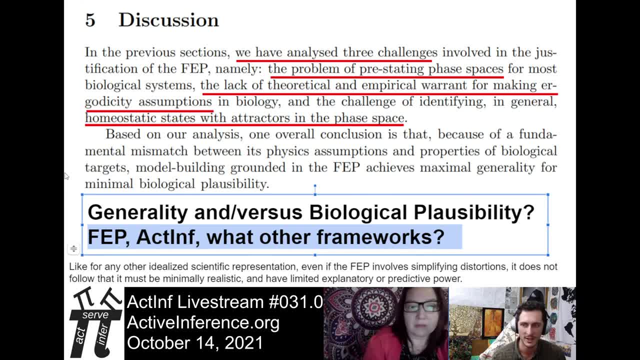 What is its relative generalizability And what are we relativizing to? Because, as they say, like for other idealized scientific representations, even if the FEP involves simplifying distortions, it does not follow that it must be minimally realistic and have limited explanatory or predictive power. 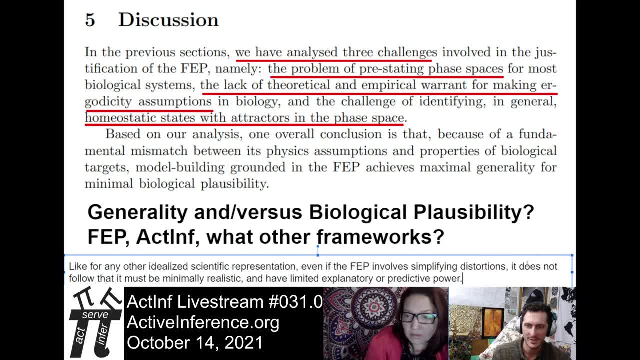 So they're saying it's kind of like: enemy of my enemy is my friend. It's like saying, just because you idealize and simplify, that it doesn't mean that you're going to get explanation or prediction. So that's their discussion. 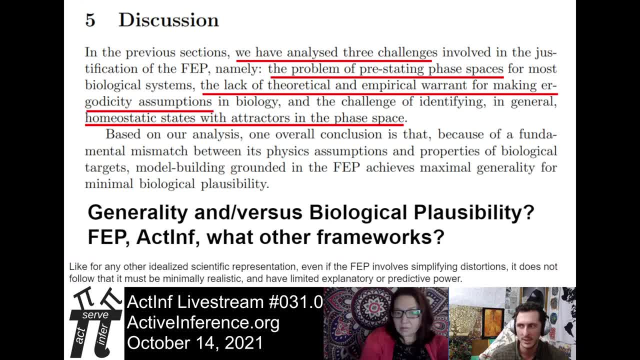 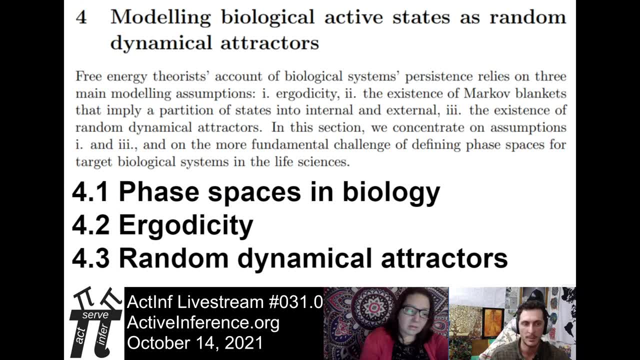 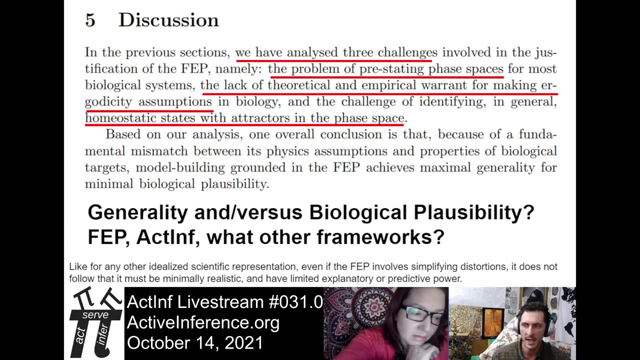 They fall back to the three key points that they think challenge the usage of physics ideas in biology that are postulated to be underlying the FEP phase- spaces, ergodicity and random attractors- And they're concluding that they're concluding that there's a mismatch between the physics assumptions and the properties of biological targets. 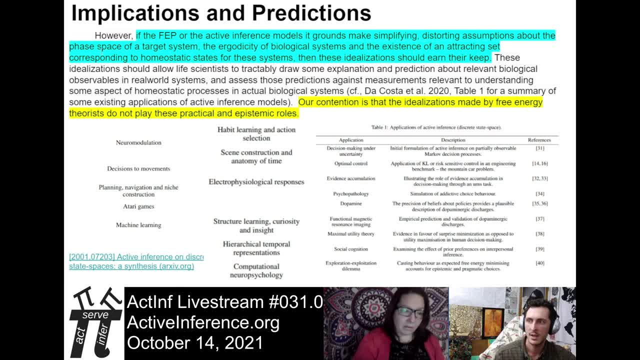 Here in the implications and predictions they write. if the FEP or active inference models it grounds make simplifying distortions, distorting assumptions about the phase space of a target system, the ergodicity of biological systems and the existence of an attracting set corresponding to homeostatic states for these systems, 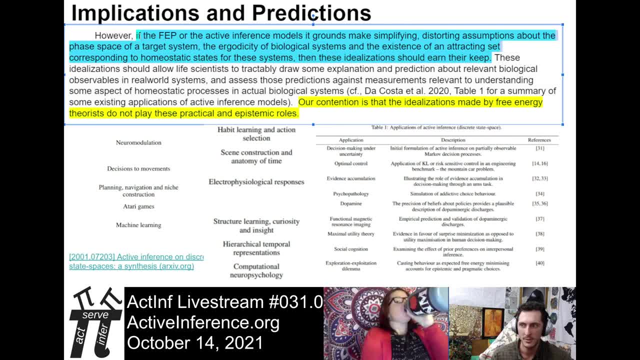 then these idealizations should earn their keep. We'll just read a little bit. These idealizations should allow life scientists to attractively draw some explanation and prediction about relevant biological observables in real world systems and assess those predictions against measurements relevant to understanding some aspect of 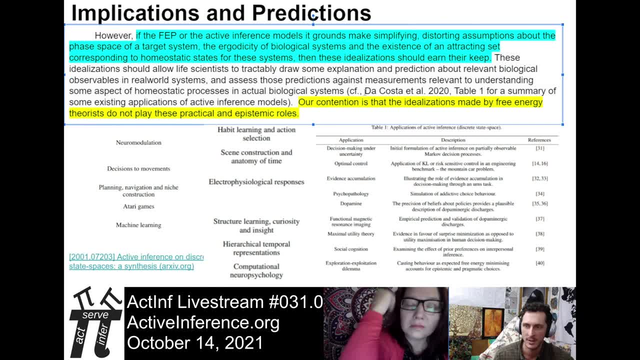 of homeostatic processes in actual biological systems- DaCosta et al 2020.. Our contention is that the idealizations made by free energy theorists do not play these practical and epistemic roles. So this is the DaCosta et al 2020, active inference on discrete state spaces- a synthesis. 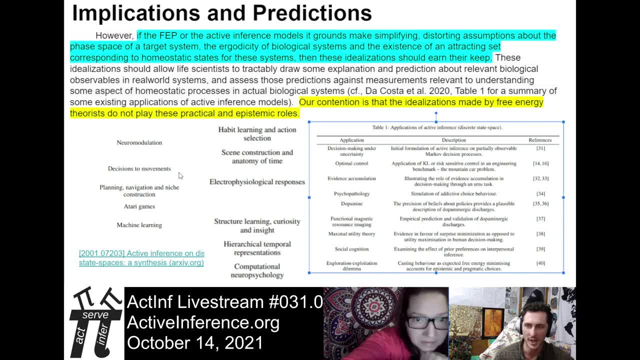 And here are from table one. here's all the applications. So it's interesting because, like this pragmatic and epistemic role, that's kind of the ontology of active inference, That's how we talk about policy selection, And then it's like, okay, looking at this list, I'm seeing a lot of pragmatic and epistemic. 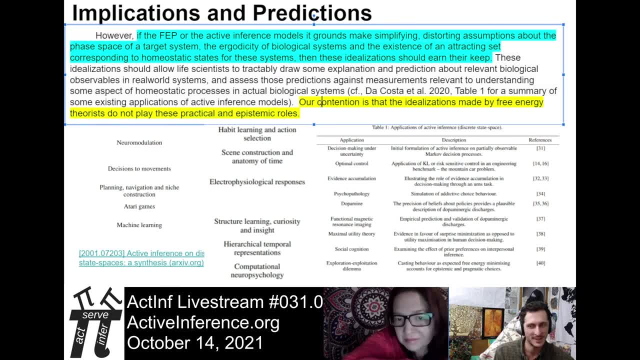 value. but what is the contention That the idealizations themselves do not play pragmatic or epistemically valuable roles? I think it'd be good To get a little clarification, because table one has a lot of, and since then even there's. 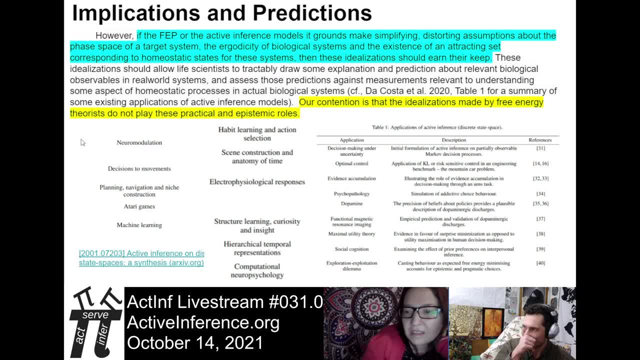 a lot of interesting areas. What do you think about that Blue? Yeah, it's interesting, Like the word choice of the author here, like the idealizations made by the free energy theorists. So what are these idealizations? Like the reliance on ergodicity and random dynamical systems theory. 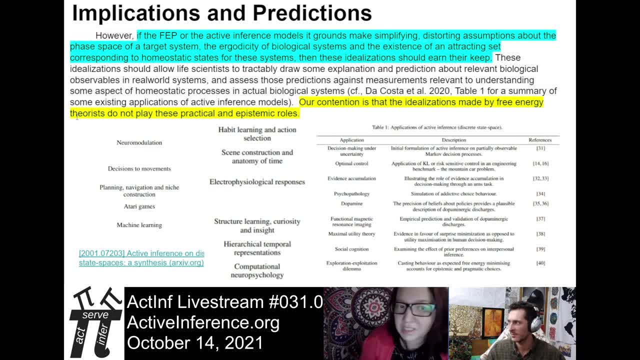 Like? are these idealizations? or is it actually using the FEP and active inference for practical applications that don't play the practical and epistemic roles? So I just am curious as to that word choice. And Steven in the chat wrote the use of approximation science around ergodicity could give the potential. 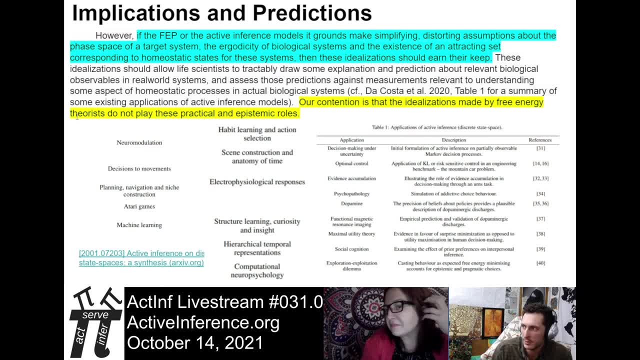 to have sufficient revisiting of states to make meaningfulness plausible? How can we measure when sufficient approximation to ergodicity exists in order to make variational free energy inferences? So good question we can ask And as we kind of explored revisiting, 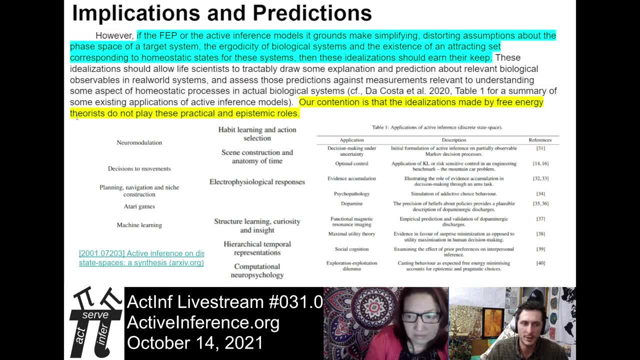 Revisitation is one component of ergodicity, but also there's this element of revisiting every point and of exploring the whole phase space. So, as we kind of addressed what is the reality of ergodicity and applying those models to biological systems, 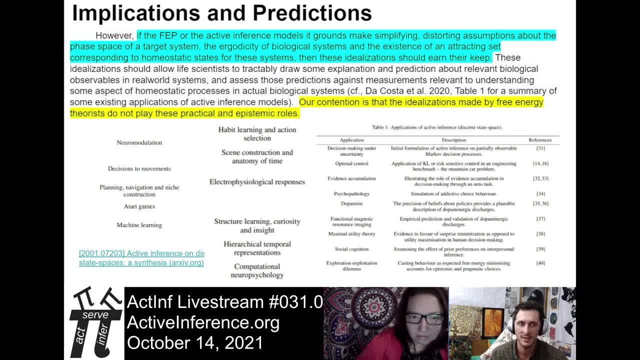 And then, yeah, can we use approximations and approximation science to make it work, Even if in the infinite perfect case it doesn't exactly seem like it would Like. the t-test assumes that there's an equal variance between the two groups, unless you. 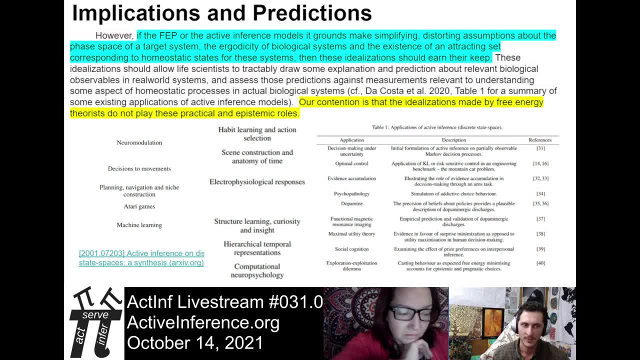 have a t-test with in-equal variances, yet no two groups in reality are going to have the exact same variance, yet the t-test works. So how can we take that same approach and think about the systems that we're working with here? 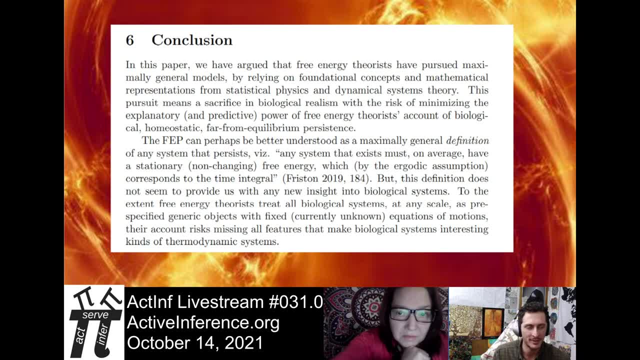 Here's their whole conclusion. in a churning maelstrom, They're arguing that FEP theorists have pursued maximal generalization By relying on physics concepts. however, that means that they've sacrificed biological realism, and the danger of sacrificing biological realism is that you risk minimizing explanatory. 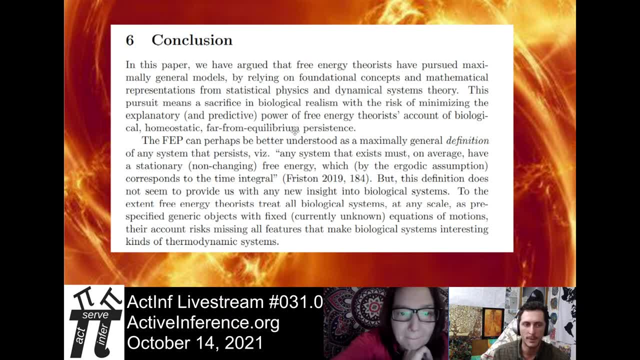 and predictive power of those accounts for biological systems which are homeostatic and manifestingly far from equilibrium in their persistence And their last paragraph, the FEP, can perhaps be better understood as a maximal generalization. It's a maximally general definition of any system that persists. 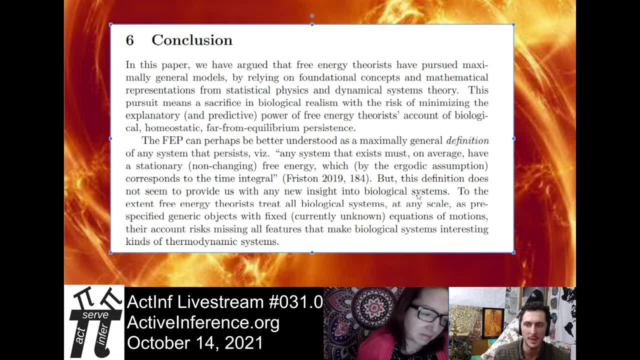 But this definition does not seem to provide us with any new insight into biological systems. To the extent free energy theorists treat all biological systems, at any scale, as pre-specified generic objects with fixed, currently unknown equations of motion, their account risks missing all features that make biological systems interesting: kinds of thermodynamic. 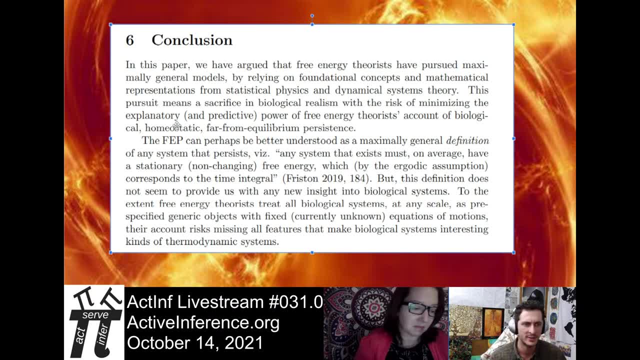 systems. So it's like you know a system that's fixed. It's like a city where there's all kinds of intersections and then you have a grid map, And so we distort the system in a way where all of a sudden we thought we were generalizing. 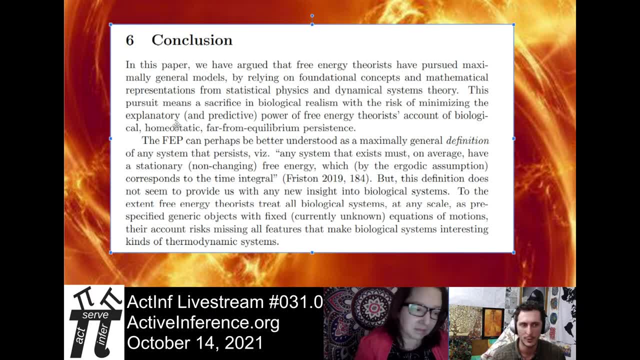 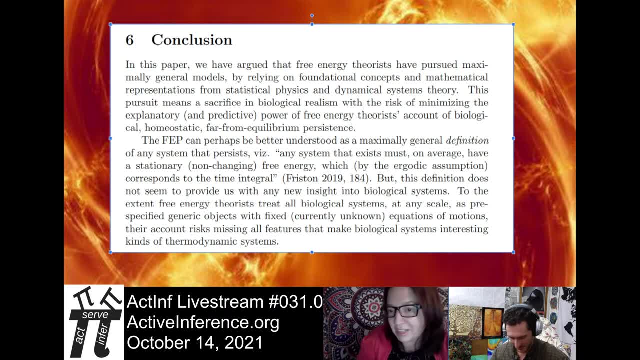 I think the FEP also has a lot to say about it, And the FEP also has a lot of room to grow, being that it's, you know, relatively not quite 20 yet. So I think that you know, hopefully, that some pragmatic and epistemic value will be. 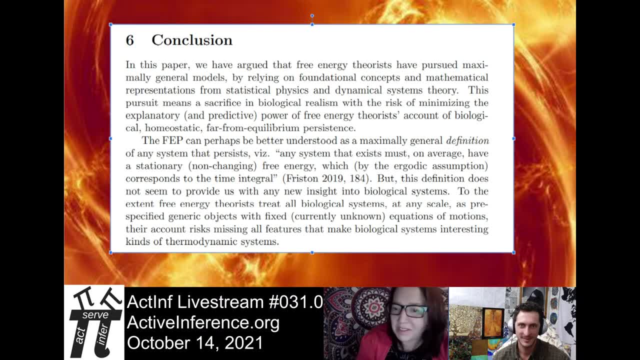 put forth by the generalizations made by the FEP in some future model. perhaps That's almost like a deep time sociological value, even a provocative theory which has limited epistemic or pragmatic value. not saying the FEP is could play a role in a broader social system that still gets the job. 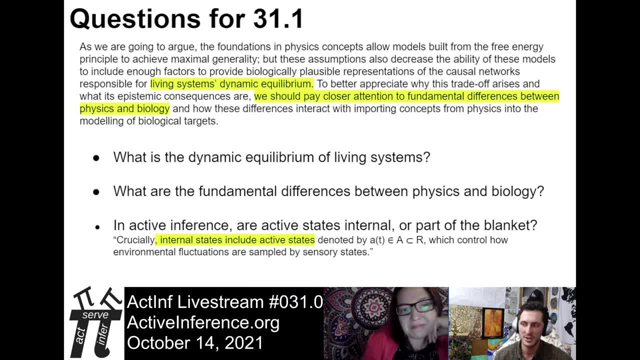 done. So that's kind of a cool notion. What questions for 31.1 did you put up? So I think I raised them all already. So, like, what is the dynamic equilibrium of living systems, as the authors state here and as I stated in the beginning, keywords, and it says we should pay. 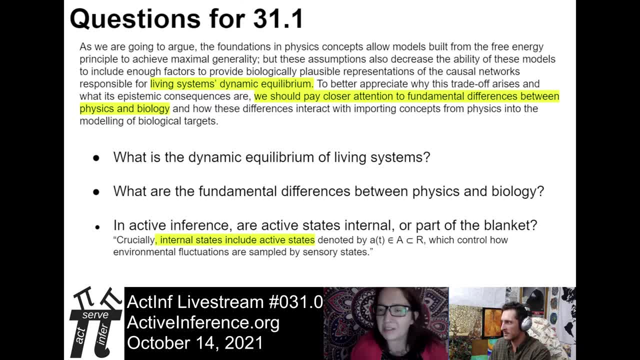 closer attention to the fundamental differences between physics and biology. Like, what are the differences between physics and biology? Like in the paper they made, they went to a great length to explain, like why biological systems weren't ergodic, but then also, like they made the point, 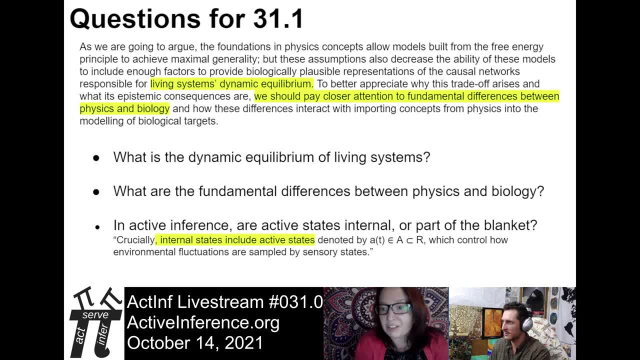 that physics they have a really hard time like proving ergodicity exists at all in any physical system. So what are these fundamental differences between physics and biology that are so critical like that? It seems that you know the FEP kind of misses the point And then they refer often in the paper. 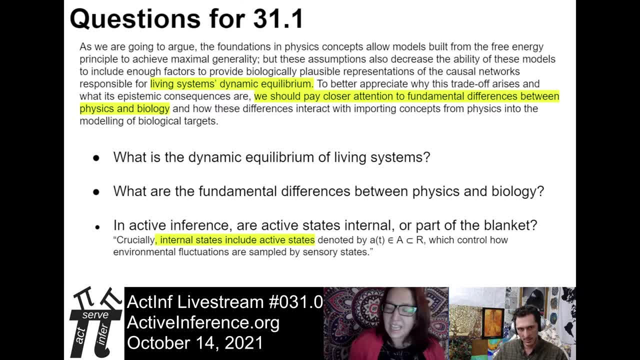 to active states as internal states And I just wonder what, like? I mean, I've really thought about active states as, like, the interface between internal and external and part of the blanket, And so I just wonder why the active states are included in internal states and their you know. 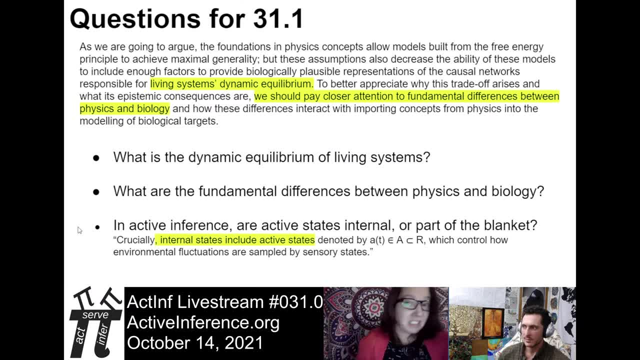 description of the model. So so just some, some tenets. I just wanted to, you know, share just some technical things that I have questions about and, you know, hopefully the authors will be here to answer them. Cool, Stephen wrote: we may never know the whole phase space, as the phase space may be variable. 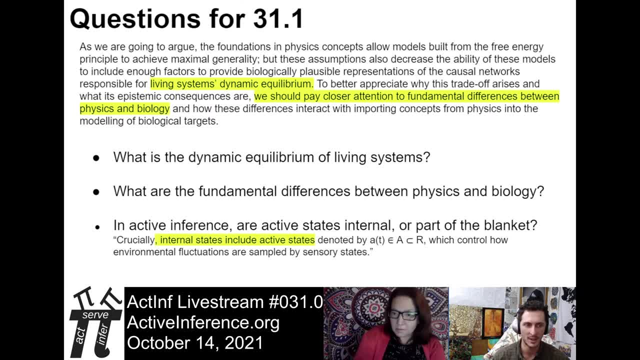 Yes, that's what we talked about. like the phase space of temperature, does that include impossible temperatures that the system cannot persist at? And then the fact that the phase space can change is the open-endedness of the- the Longo, I think- 2012- open-endedness of the phase space in biological systems. 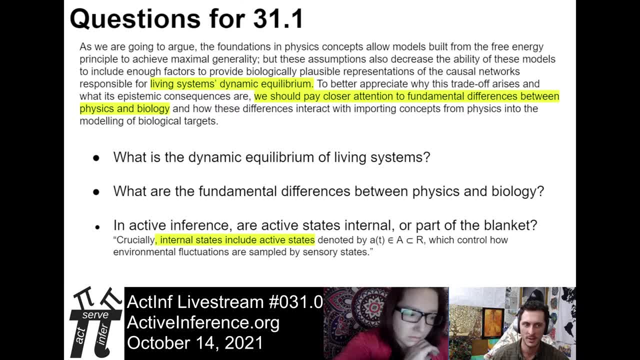 So for sure, that's why we can read the papes and then have specific citations and ontologies in mind. so we're not kind of cross-angling, because those are great points and they were the points made in the paper. and then steven asks: is biological realism based upon folk biological assumptions? so i think 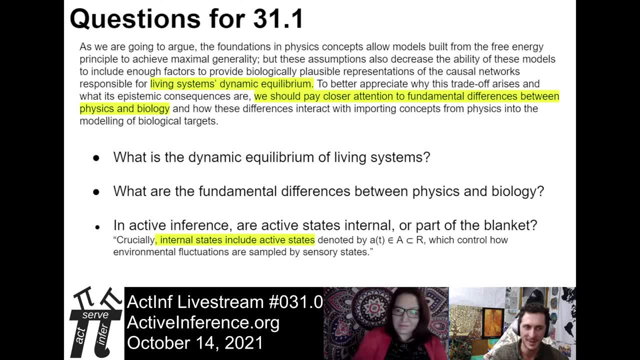 this sort of like folk hyphenated. everything has come into the forefront with the discussion with matt sims. so, yeah, what is biologically real? you know what models are biologically realistic? isn't that just like the question of what is real? so, yeah, what is even real at all? exactly, yeah, realism.